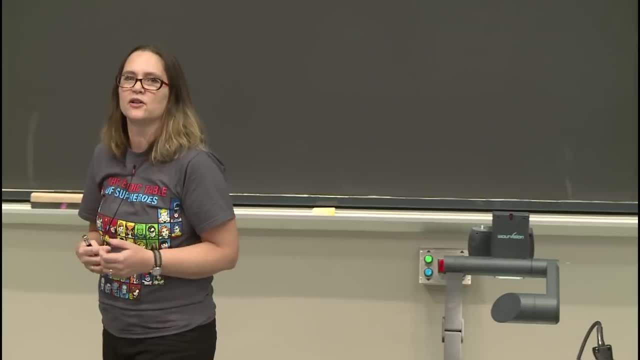 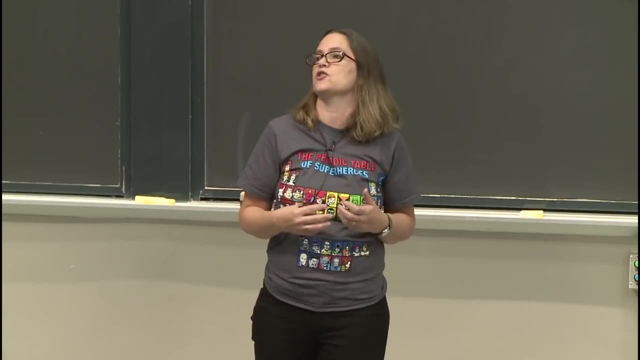 these incredible colors And they can put the transition metals in something with a magnet and see that they have magnetic properties. So these things were obvious. And then chemists want to try to understand why it's true, why this particular metal behaves this way or this metal has this particular color. 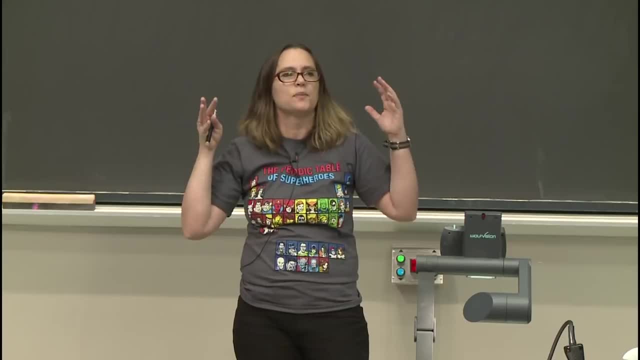 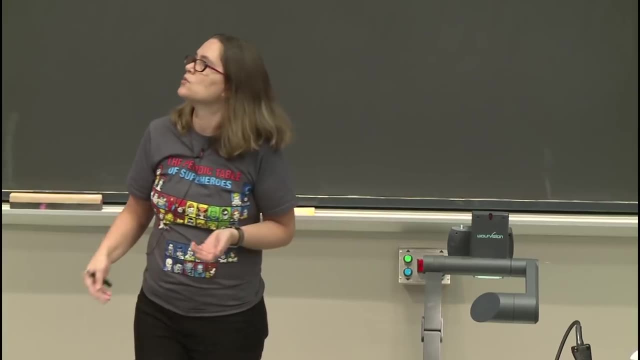 And they like to try to categorize them and come up with theories that help to explain what they're observing in nature, And so today we're going to talk about one of those theories, which is ligand field theory, And I'm also going to differentiate. 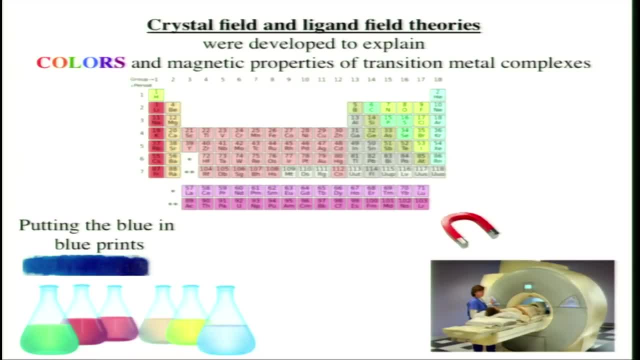 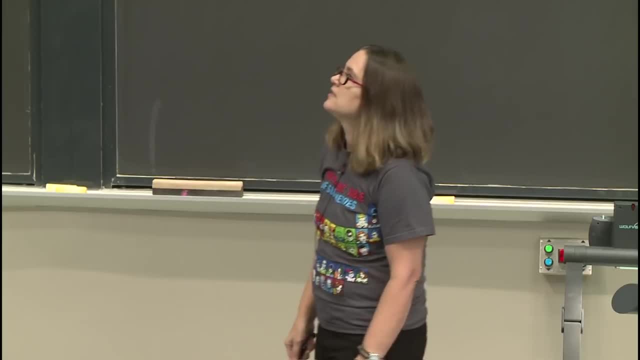 that crystal field theory and differentiate it from ligand field theory. So both of these theories again are an attempt to explain the properties that we observe, And the idea behind it is pretty simple. You have a metal ion and a set of ligands around it. 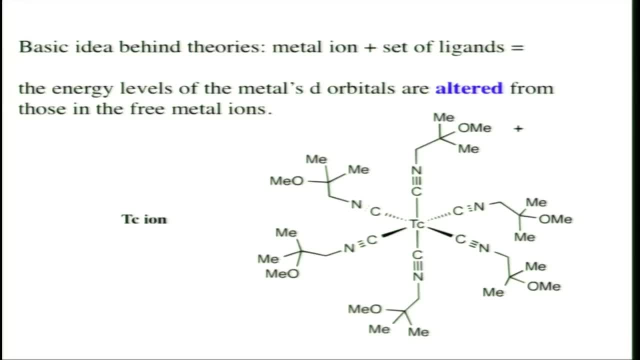 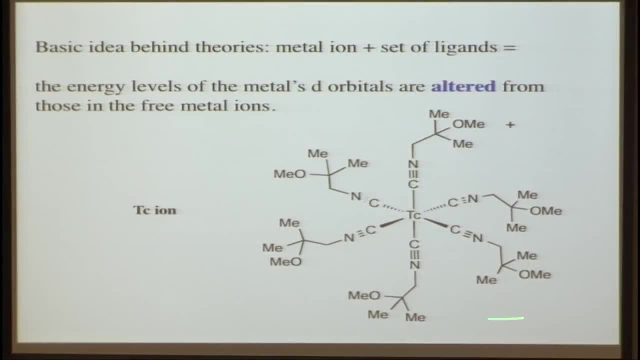 And if you compare the energy levels of that free metal ion, so here's a free metal ion with that metal ion in a coordination complex. here's a quite a pretty coordination complex. the energy levels are different. That's really all these theories are getting at. 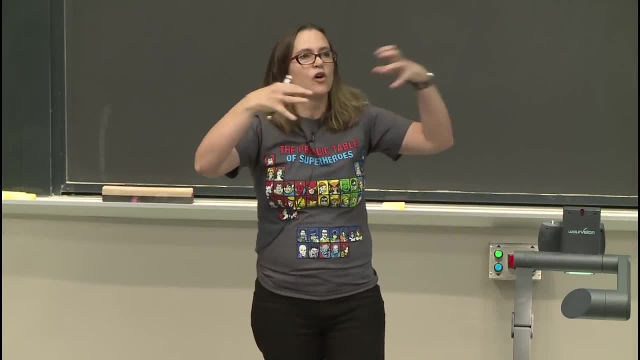 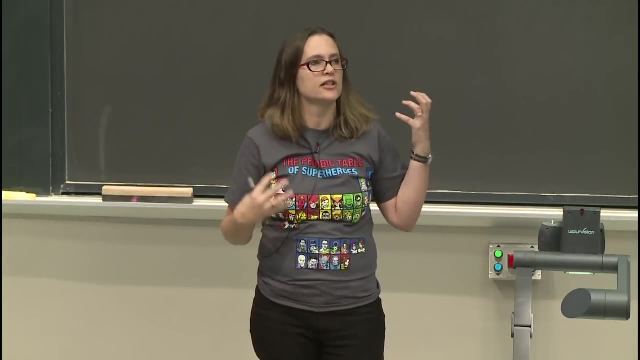 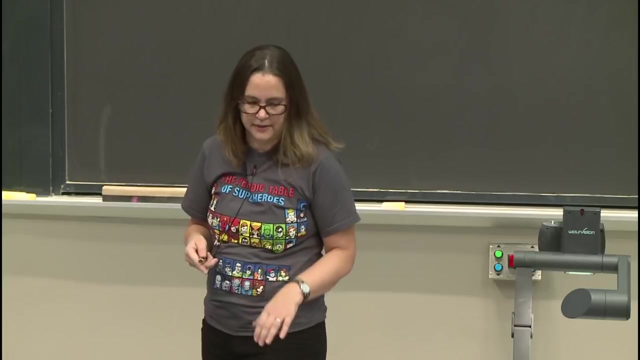 that there's a change when you bring the ligands in around a transition metal. It changes the energy levels of those d orbitals And if we understand how those d energy levels change, we can understand a lot about the properties of that particular metal in that coordination environment. 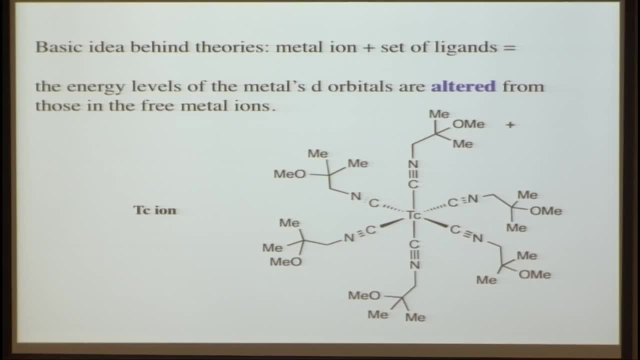 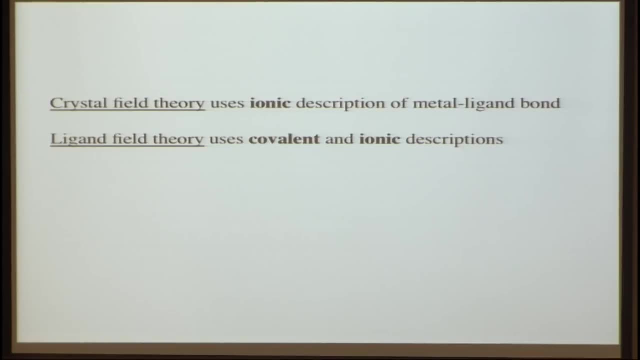 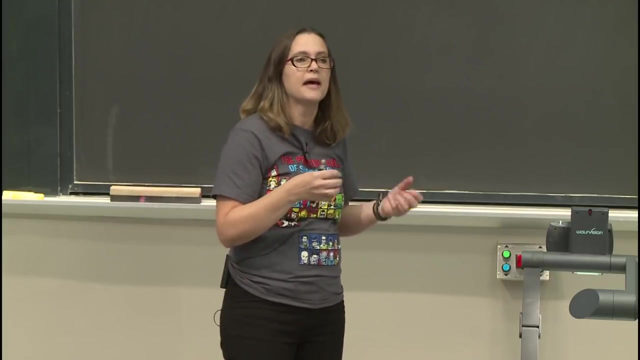 So energy levels are altered. So there's these two theories: Crystal field theory and ligand field theory. Crystal field theory is the more simple one. It just considers the ionic description of the metal ligand bond, And so we talked about ionic bonds. 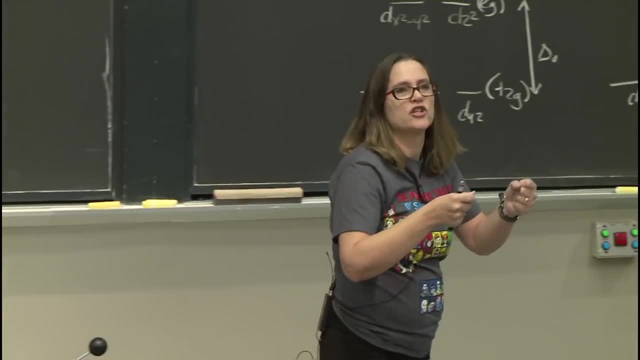 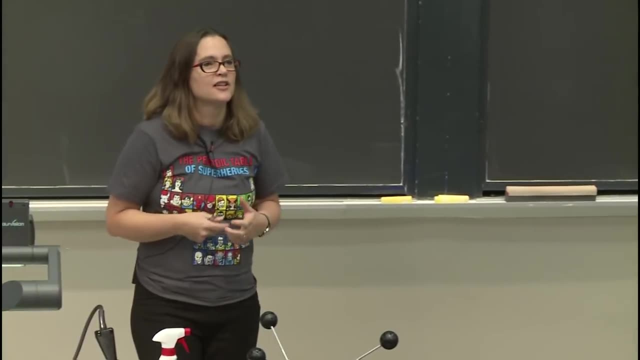 And mostly you're just kind of thinking about them as these point charges And you have plus and you have minus and they attract each other. Covalent bonding is a bit more complicated. Start talking about hybridization and other things like that. 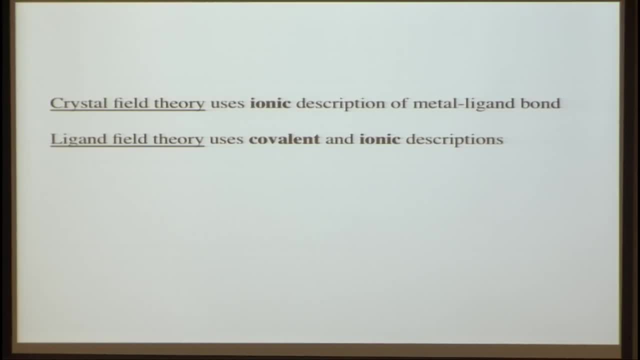 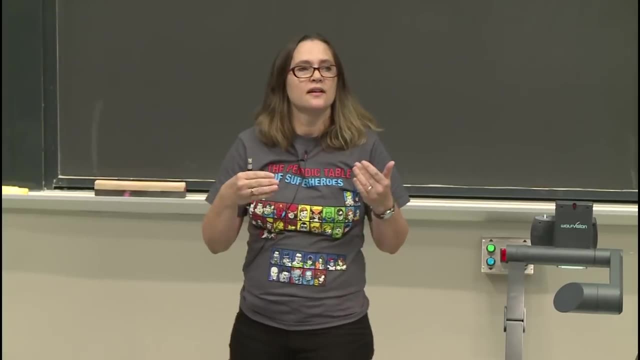 OK, So crystal field theory is really simple. It just considers the ionic nature And it does pretty well. It can explain a lot, but not everything. Ligand field theory has the covalent and the ionic, So it's a more complete description. 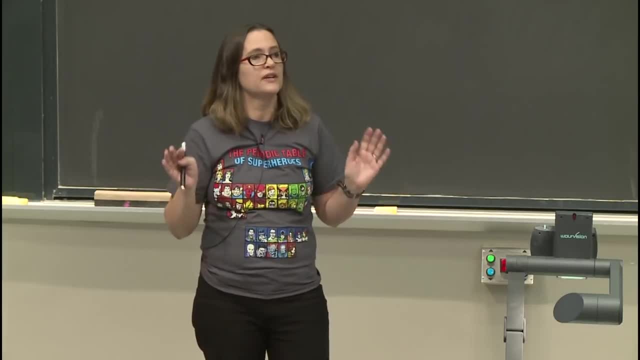 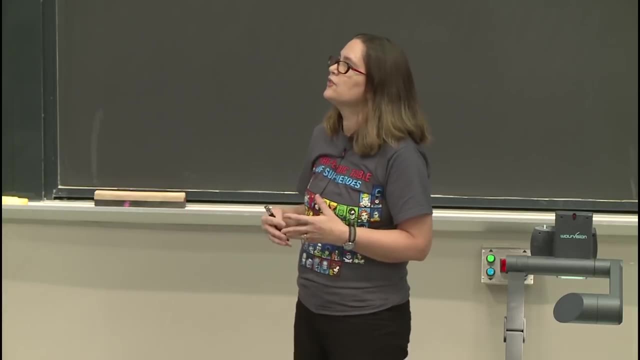 of that metal ligand bond, But this is more of an advanced topic. I just want to know that that exists. So if you take 503 here in organic chemistry, you'll talk more about ligand field theory. In this class we're just going to do crystal field theory. 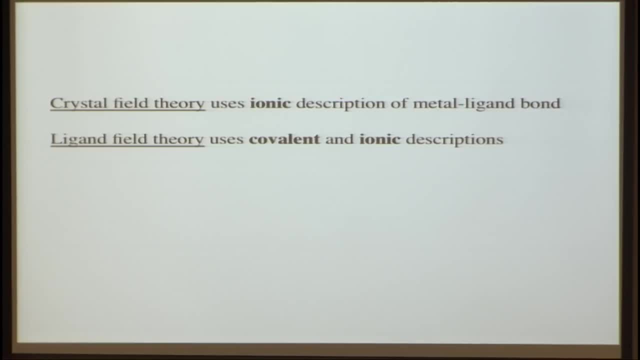 But I like crystal field theory because I like it when something that's pretty simple theory can explain a lot. I think a lot of nature can be explained by this. So if you really want to understand particular properties of a specific compound, you probably want a more complicated way. 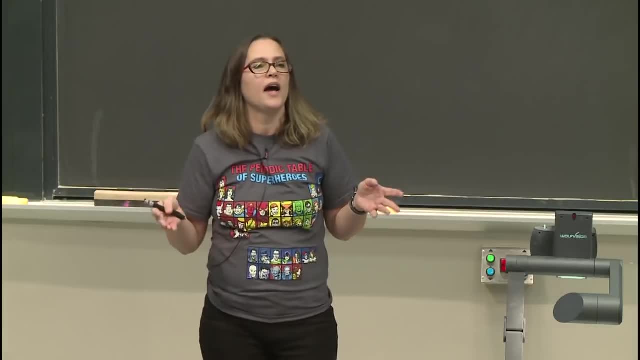 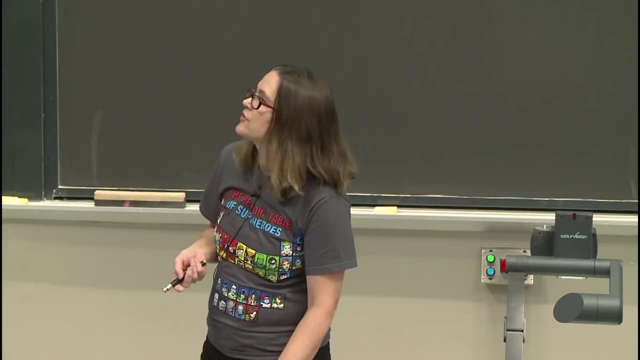 to think about it. But if in general, you just want to say why are some cobalt complexes can be so many colors, Crystal field theory works really well for that. All right. So crystal field theory, very simple idea behind it. 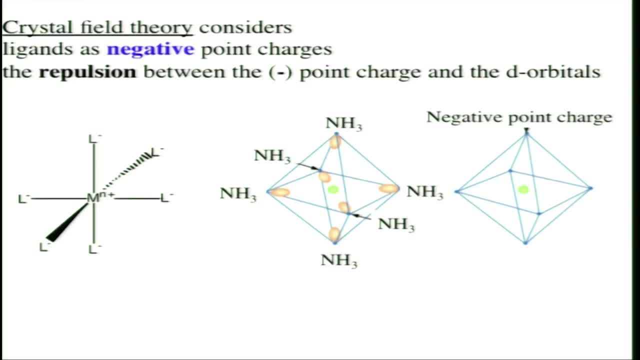 It's almost disappointing, I think, But it's OK, because you can go up here and say: yeah, we're studying crystal field theory in class. Yeah, You don't have to tell people that, it's a really very simple idea. 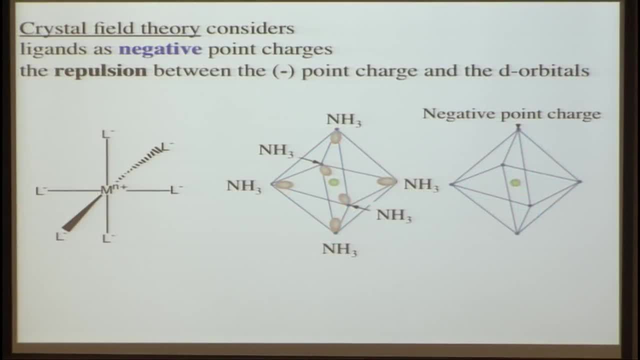 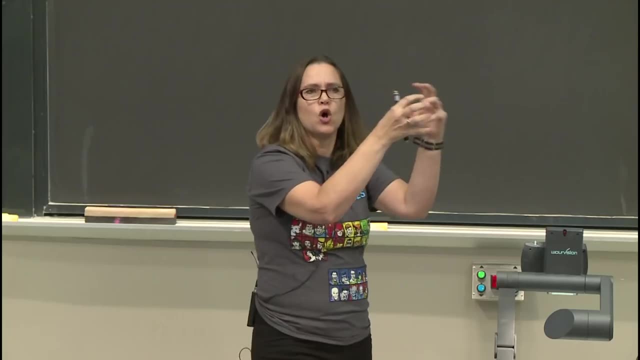 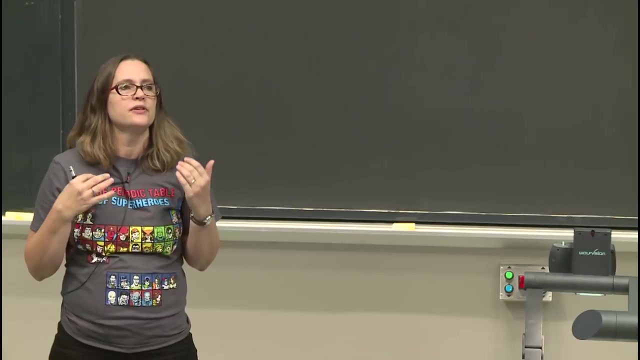 So the idea is that the ligands are negative point charges. They're like this big blob of negativity And those ligands with their lone pairs, their negative charge, they've got those extra lone pair. electrons are going to be repulsive to those d orbitals. 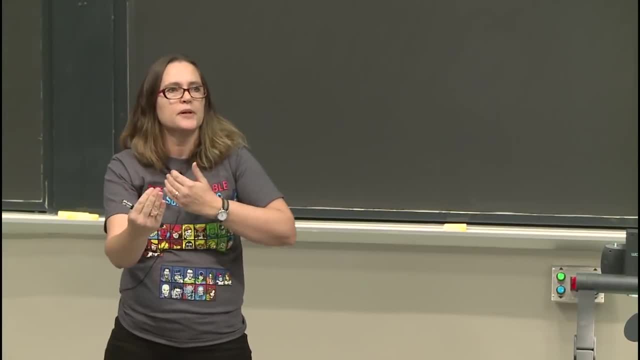 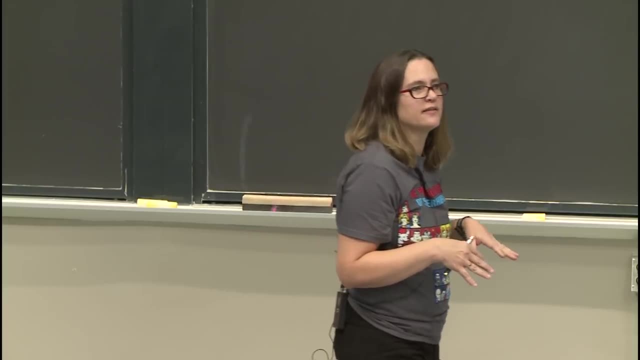 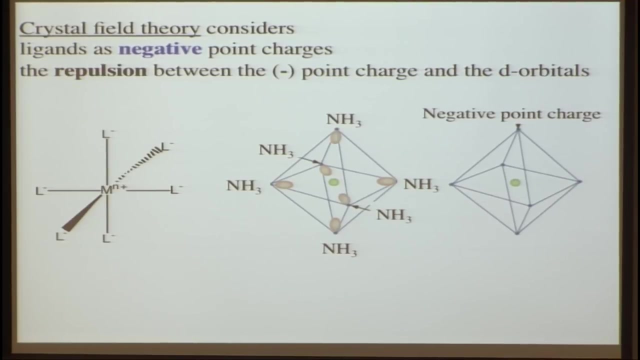 Negative point charges. you bring a d orbital and a lone pair and there's some repulsion. That's basically it: Negative point charge, repulsion- That's all that you have to think about with crystal field theory. So it sounds really impressive to tell people. 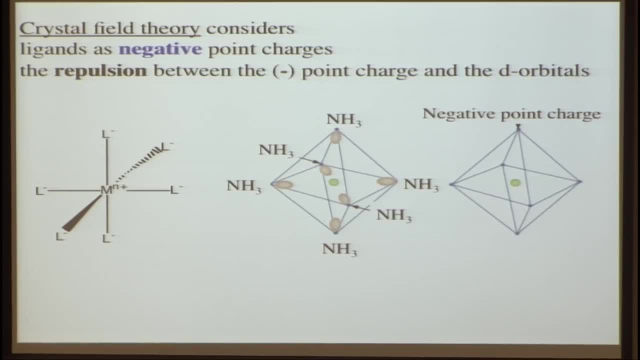 you're doing crystal field theory and you can neglect to mention that. it's just a really very, very simple idea: that sort of negative charges repel each other. That's really all. it is All right. So we're going to talk first about the octahedral case. 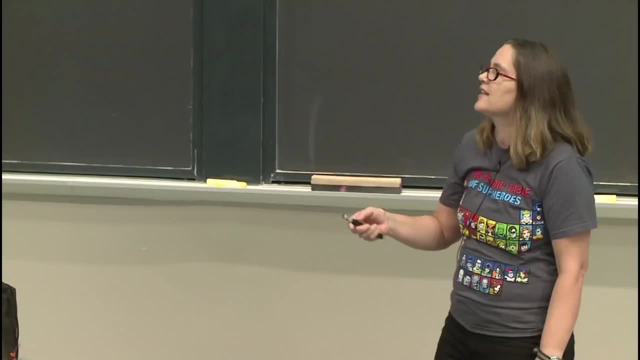 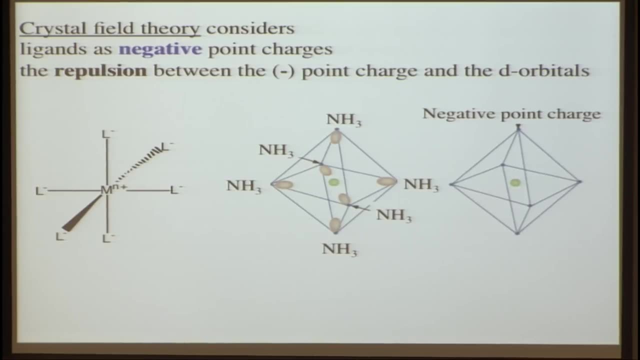 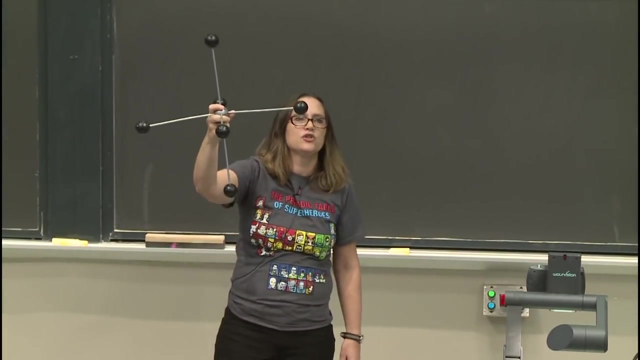 And then we're going to get into some other geometries on Friday, So that's going to be exciting. But here's our octahedral molecule, And here we have it here, And I can think about the metal in the middle, m to the n plus. 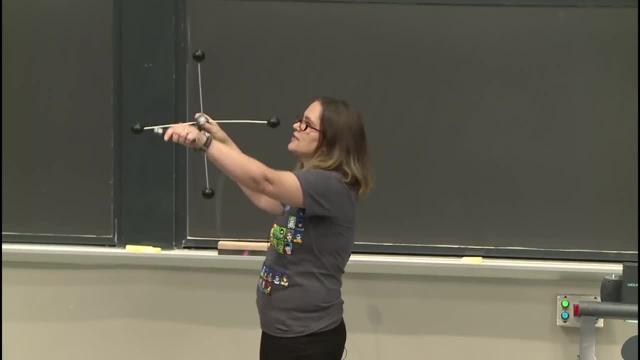 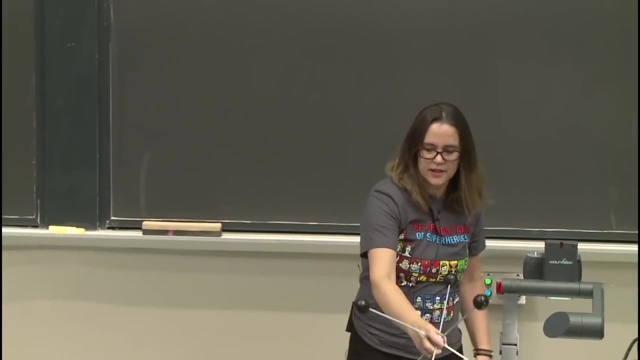 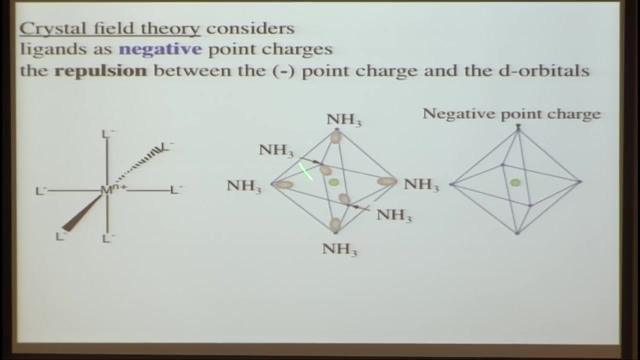 So this just indicates that's any metal and to the oxidation number And the black balls. here are the ligands And we can think of those as negative point charges. So here we have drawn sort of this octahedral shape around the metal in the middle. 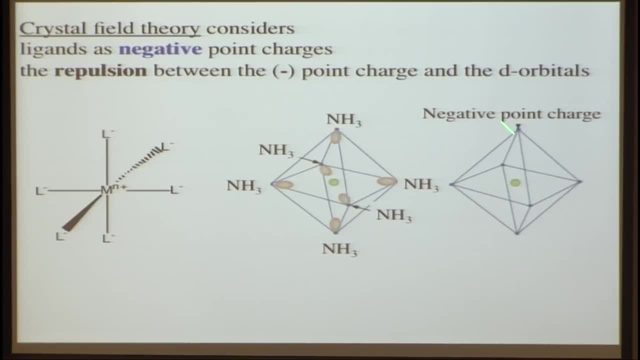 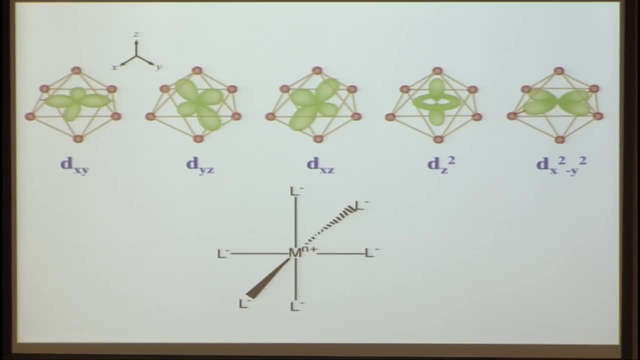 And we can think about these NH3 groups as these negative point charges. So these dots here are negative point charges. And so now, if we think about the shapes of the d orbitals again that we just looked at, we can look over here and say 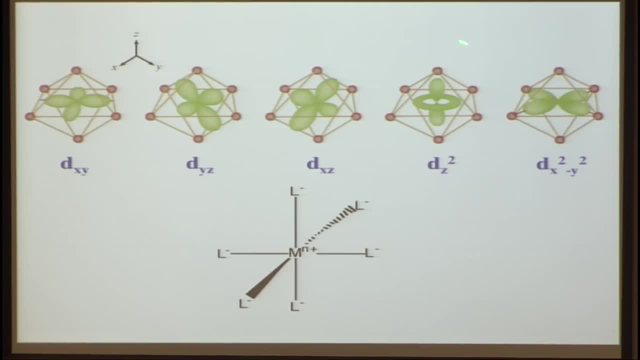 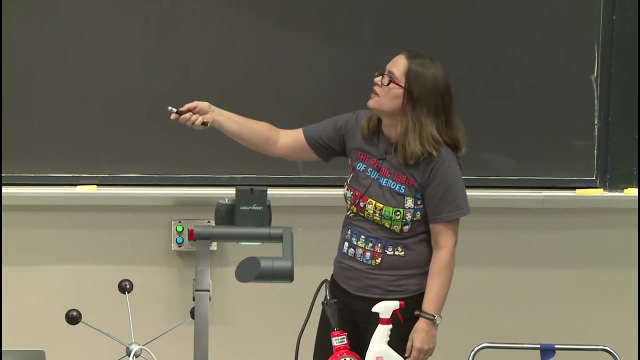 wow, some of those ligands that are, those negative point charges, Are basically right there up against that d orbital, pointing directly toward the d orbital. So that's going to be pretty repulsive if the point charge is right there next to the d orbital. 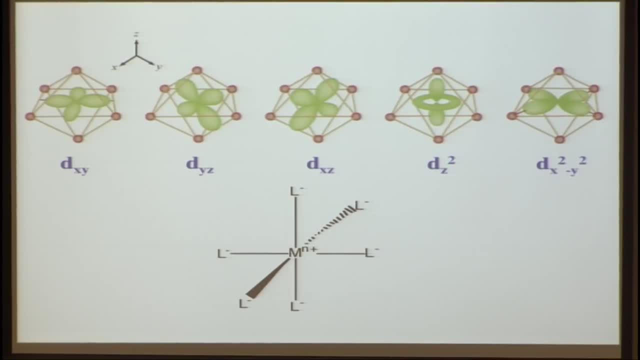 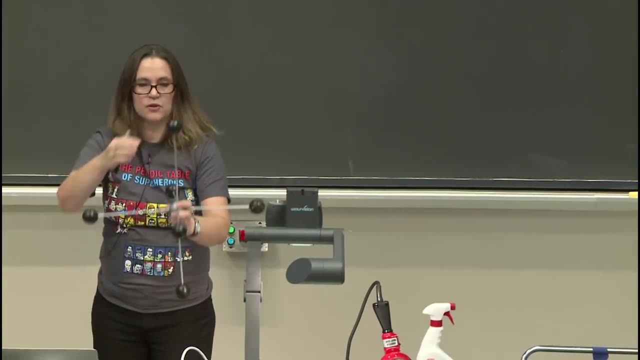 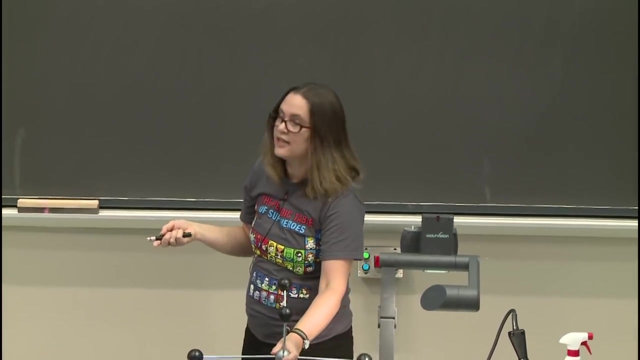 This also has a point charge kind of right toward it, along z. But these the point charges are on axis because, octahedral, you have your ligands along z, along x and along y, But these sets of orbitals, The negative point charges, aren't pointing directly. 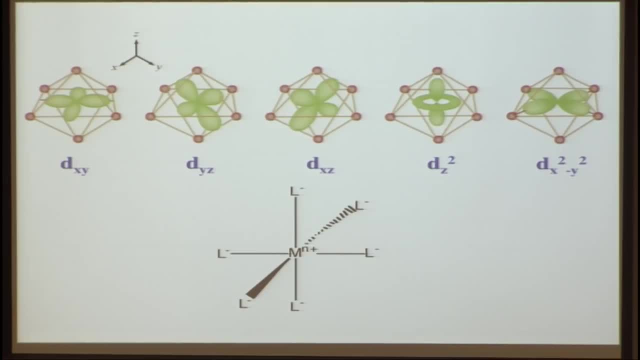 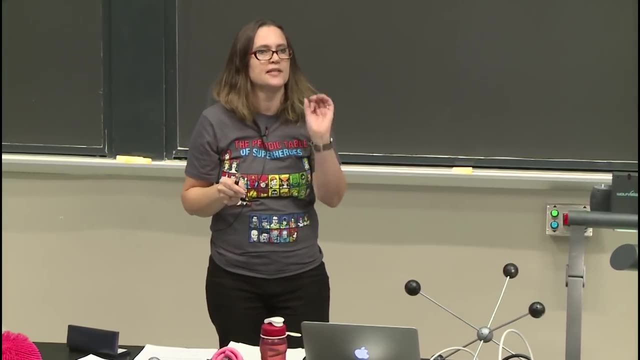 at the d orbitals. So one could think about the fact that these are not going to be not as much repulsion. This is a lot of repulsion, All right. so let's go through orbital set by orbital set and consider how repulsive it's going to be compared. 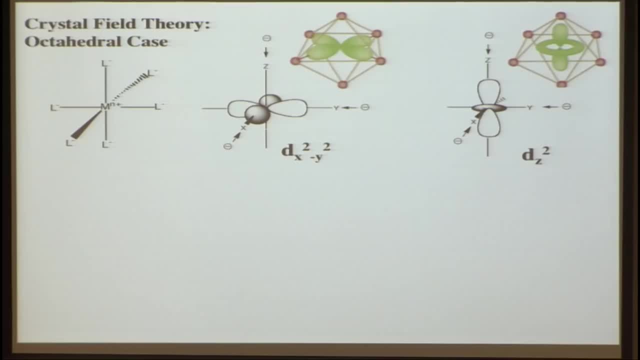 to the other orbitals. So if we look over here at the octahedral case- and I have both- these drawings were on the first page of your handout. This is on the second page, But you can think about them Here. it's drawn more where they're all. 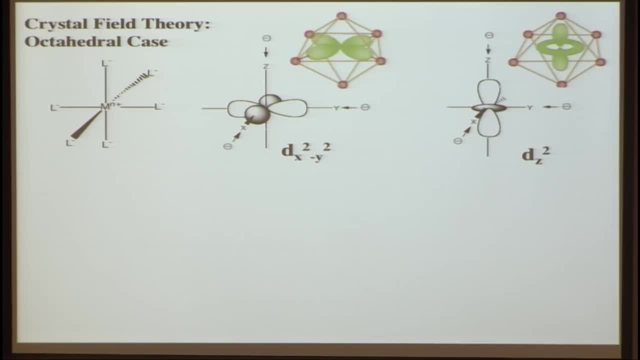 drawn kind of the same way. Here it's sort of moved a little so you can see better. So we can keep both of these in mind. So again the negative point charges around the orbitals here And on these drawings. I have these little negative signs. 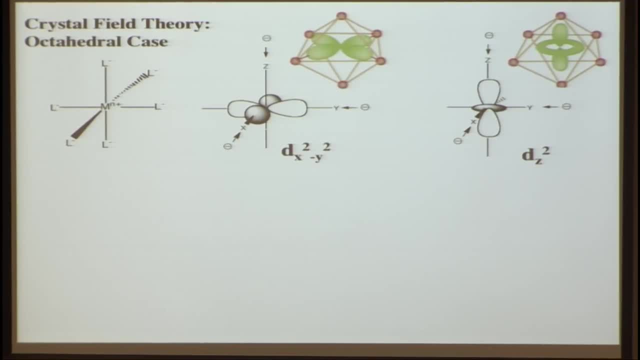 pointing in to give you a sense of where those negative point charge ligands are coming. So we have our dz squared And we can see the negative point charge right toward this maximum amplitude along z. So that's going to be repulsive dx squared, y squared- same thing: point charges. 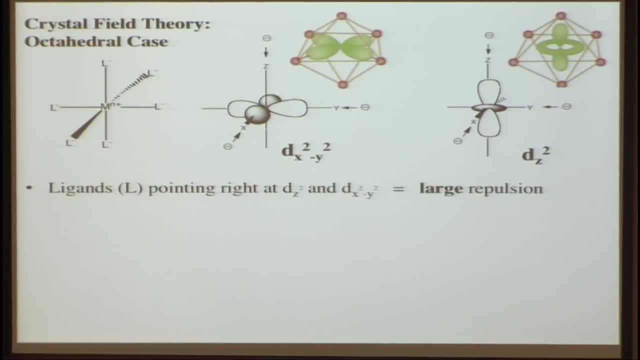 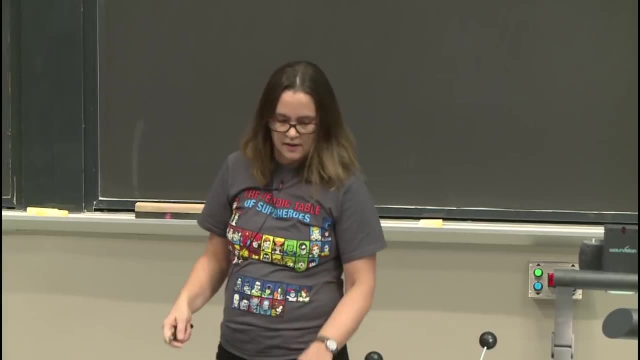 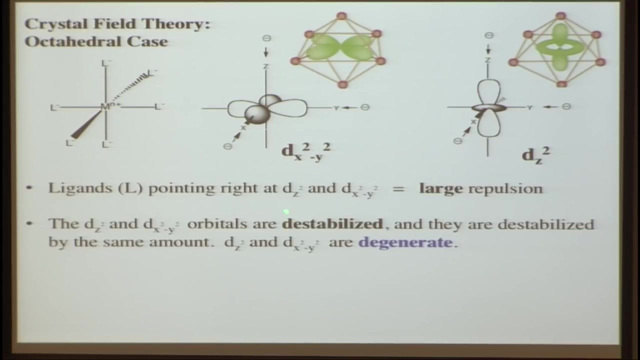 right toward these. So the ligands point directly at dz squared and dx squared minus y squared. So there's a large repulsion there. And in this particular case, in the octahedral case, what turns out to be true? both of these are destabilized. 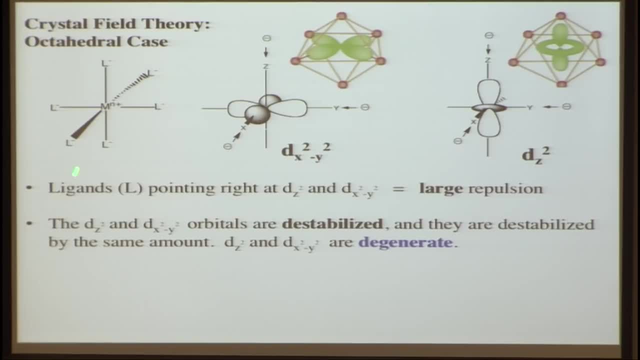 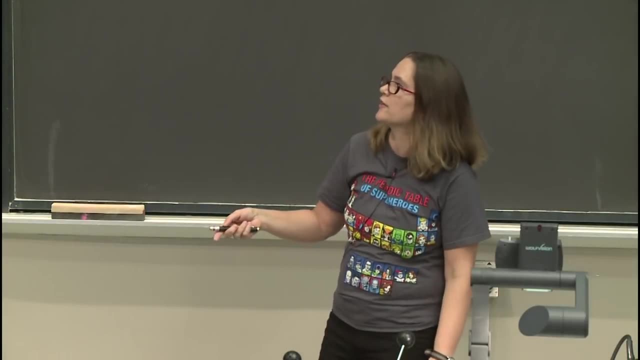 And they're destabilized, actually by the same amount, And so that means that they're going to be repulsed, which means that they have the same energy which we learned before, means that you could say they're degenerate with respect to each other. 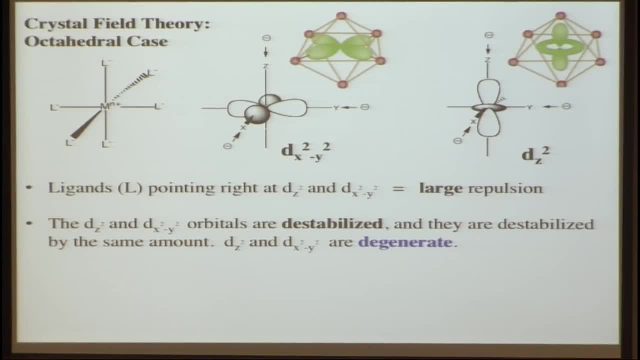 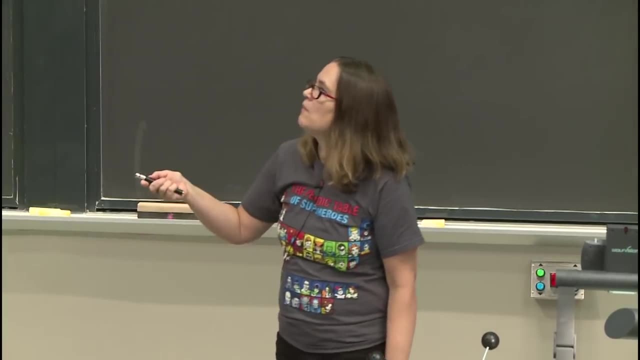 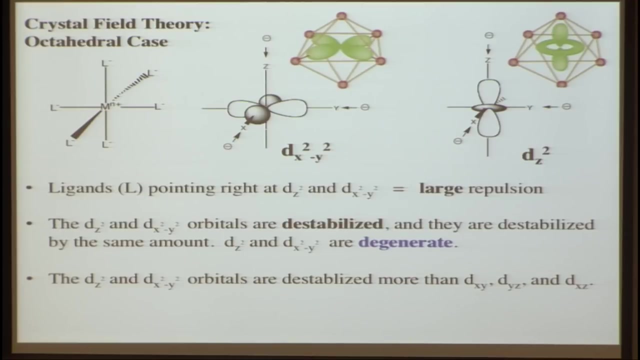 So both of these big repulsion, both are destabilized by those negative charges by the same amount And you have much more repulsion and much more destabilization for these two orbitals compared to the other set of orbitals, the ones that are 45 degrees off-axis. 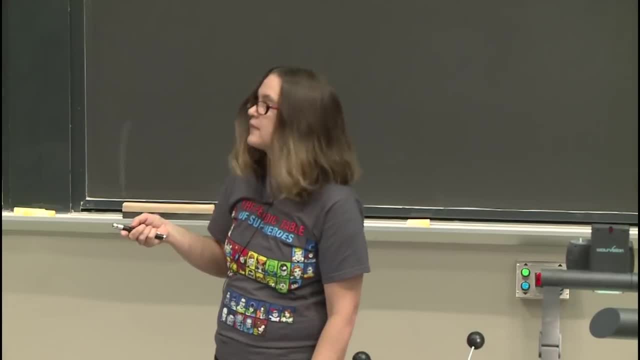 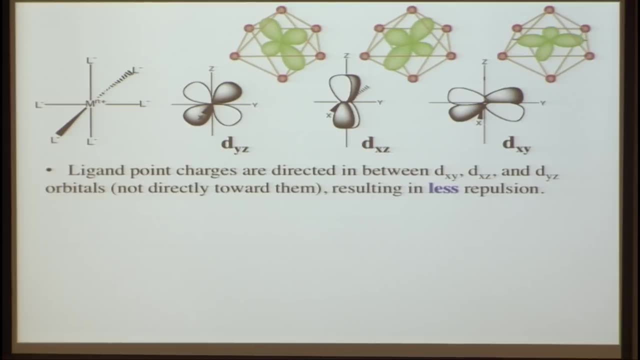 Now let's look at these and look at where the point charges are. So this is the picture in your handout. I just kind of put these up there too so you can think about where those point charges are for octahedral geometry: 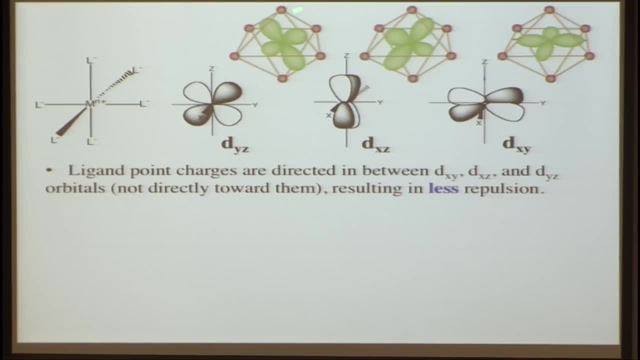 So the ligands again now are not pointing right at the orbitals, They're off-axis. because the ligands are on-axis and the orbitals are off-axis, so they're not directly pointing toward each other, And so this is a lot less repulsive. 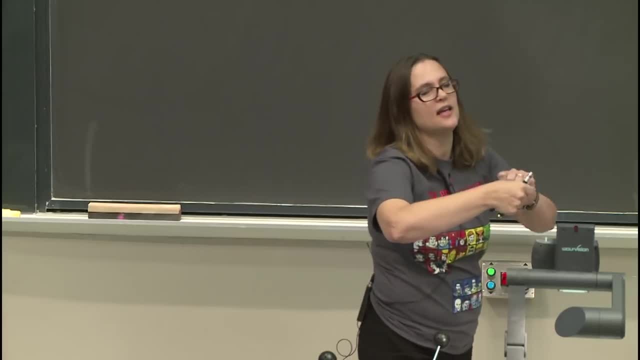 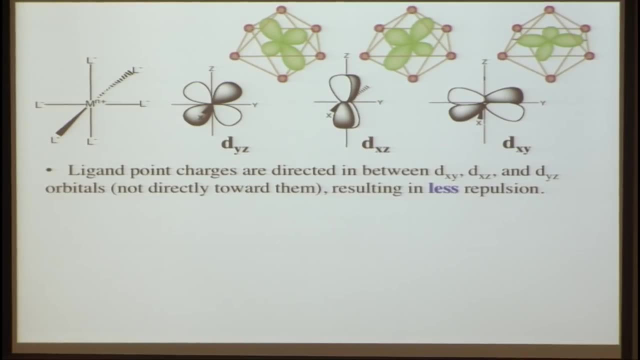 OK Than the other situation where you had the ligands and the orbitals both on-axis, pointing right toward each other. So now, this is why it's important to know which orbitals are 45 degrees off-axis, because we now can think about the fact. 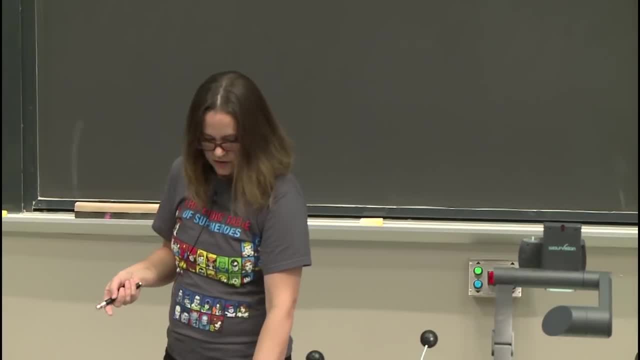 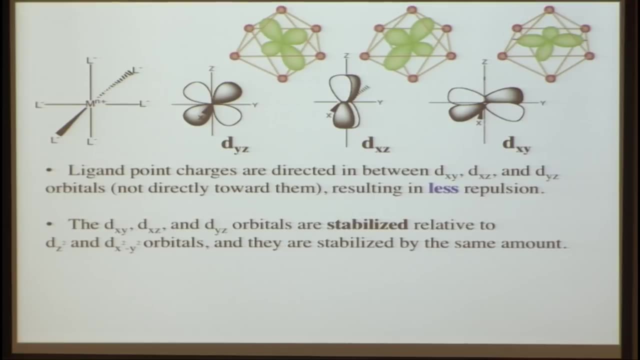 that there'll be less repulsion in this case. So we can say then that d, xy, y, xz and yz orbitals are stabilized compared to dz squared and dx squared minus y squared orbitals, And they're also stabilized by the same amount. 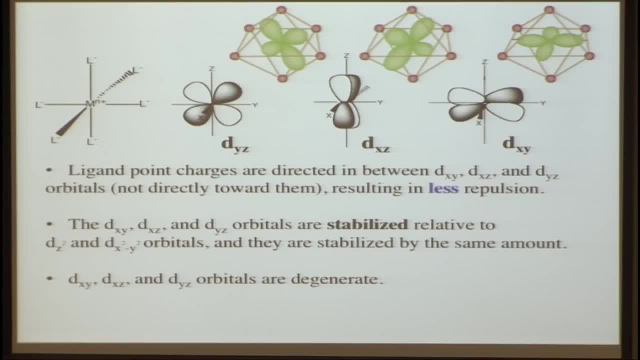 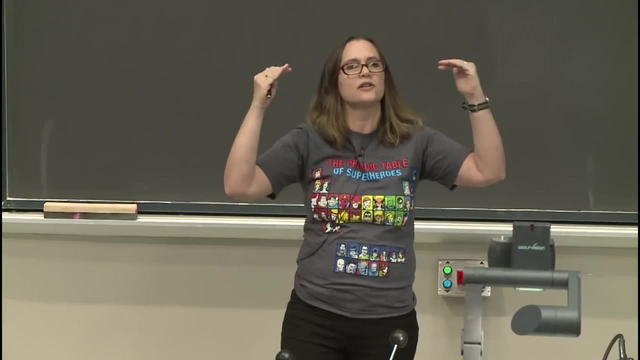 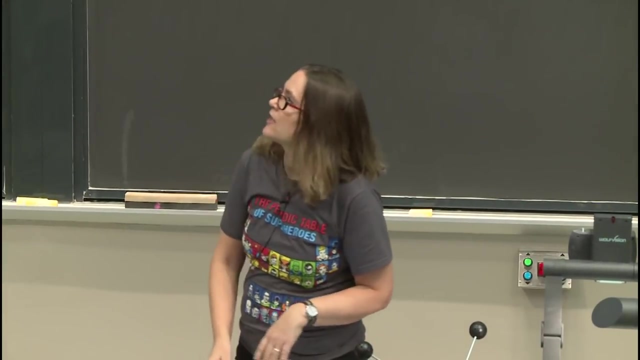 So these are also degenerate. with respect to each other, They have the same energy. All right. so we have these now, two sets of orbital types: two orbitals that are destabilized and three orbitals that are stabilized compared to them. So now let's draw what's known as an octahedral crystal field. 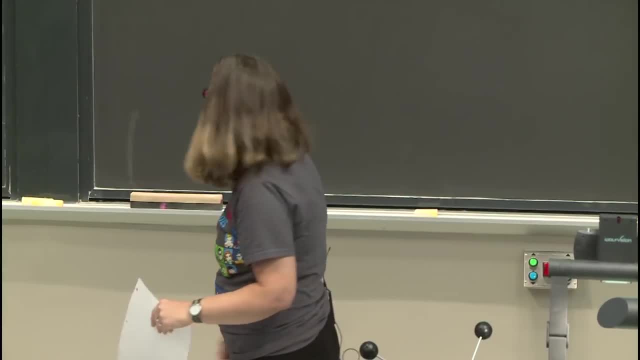 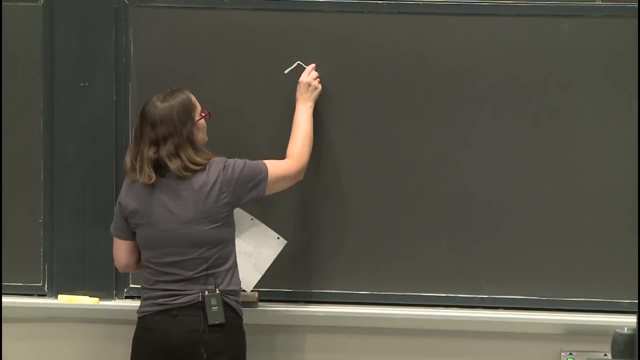 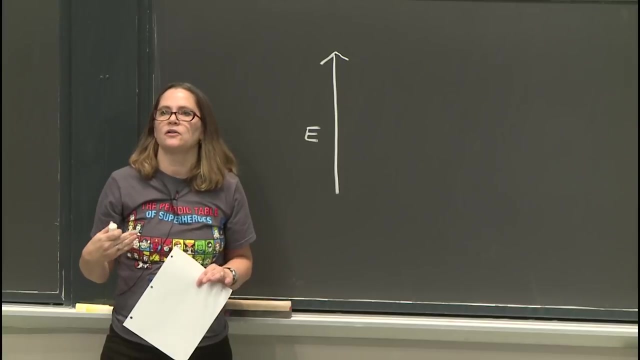 a splitting diagram and think about what's happening. So I have some over there. Ignore those for now. I'm going to draw one over here. So first we have energy going up And we have a situation. We first want to think about what would be the case, say, if you had ligands everywhere, not just on the axis, not octahedral geometry, but just everywhere. So if you had ligands everywhere, you would have your five d orbitals. all would have the same energy Because all of them, there's ligands everywhere. 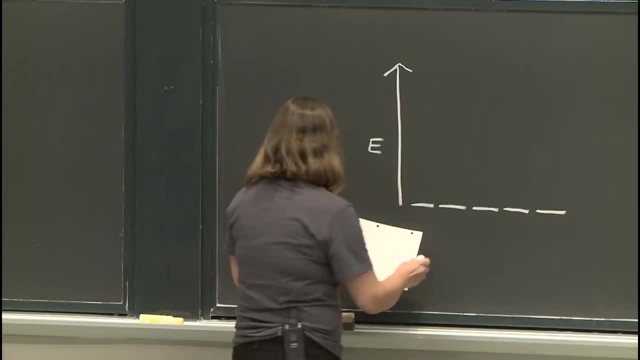 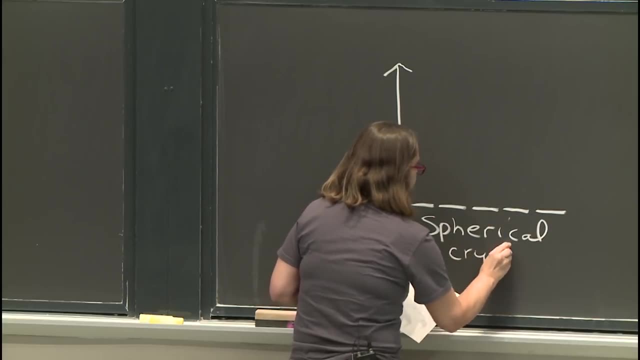 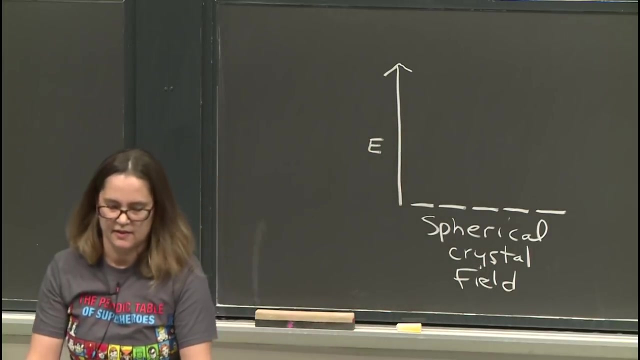 all of them would be experiencing the same amount of repulsion. So this would be the case for a spherical crystal field, And I like to think about this with this prop. I had this before as an s orbital. It's convenient for that. 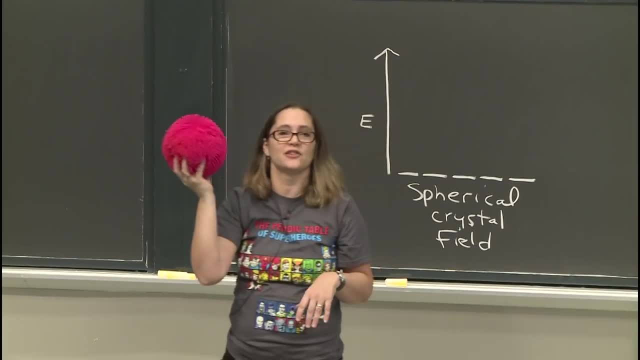 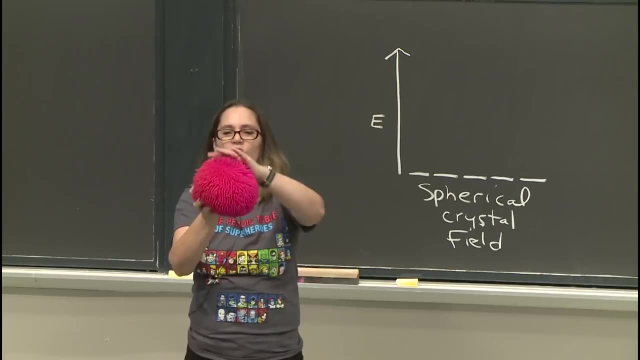 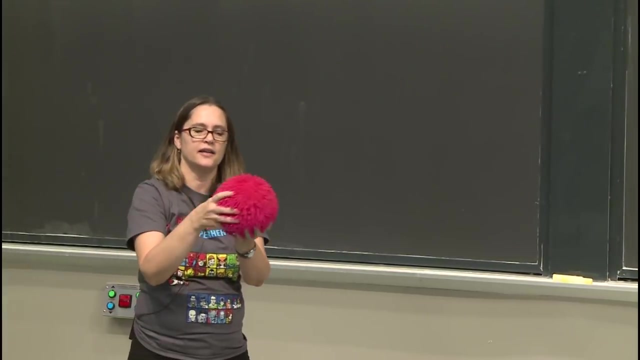 Well, but really what it is is a hypothetical spherical crystal field, because these are all little ligands And you can see, these little ligands are completely symmetric around And if you feel sort of the inside, there's something in there. Well, that of course is a metal ion. 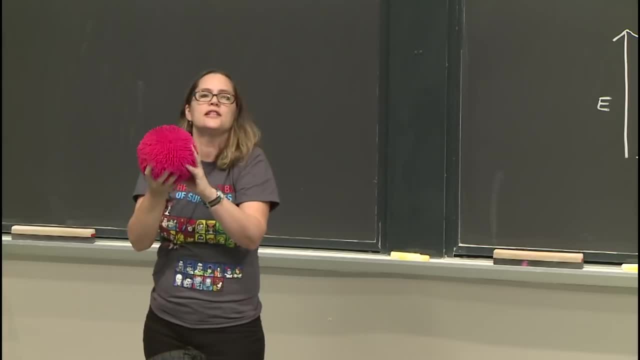 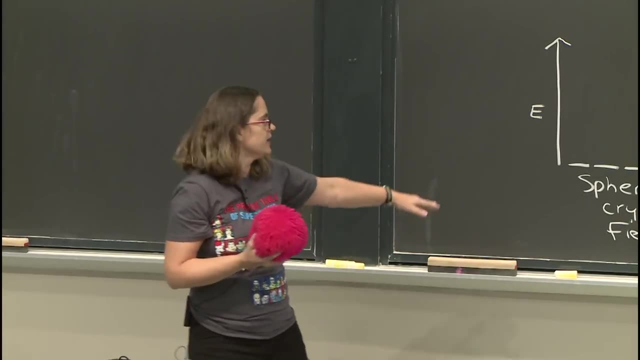 And these ligands are completely around, So all the d orbitals are equally feeling the repulsive effects of these ligands And so they all have the same energy In this hypothetical case. I was so excited when I found this at CVS. 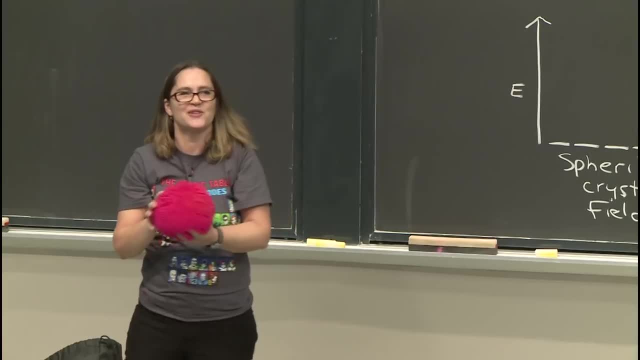 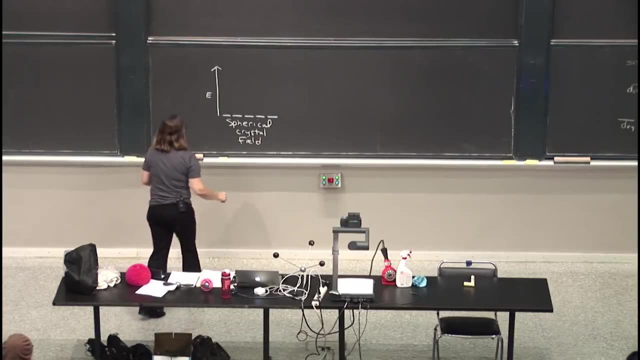 And I went up and I was like, wow, you sell hypothetical spherical crystal fields here. And the person was not amused. OK, So now what happens? because this is not the case. This doesn't exist. This is just hypothetical. It looks like it exists, but it doesn't. 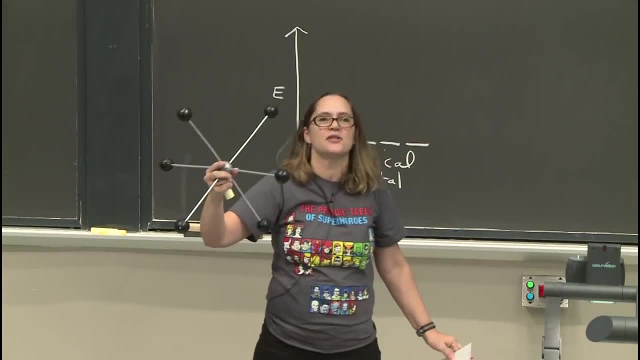 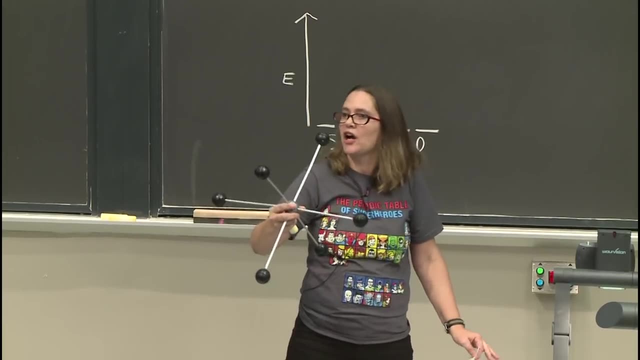 This is what really exists. You have certain geometries. The ligands come together with the metal and form particular geometries, And we already talked about what those geometries are. There's not a whole lot of variation. We get the same kinds of geometries. 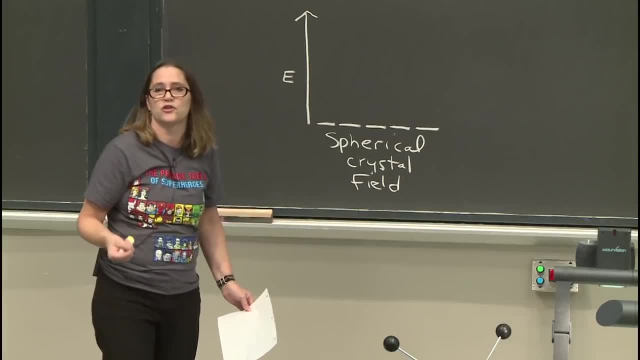 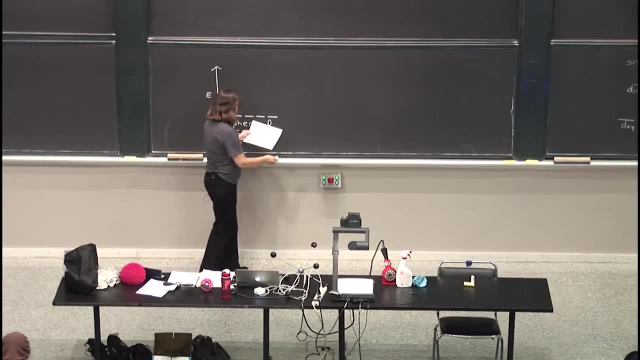 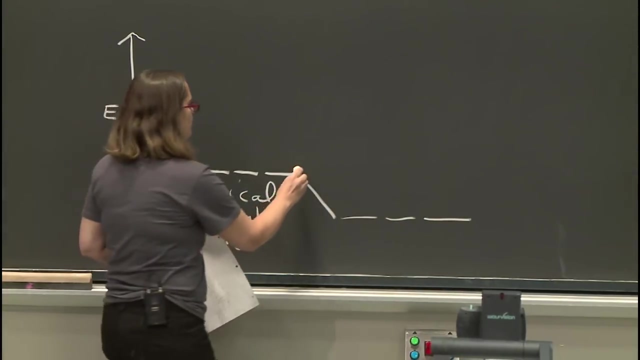 And octahedral is the most common geometry for a transition metal complex. So what's going to happen here? So the ligands will now split the energy of the d orbitals And three of them are going to go down in energy. They're going to be stabilized compared to the two that 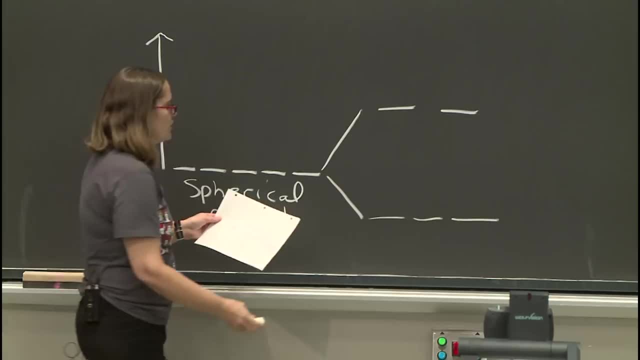 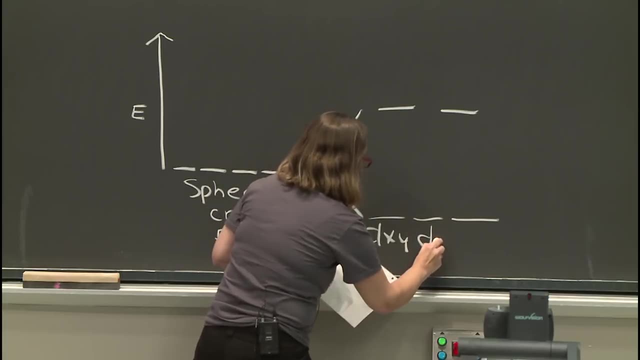 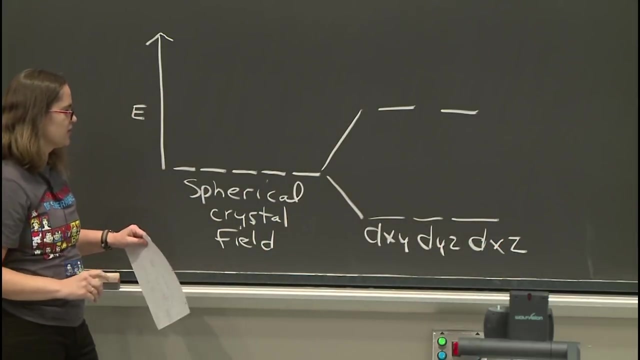 go up in energy. So the three that are stabilized again are d x y, d y z and d x z. If you can't read this, it all should be in your handout. so it's OK, You don't have to read my handwriting. 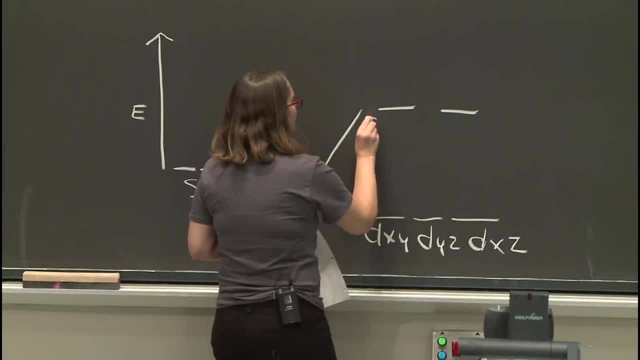 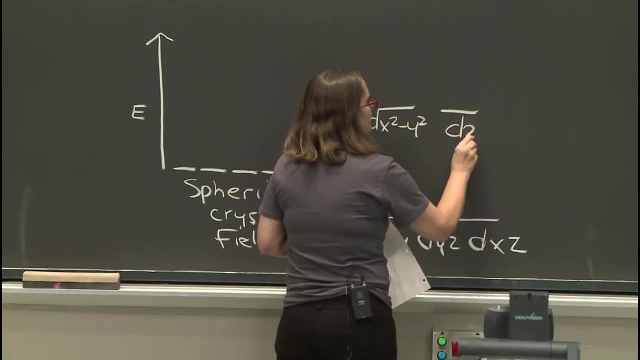 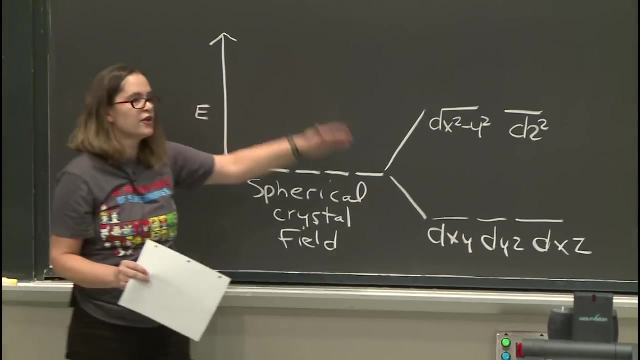 And just follow along in your notes. And then the ones that have the most repulsion are d- x squared, minus y squared, and d z squared up here. All right, So two go up in energy, There's more repulsion. Three go down in energy. 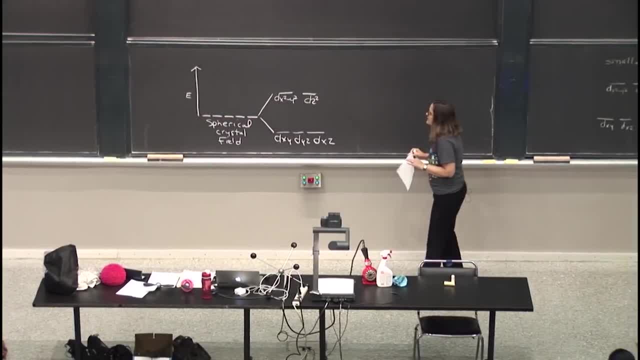 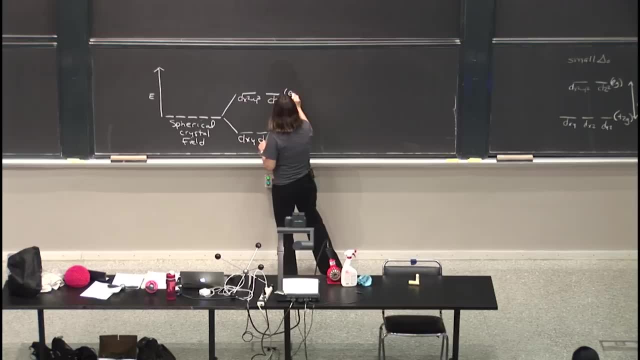 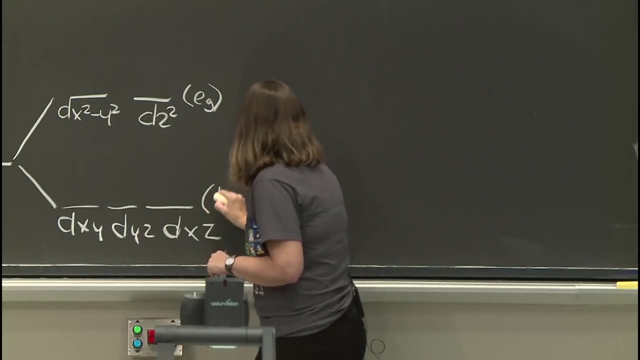 And instead of writing all of those d's and x's and y's, they're little abbreviations that people use, So they call these two orbitals the e- g orbitals. So those are the ones that are destabilized, And the ones that are stabilized are called t to g orbitals. 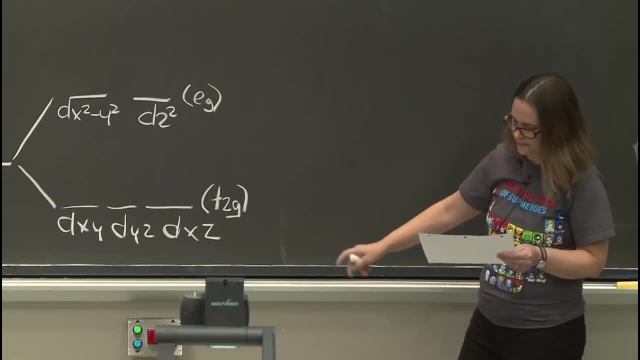 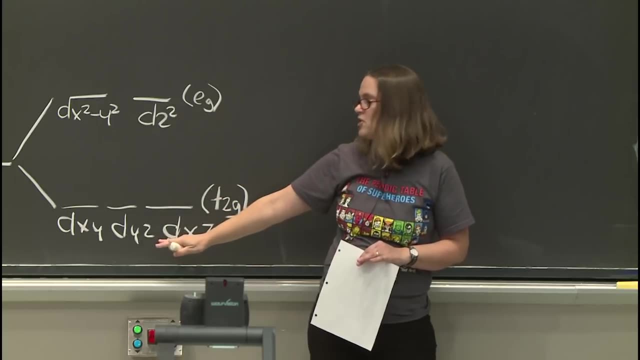 which is going to make our nomenclature easier later on. These two, again same energy. I tried to draw a straight line between them. They're degenerate with respect to each other. These three have the same energy, Again degenerate with respect to each other. 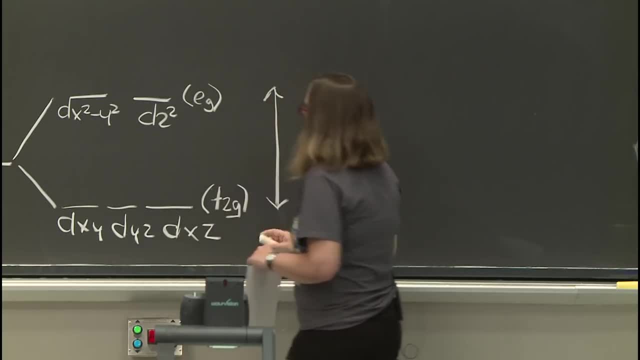 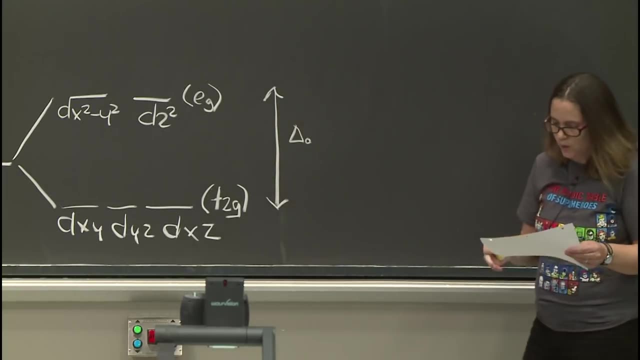 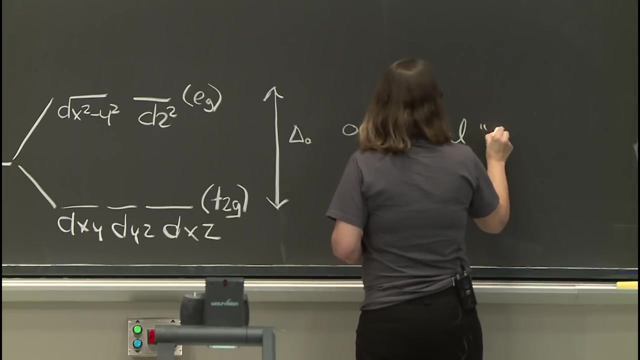 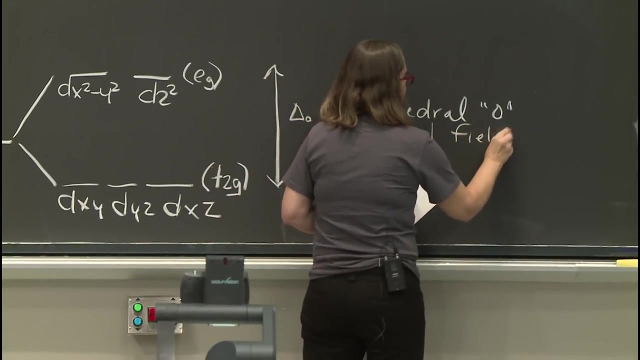 And then the difference of how much it's being split. this energy difference has a special name. It's sort of this delta sub o And this is the octahedral And that's the o. The o is octahedral, crystal field splitting energy. 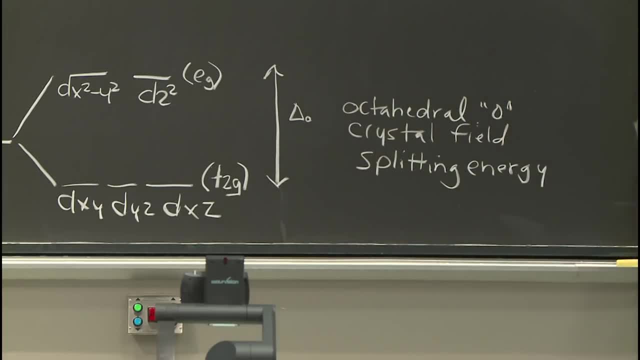 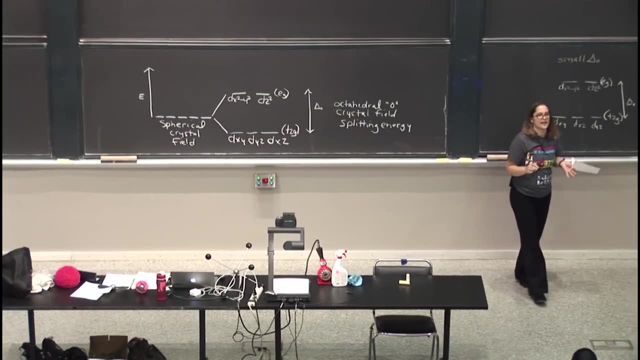 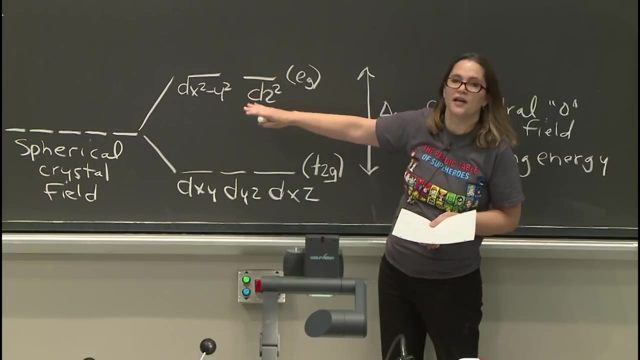 because it's the energy that shows the splitting of the crystal field. So that's at least a good name for it. All right Now. overall this energy is going to be conserved. So the octahedral, The orbitals that are destabilized, and two go up. 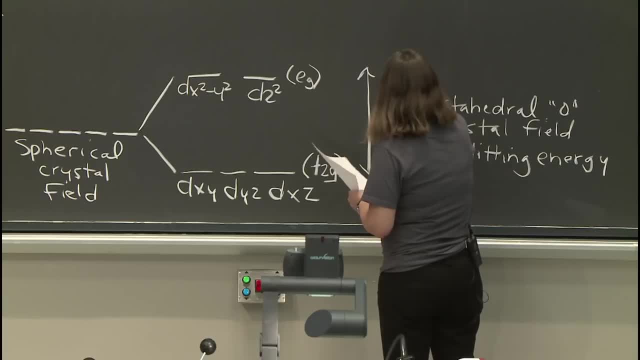 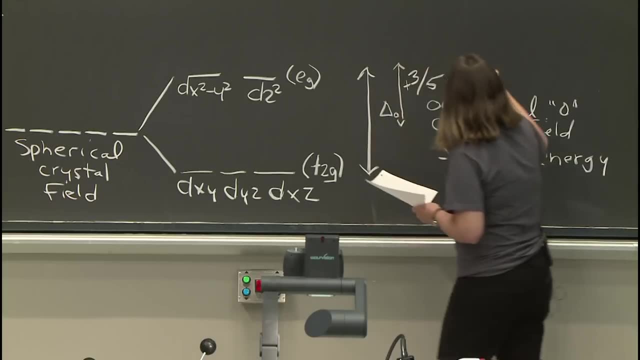 and three go down. So we can also put that the two that go up go up by 3 fifths times the octahedral splitting energy And the three that go down are stabilized, go down by minus 2 fifths times the octahedral crystal field. 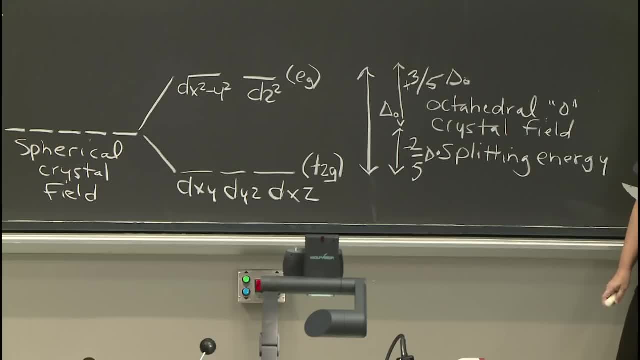 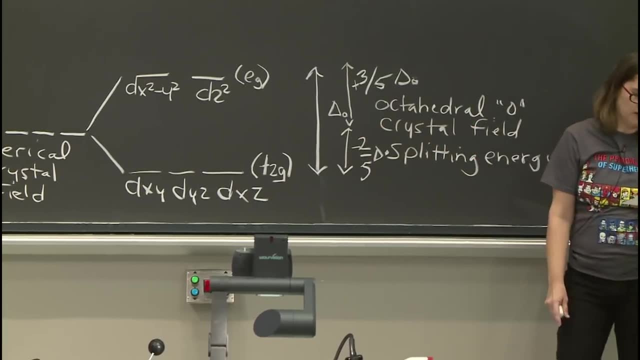 splitting energy. This is why I have it in your notes, because you can't really read my writing too well. So two are destabilized up by 3 fifths. Three are stabilized down by 2 fifths in energy. All right, 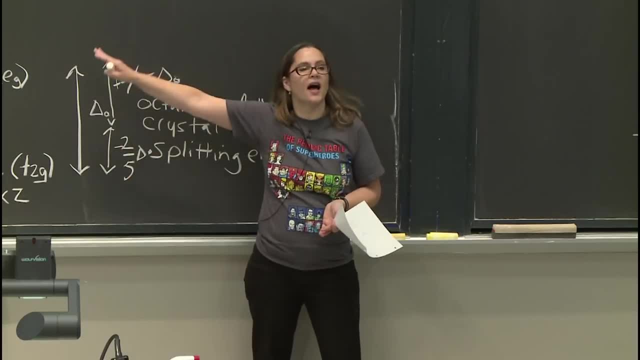 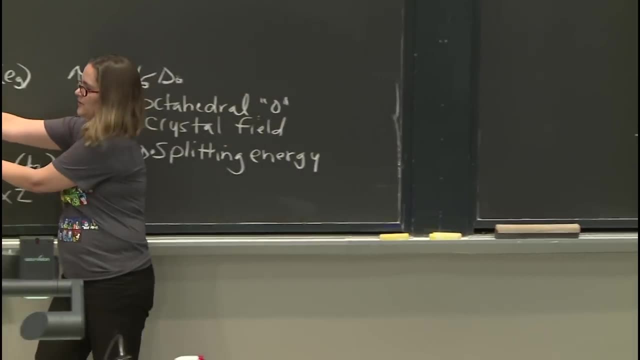 So now, what controls the overall size of this splitting energy? How do you know? Is it a small splitting? Is this, should I have drawn this- that they're just tiny bit, Or is it like it could be a really large splitting? 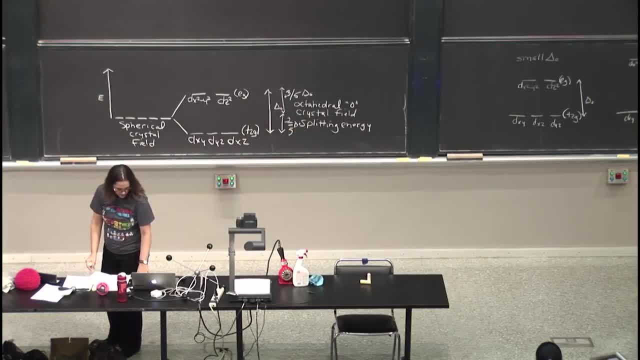 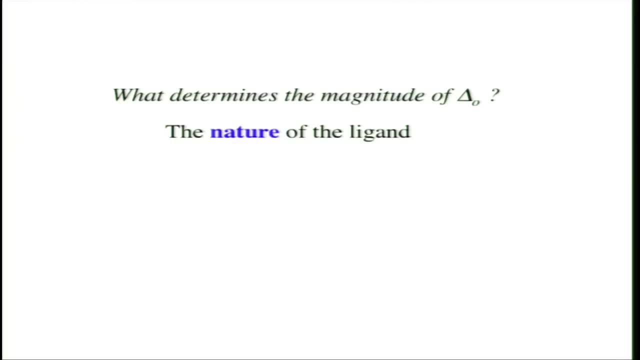 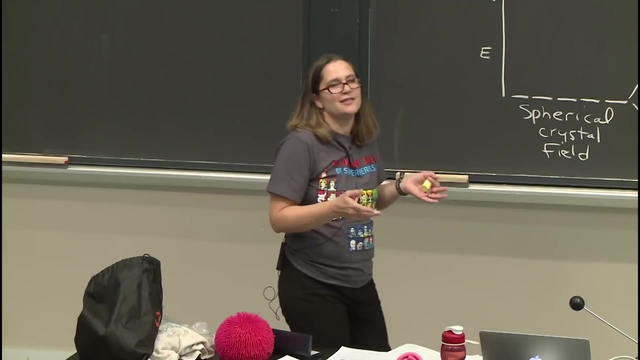 What determines the splitting, the magnitude of this splitting Right, splitting energy. So what determines that are the nature of the ligands. So some ligands are really repulsive, big splitting, Others you barely notice, they're there, very little splitting. 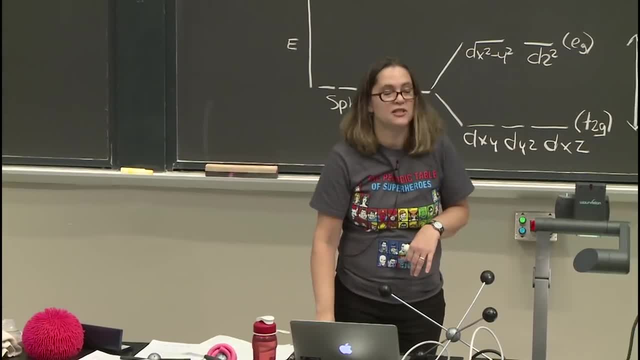 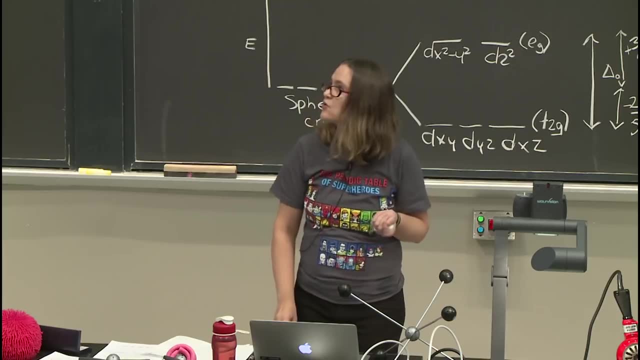 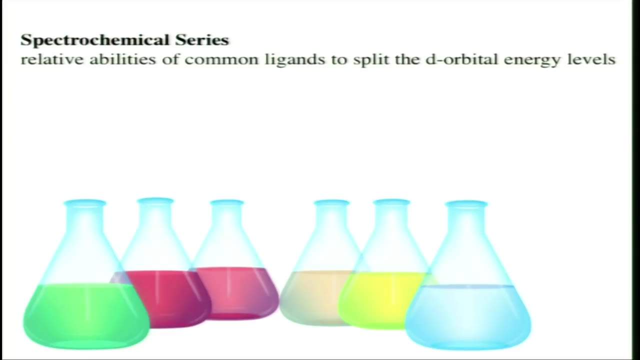 There's always some splitting, but it can be different. So the relative ability of a ligand to split the crystal field gives rise to what's known as the spectrochemical series. So it's the relative ability of common ligands to split the energies of these d orbitals. 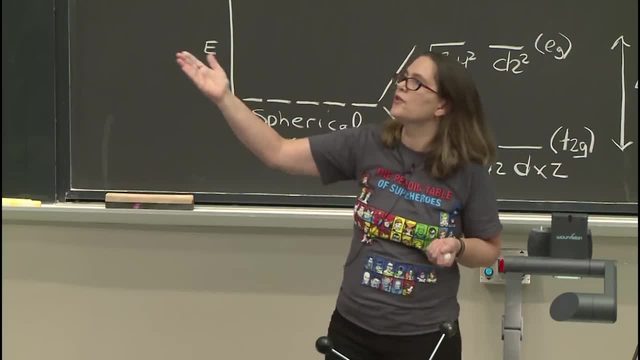 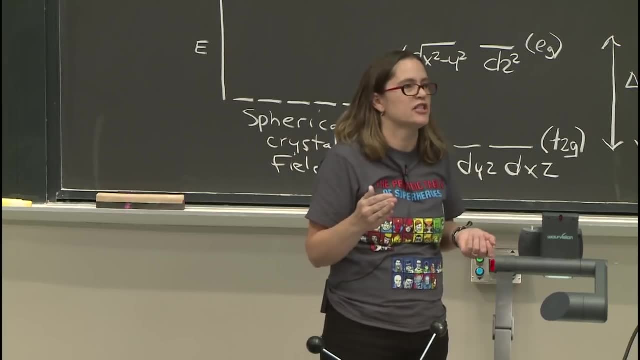 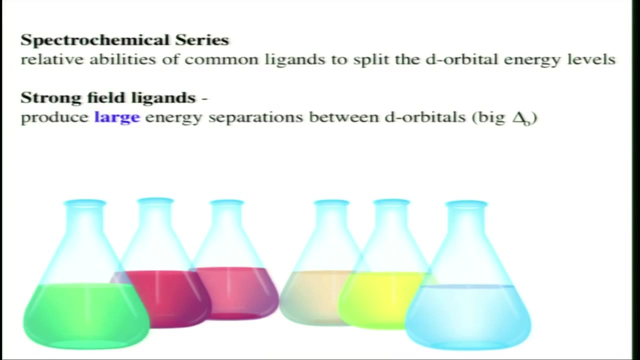 And this is what gives rise to these beautiful colors. So all of those colors are possible from cobalt compounds, every single one of them, Because different ligands will split the energy different amounts, giving rise to those different colors. So we have what's known as strong field ligands. 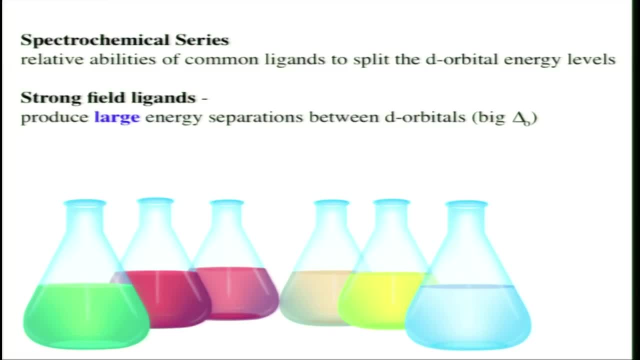 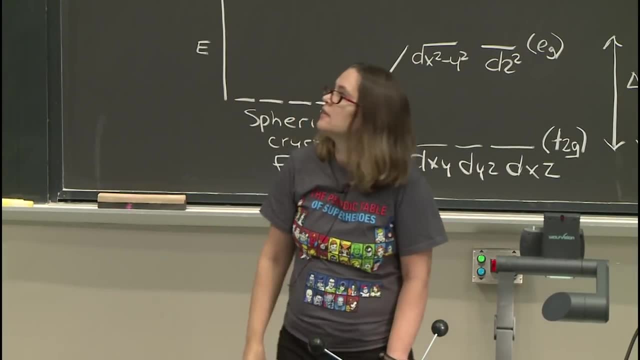 And as that name would suggest, they suggest strong field ligands are going to have a large splitting. They're very strong, They split to a large degree And we have weak field ligands. Weak field don't cause much of a splitting. 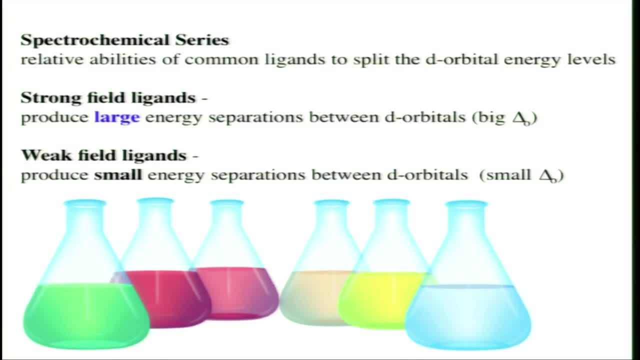 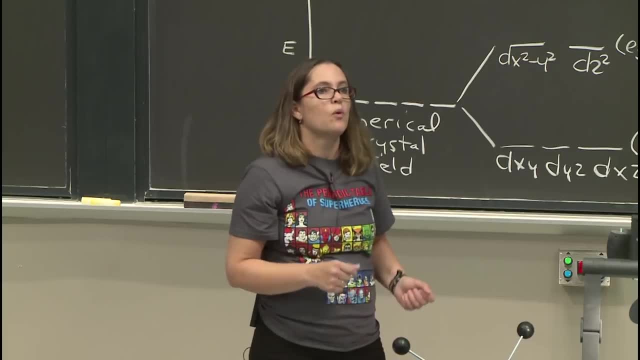 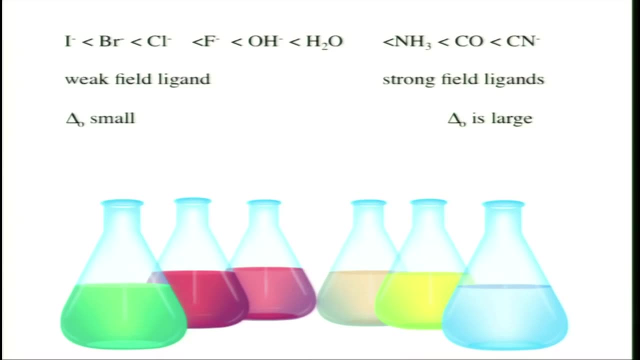 It's a small delta sub O, small octahedral crystal field splitting energy. All right, so which common ligands fall into which categories? Here is the list that we talk about pretty much in this class. I don't think there are any other ones. 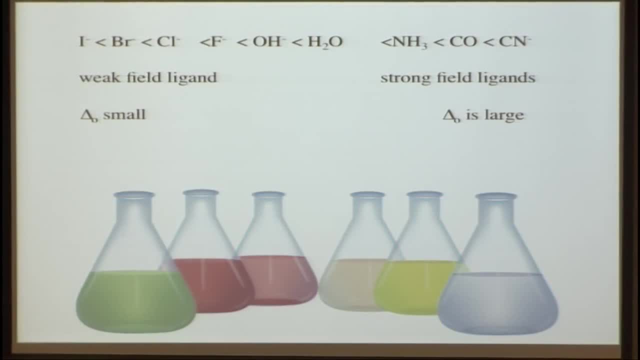 So what I will put on your equation sheet. your equation sheet, for example, has lots of cool, interesting things that were not on the other equation sheets And I will tell you which are weak field and which are strong field. But I will not tell you that weak field means. 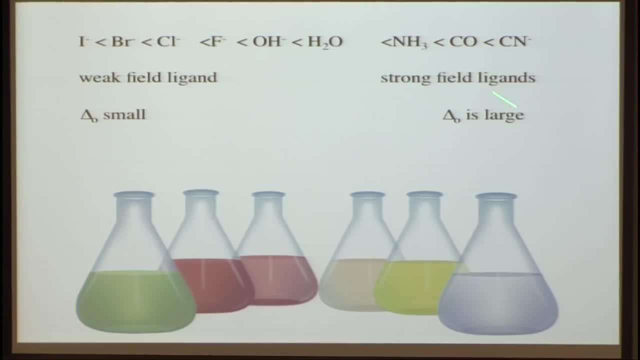 that it's a small splitting. That's something that you need to know- Or that strong field means it's a large splitting. But I will tell you that your halides down here are weak field ligands, Water and hydroxide are sort of in the middle. 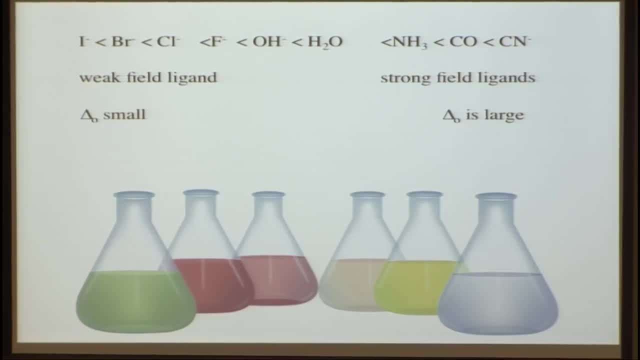 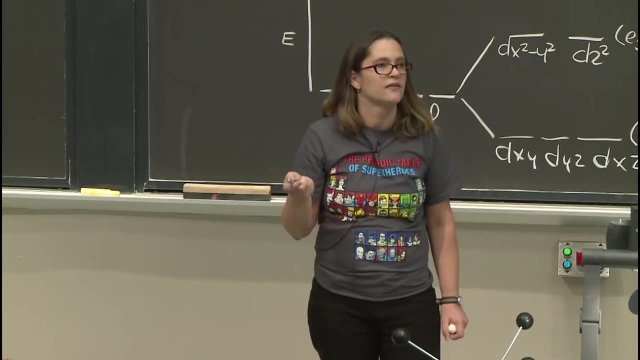 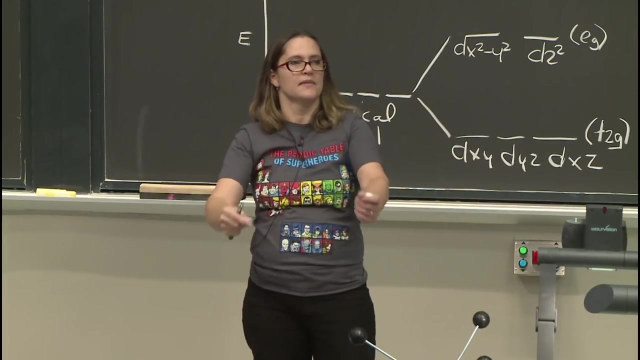 And they can have all sorts of different colors. when they're bound to coordination complexes, They're sort of intermediate And then your strong field ligands, with your strongest being cyanide. very strong field ligand, All right. so if your metal has a weak field, intermediate field. 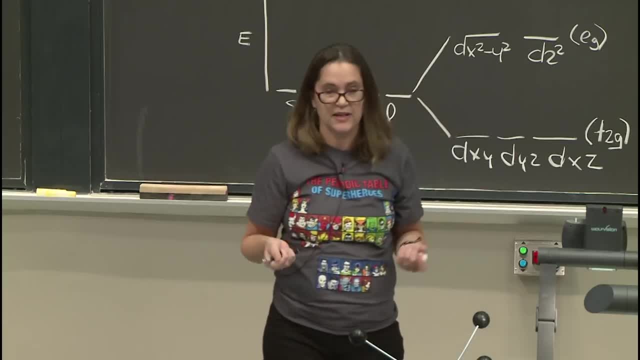 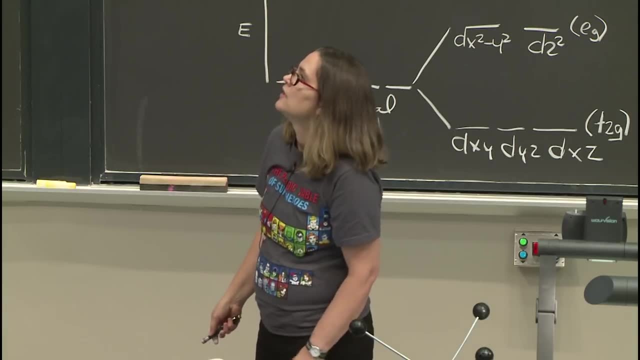 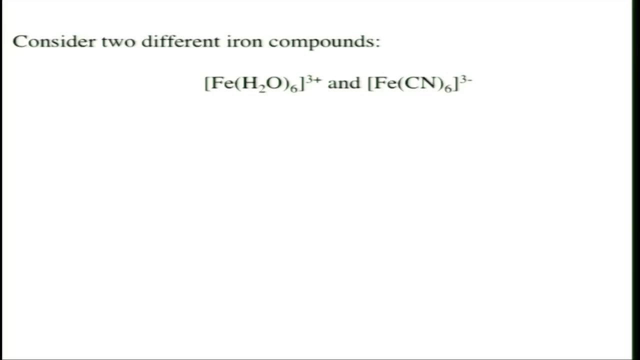 or strong field ligand. it can have very different properties, especially very different colors. Also, it could be paramagnetic or diamagnetic, Depending on this. So let's take a look at two different iron complexes. We have iron with six waters with a plus 3 charge. 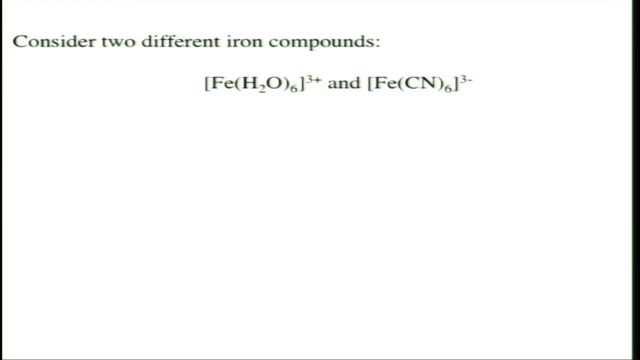 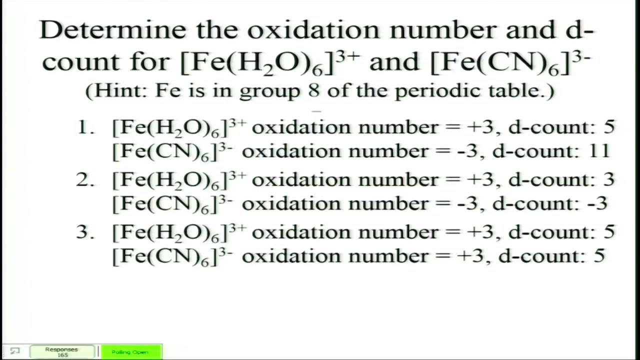 and iron with cyanide, with six cyanides and a minus 3.. So the first thing we have to do is figure out the oxidation number of the iron and the d count, And that's our first clicker question. All right, let's just take 10 more seconds. 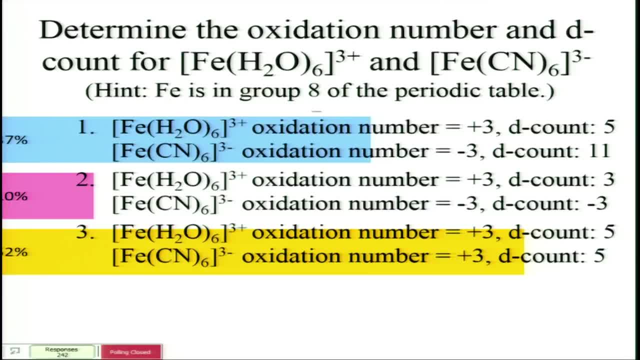 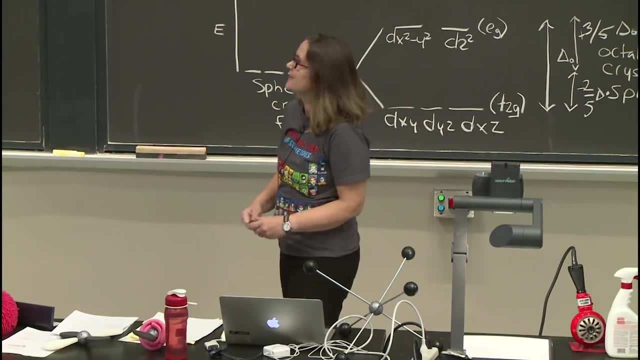 OK, there we go. There's the right one. A little more people say that: All right, so let's take a look at this And you will get used to thinking about what the charges are on the various ligands. So here we know that the overall charge 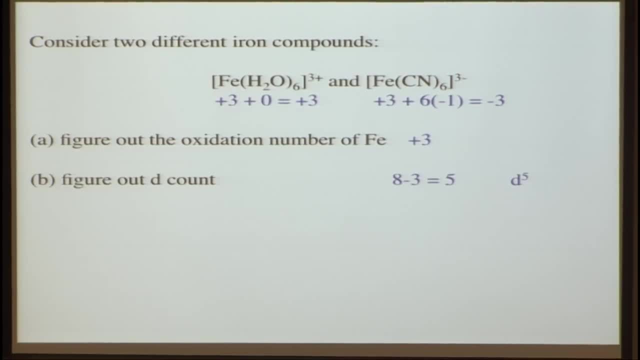 has to be the same as the overall charge on the complex Water is neutral and so that means this iron has to be plus 3.. Cyanide has a minus charge And you may have noticed that in the list of ligands that it was Cn minus. that when I just showed you. 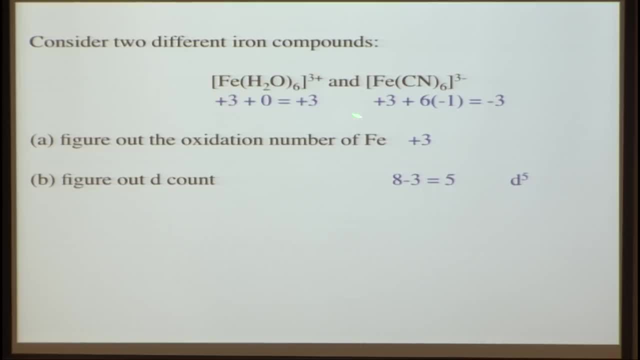 the strong field ligands. So there's six minus 1s and so it's also plus 3 to give you an overall charge of minus 3.. And as you do these problems and problem sets, you'll become very familiar with what the charges. 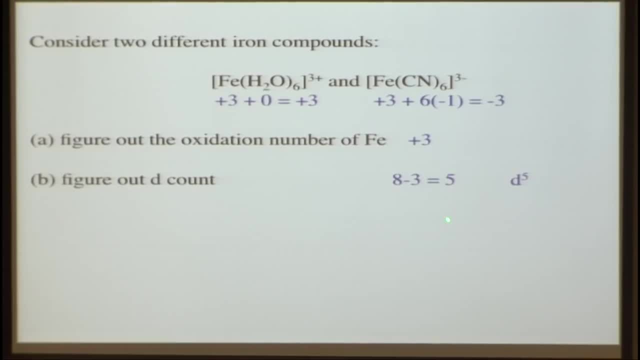 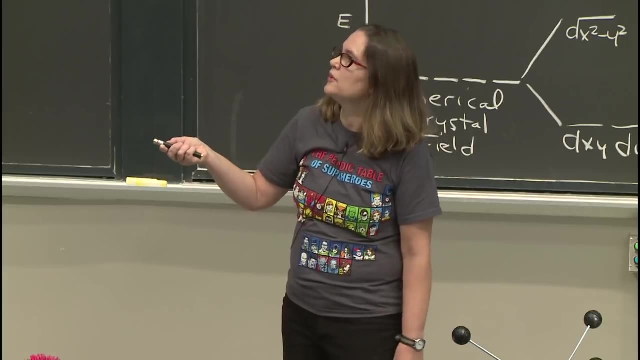 of the different ligands are. So, overall plus 3, 8 minus 3 is 5.. It is a d5 system. So the next thing we're going to do is we're going to draw our octahedral crystal field. 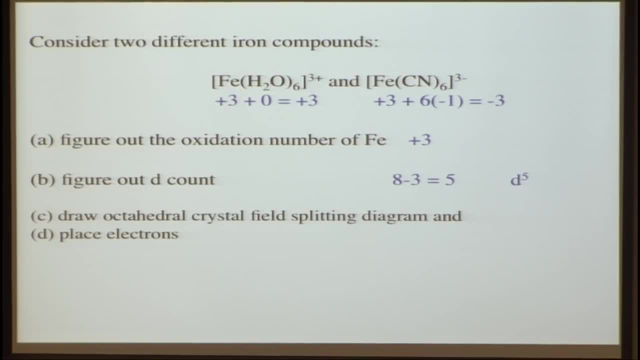 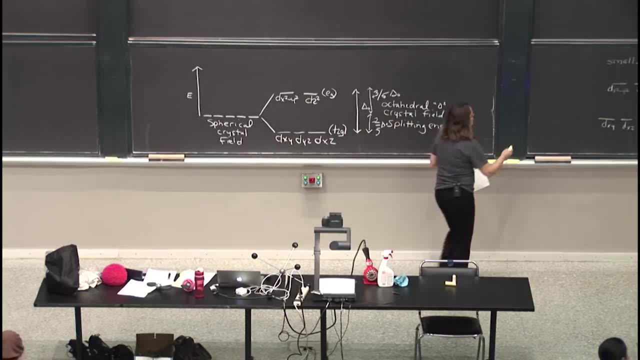 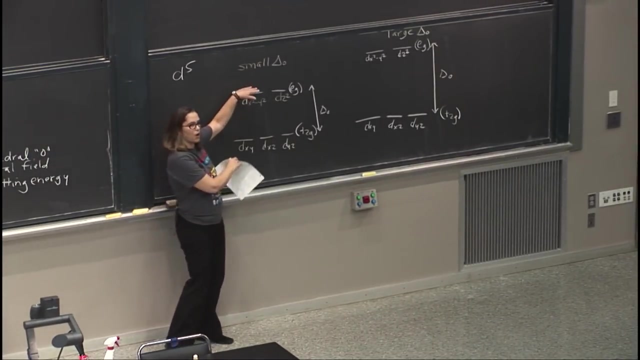 splitting diagrams and place electrons And I already have over here a starting place for those. So we're doing here our d5 system And we have a diagram with a small splitting and one with a large splitting. So with the small splitting, is that? 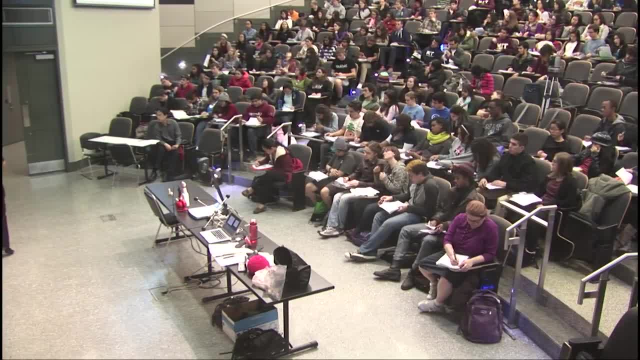 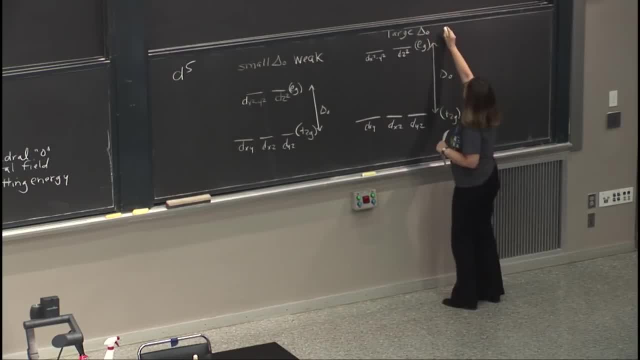 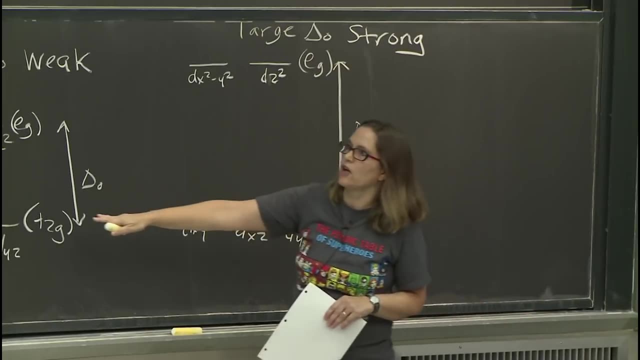 going to be a weak field or a strong field. Weak field, That would be a weak field, And when we have a large splitting, that is a strong field. So which of our two compounds is going to be the weak field compound And which will be the strong? 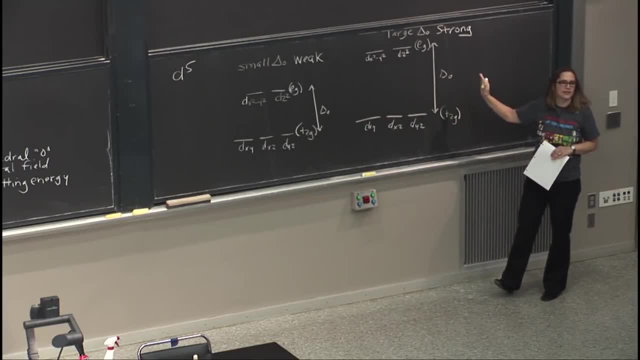 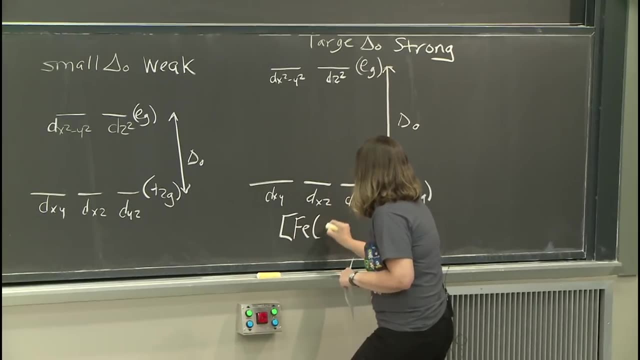 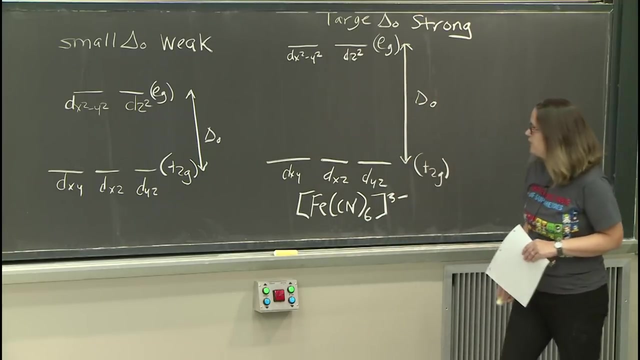 Let's do strong first. Which one has a strong field? ligand, Strong, Strong, Strong, Strong, Strong. Cyanide, Cyanide one. So this one is going to be our cyanide complex because it has the strong field, And so this one would be the water. 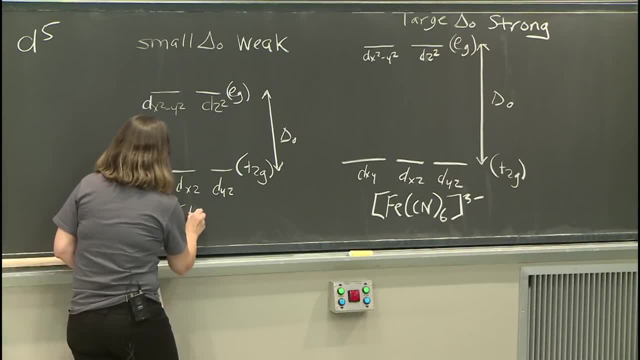 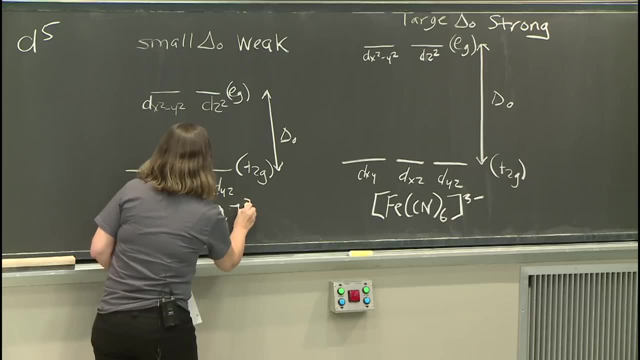 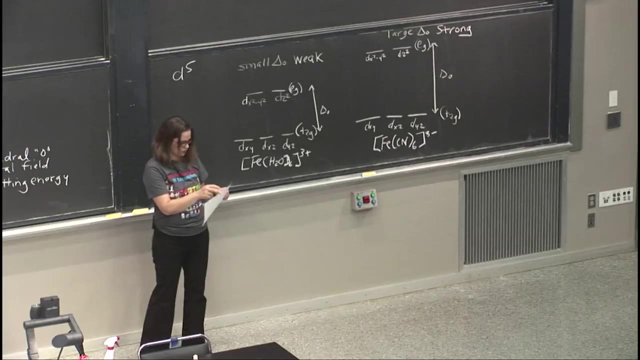 Water's intermediate. so you kind of have to see what the comparison is first before you decide. 6, bracket 3 plus OK. So here we have water, There we have cyanide. So a weak or intermediate field versus a strong field. 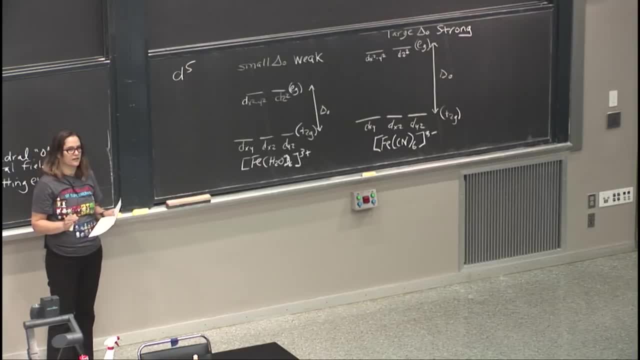 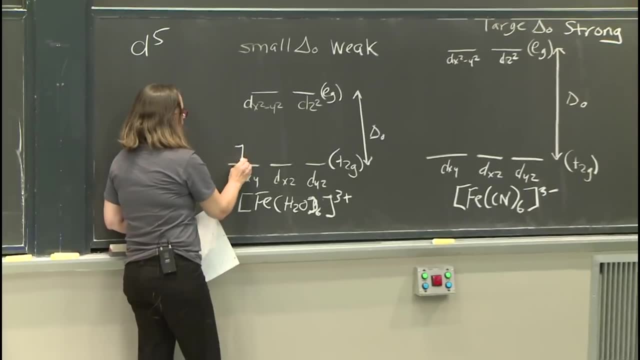 All right, Now we need to put electrons in here, So I have to decide. I have five electrons I'm going to play with And I could put them in here. Let's just start here. Do 1,, 2,, 3.. 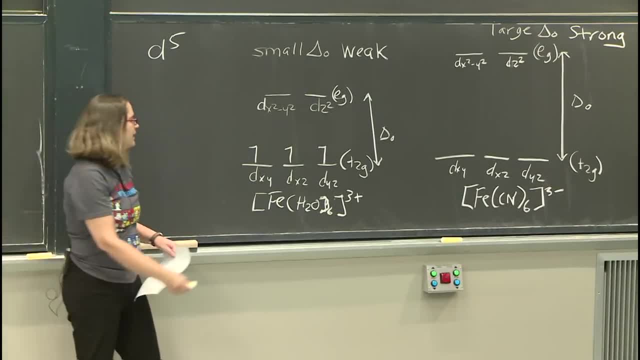 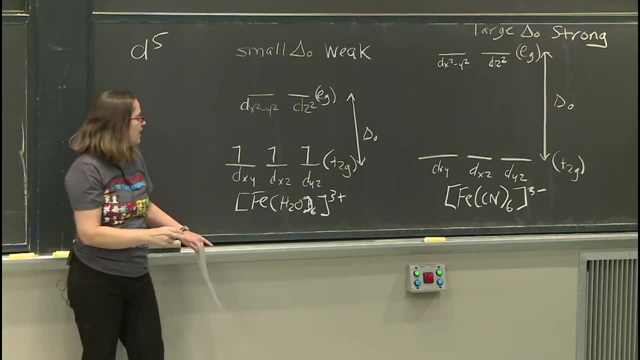 Now the question is: where am I going to put 4?? Am I going to put 4 down here or put it up here? And so here, it depends on if I put it down here. I'm pairing And you know the seats on the bus. 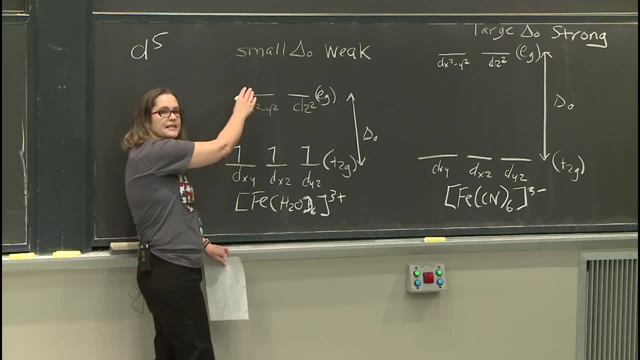 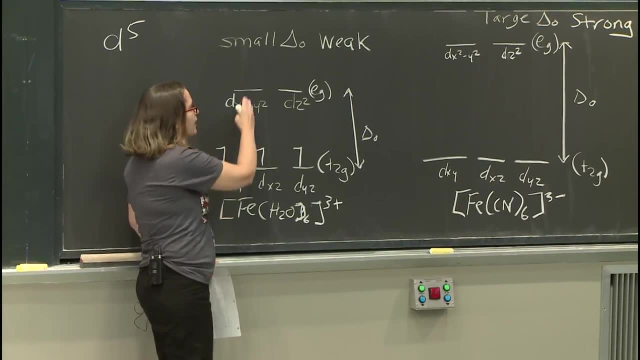 People don't really want to sit together if they're empty seats. Now they're empty seats up here. So the question is: is it going to take more energy to pair or more energy to put it up here Now? if this is a weak field- which it is- 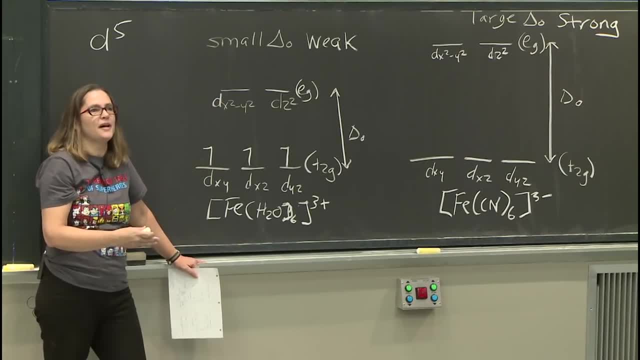 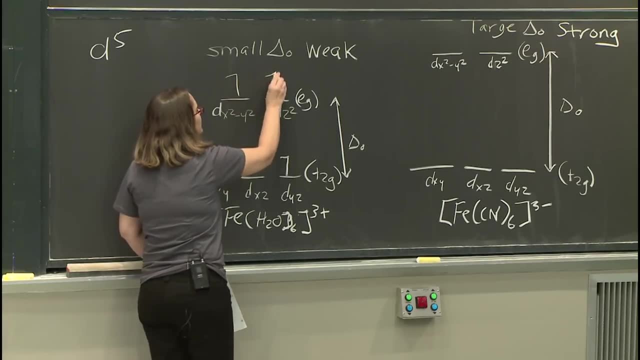 then that's not all that far away. You get on a bus and you see a seat in the back. you'd rather sit up front, But you're like then you have to sit with someone, so you go to the back. So that's what happens with a weak field. 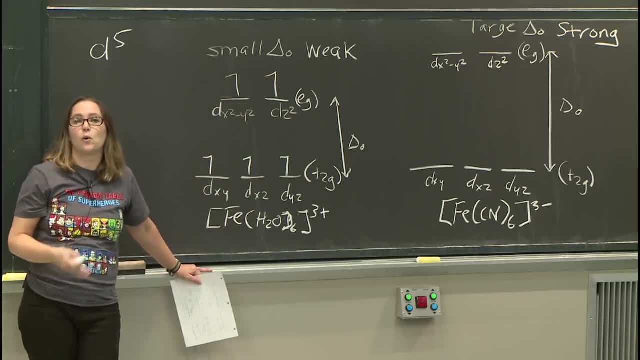 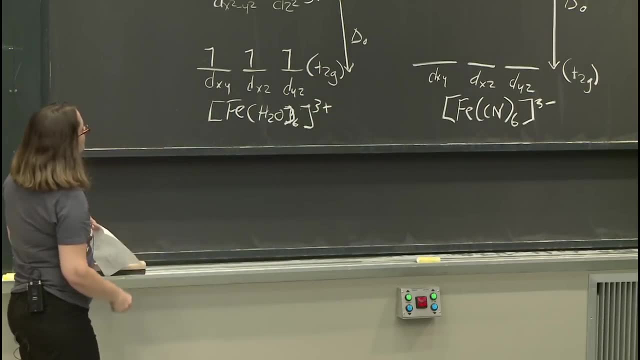 OK, So the other energy levels are just not that far away. so you go up there, And if I kind of move it up for just a second and then I'll say, so this rule here, and I'm going to kind of cover this up again. 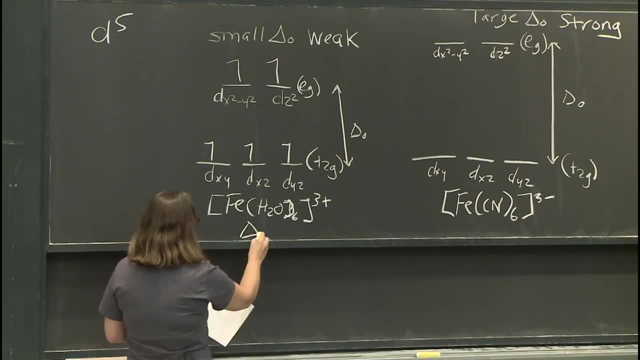 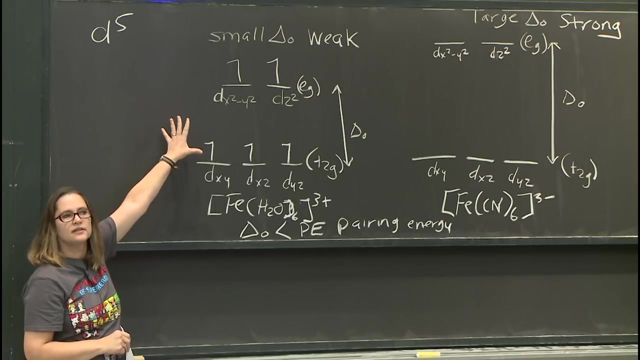 but maybe I'll just put it down here. This is in your notes. So here the octahedral crystal field splitting energy is less than we call Pe, which is pairing. So it's not that far away. You just put them singly to the full extent possible. 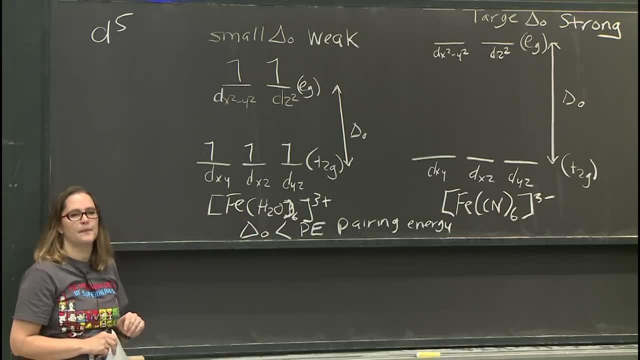 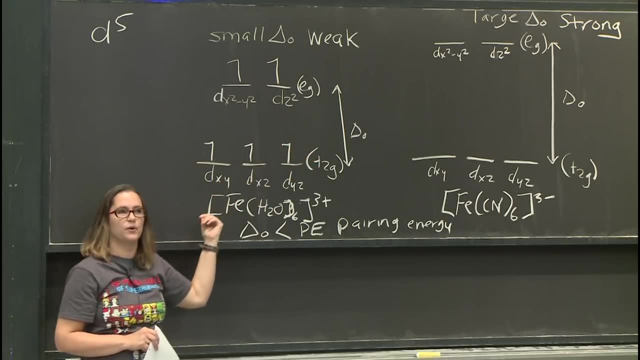 before you pair. So that's what happens with a weak field, And we also can think about how we're putting in our electrons parallel. We're not putting them in all sorts of different directions. And if we do pair, we're going to pair. so one's up. 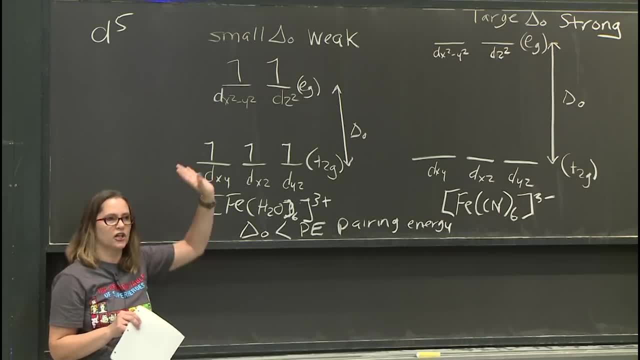 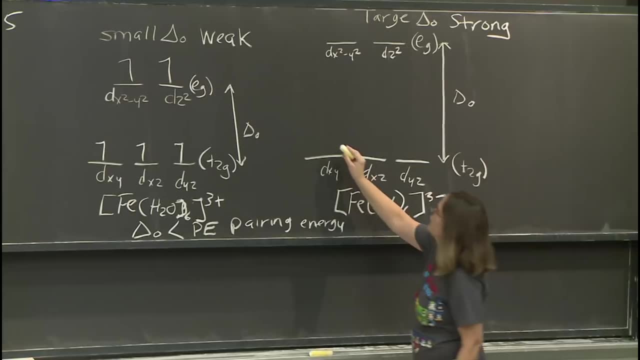 one's down. So all the rules that we learned earlier are going to apply here. So this is good review. So now, in this case, we can put in our first three electrons. And what do you think? Do you think I'm going to pair, or do you? 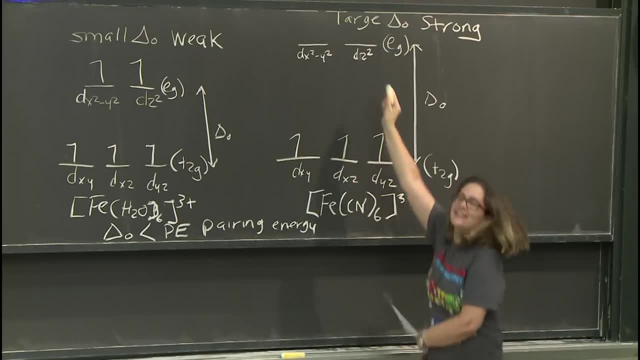 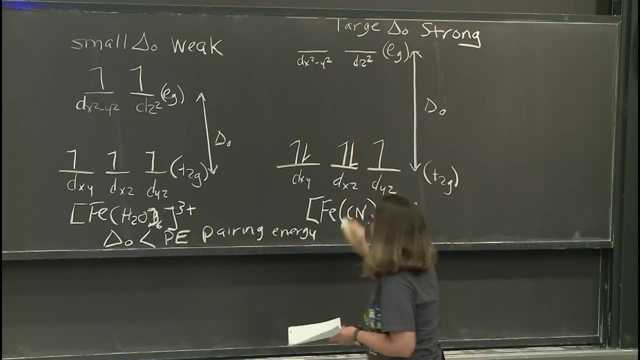 think I'm going to go up there. What do you think I'm going to pair? Yeah, I'm definitely going to pair, So I'm going to put my other two over here. So, in this case, the pair, the electrons. 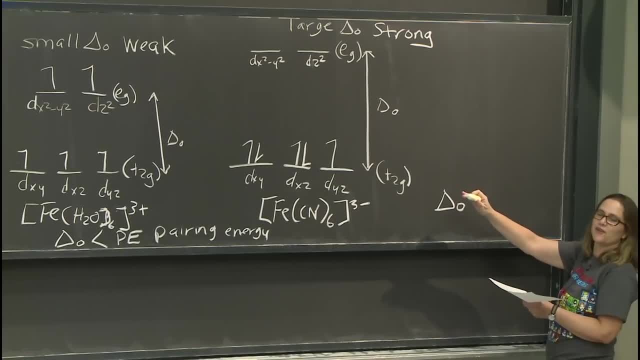 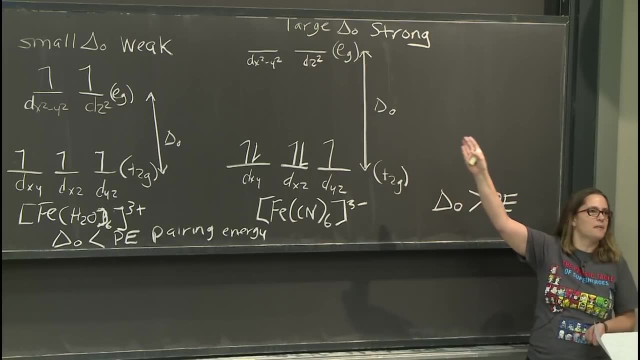 and the octahedral crystal field splitting energy- it's so much fun to say that so many times is greater than the pairing energy, And so in this case there might be empty seats, but maybe it's a long train And you could sit in car one with someone else. 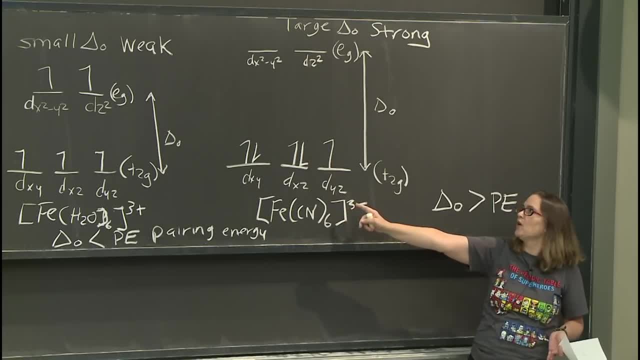 or carry all your luggage. And why did you bring so much? You're just going home for Thanksgiving. All the way, 23 cars later, to an empty seat in the back. You're just not going to do it. You don't have enough energy. 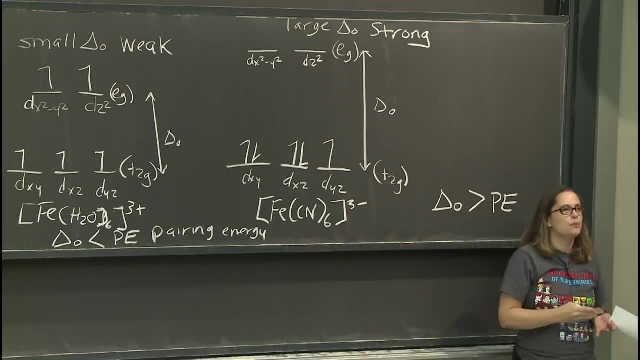 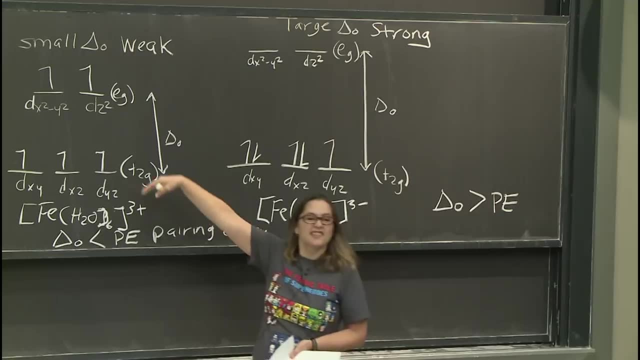 You'd rather sit with somebody up there. You'd rather sit with somebody up front. So how you put in electrons depends if it's a weak field or strong field. It depends on whether it takes just a little bit of energy and it's worse to pair, or it takes a huge amount of energy. 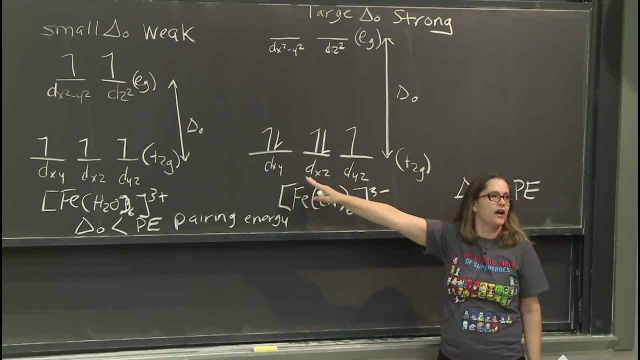 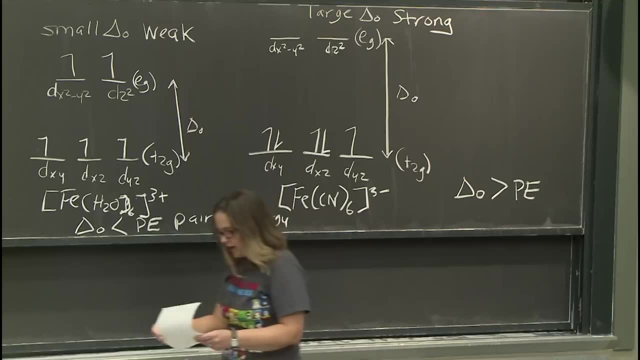 There's a big splitting, a really strong field, And in that case you're going to pair first And you're only going to put electrons up here when you're completely done here. All right, So now we have placed our electrons. 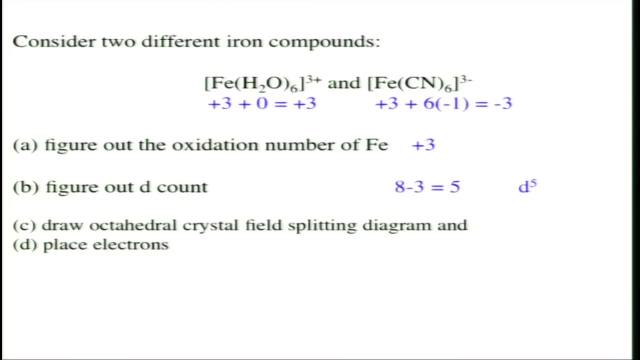 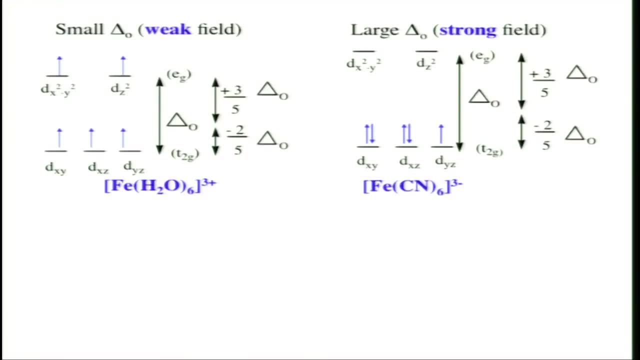 We've talked about pairing energy, And we've talked about the weak and strong fields, And now we can talk about some notation, because there's always notation. So this is what we've done already, And now we're going to do step E. 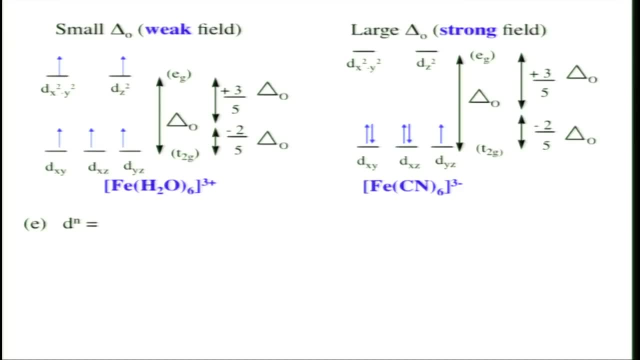 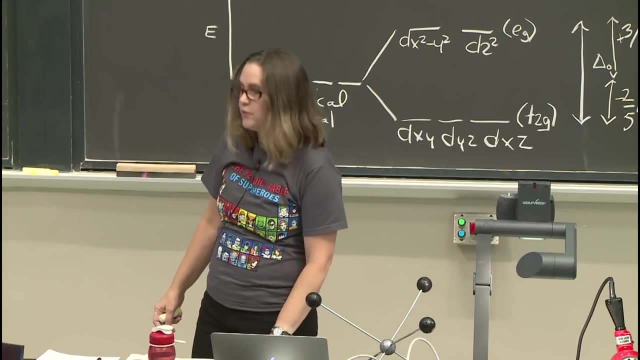 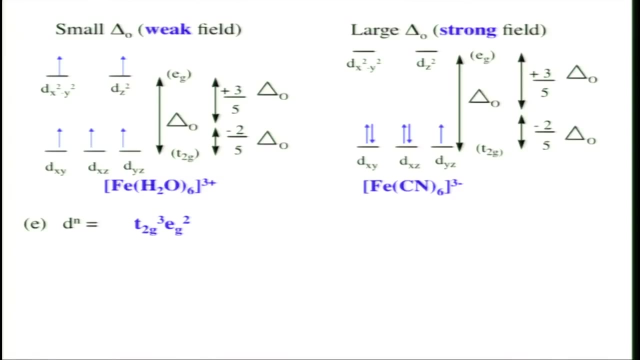 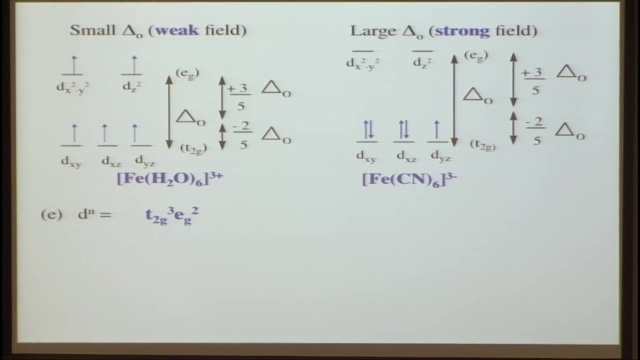 which is to our d, to the n electron configurations. Every diagram. there's different configurations every time. So this one we do using those little kind of cool terms I told you about. So, instead of writing, I have one electron in dxy, one electron in dxz and one electron in dyz. 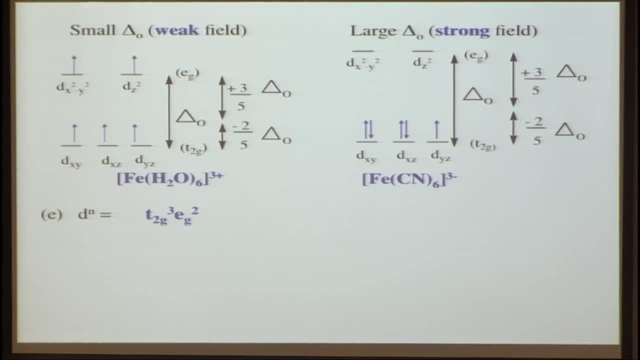 I can just say I have three in the t2g set of orbitals, So that is a lot more convenient. So you would just say t2g3. And I have two up here, so eg2.. And that's how you would do this. 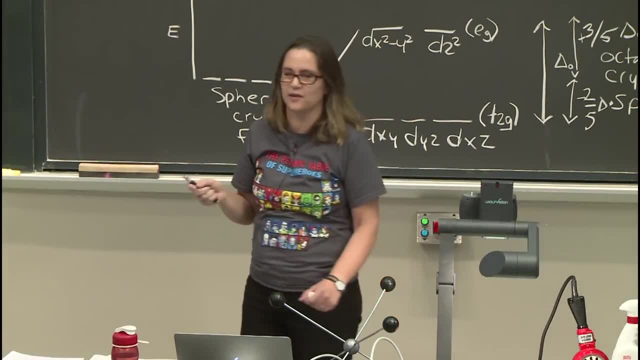 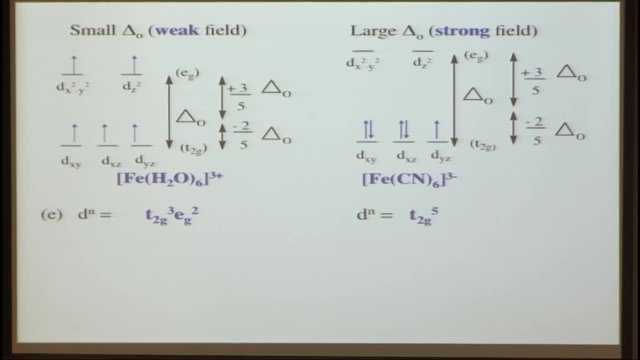 I think this is our last configuration for electrons in a diagram that you're going to be learning. There's a lot of them, OK, So then over here we would just say: we have five all in the lower energy set, all in our t2g. 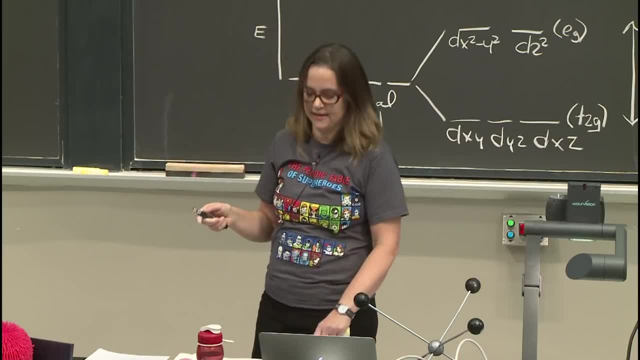 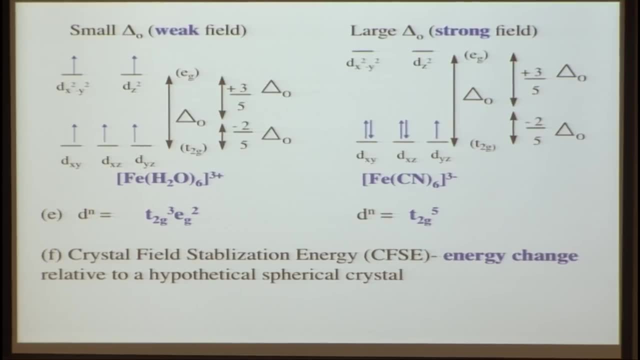 All right. One other thing, part f, that you can be asked about, which is the crystal field stabilization energy, not to be confused with the crystal field splitting energy. They both start with an s, So I don't know why you wouldn't be confused by that. 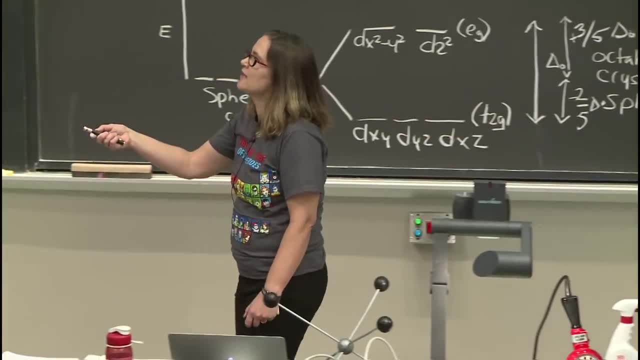 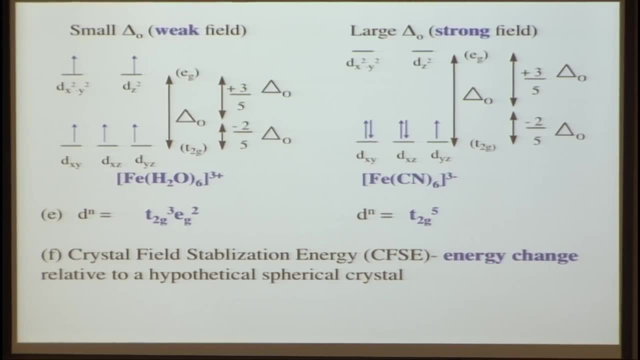 But if you can try to remember it, that would be awesome. It's often abbreviated cfse, And this is the energy change that's due to going from this hypothetical spherical crystal field where all the d orbitals have the same energy, And if you put your electrons in here, 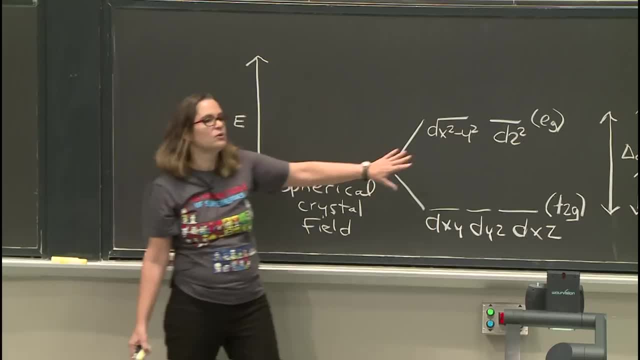 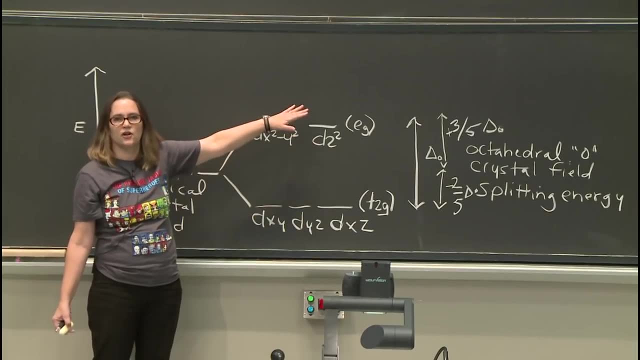 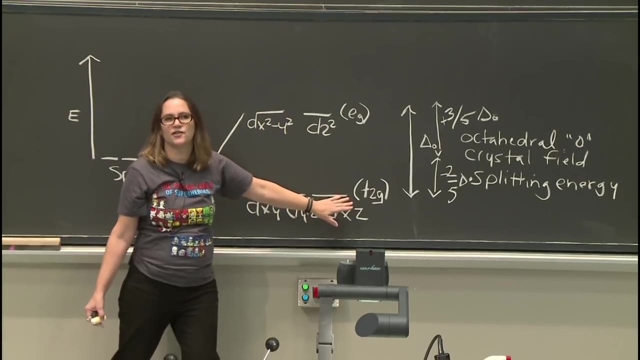 where they'd all have the same energy. you'd have the same energy to the energy difference when you're placing the electrons in lower energy orbitals or higher energy orbitals. So you're thinking about how much more stabilized is the system if all of the electrons are down here. 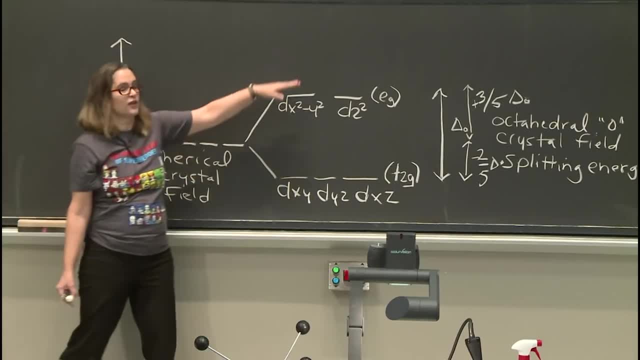 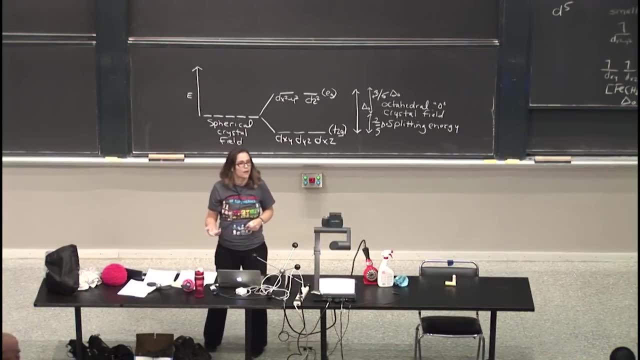 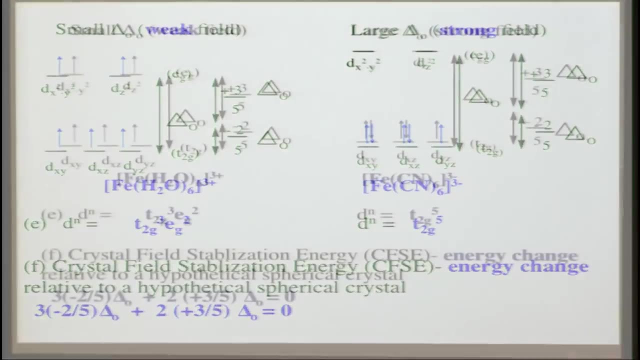 That's going to be stabilized compared to where they were here, But if a lot of them are up here, then there would be less stabilization due to this splitting. All right, So let's look at how we would write that. So we have three electrons that are down in energy. 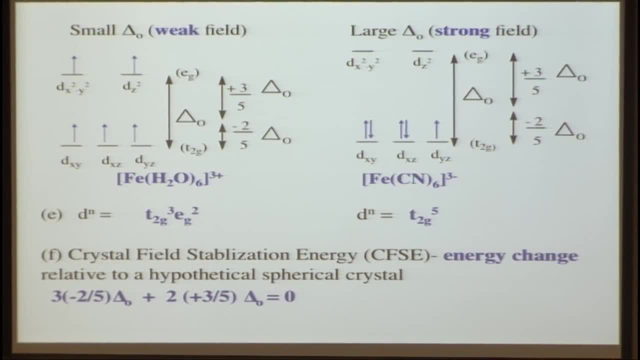 And they are down in energy by minus 2, fifths times the octahedral crystal field splitting energy, And that's because the overall energy is maintained. Three go down in energy, so that's minus 2.. Two go up in energy, again plus 3.. 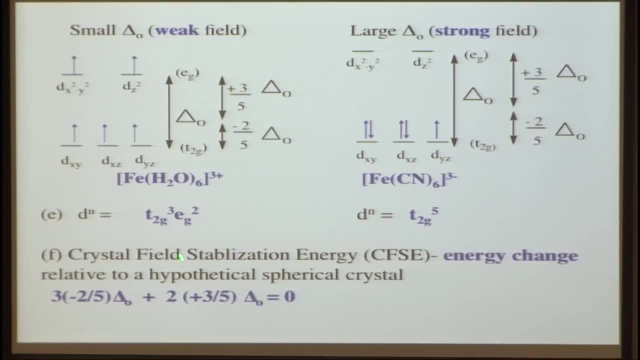 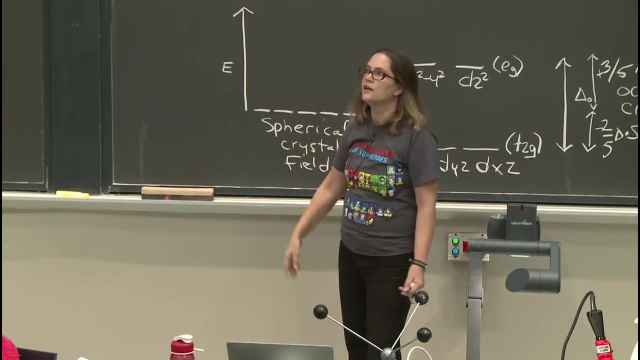 And then we have two electrons up here, so 2 times plus 3 fifths, again times the octahedral crystal field splitting energy, And so overall our stabilization is 0. There's no stabilization of this system compared to the system here, because three electrons 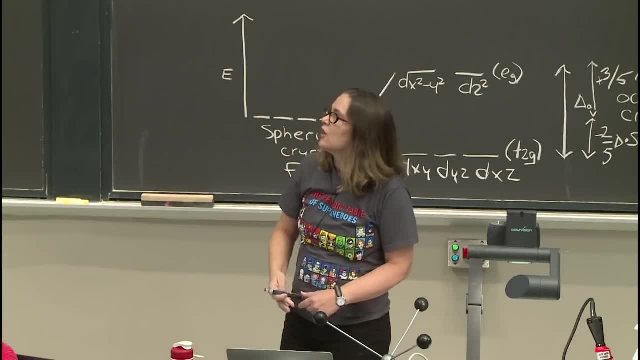 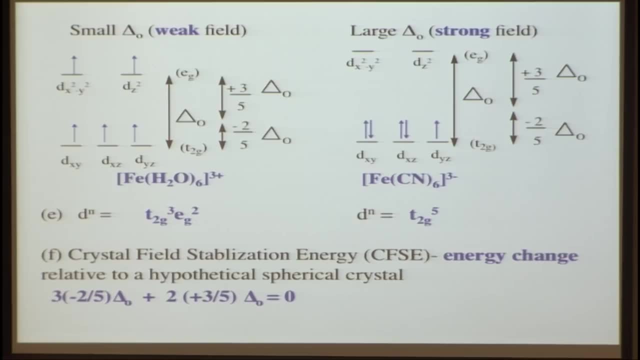 are down in energy and two are up, All right. So now you might imagine that this is going to have some extra stabilization, And you would be right. So we would write this like this: We'd say there are five electrons down, stabilized in the lower energy orbitals. 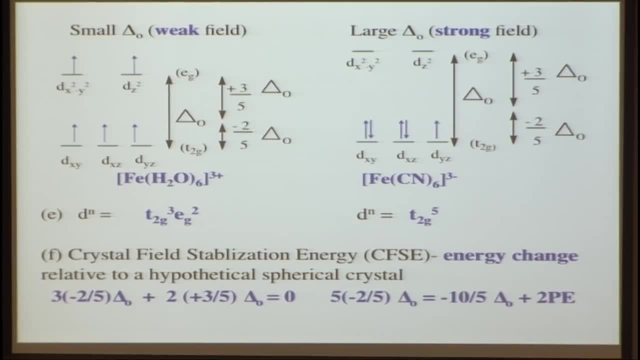 So 5 times minus 2 fifths times the octahedral crystal field splitting energy minus 10 fifths times the octahedral crystal field splitting energy. And sometimes you'll also see kind of a little truth that there's also some energy kind of due to this pairing. 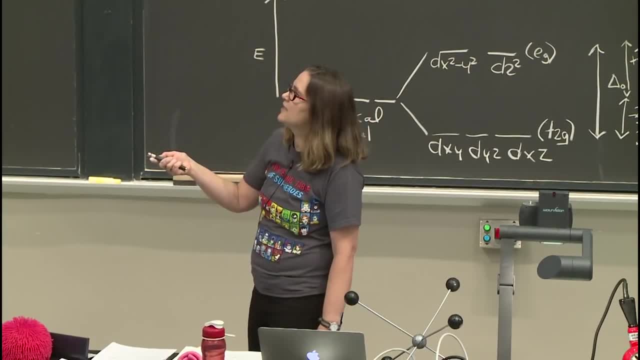 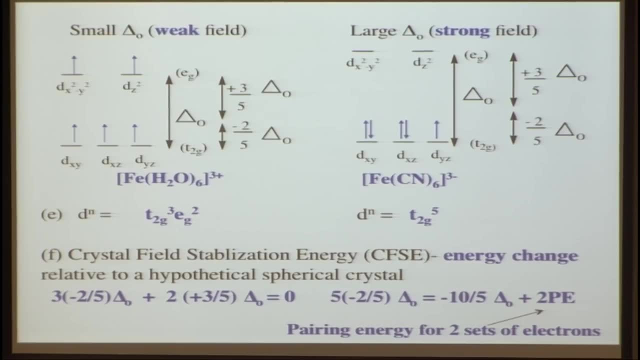 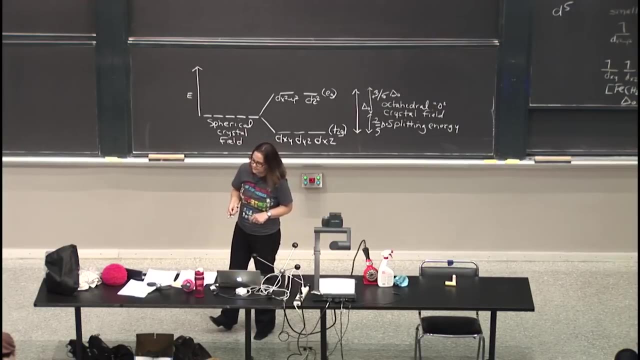 So you might see an indication that there's pairing energy for two sets of electrons. So sometimes that's included, Sometimes it's not. The questions will ask to indicate how many kind of sets of electrons ended up being paired for that stabilization. All right, 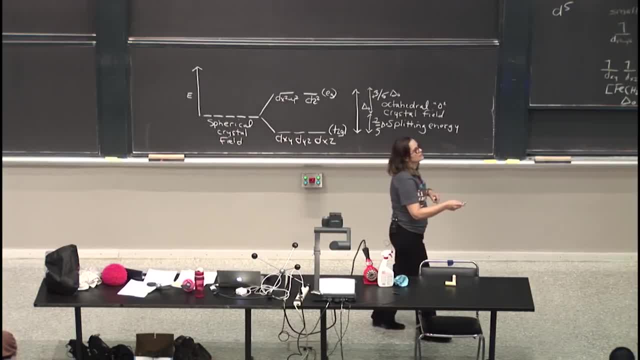 So we can think about again. we have this nomenclature here And we can think about the stabilization. So there's a big difference between these iron compounds. One, there's no stabilization due to the splitting, And the other one there's quite a bit. 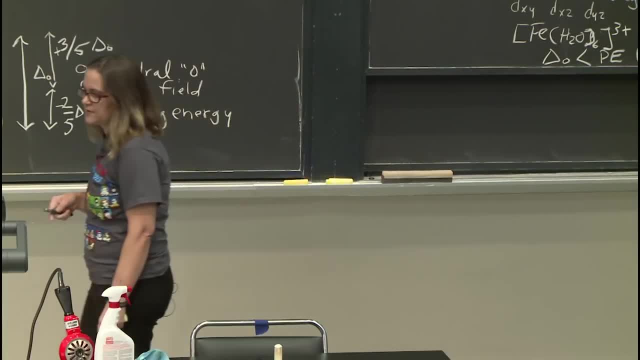 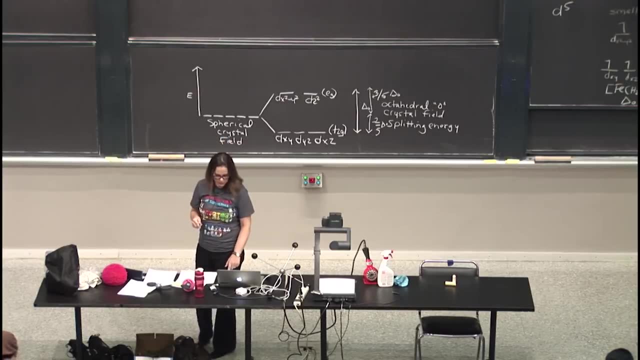 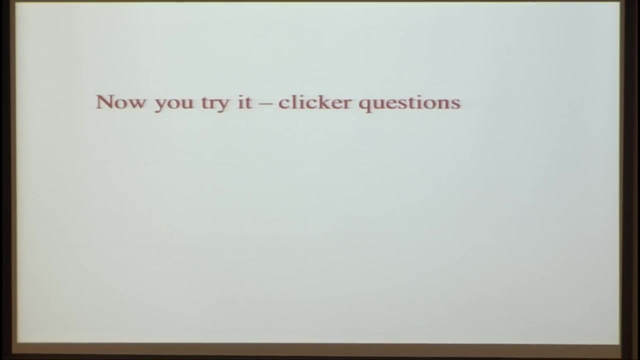 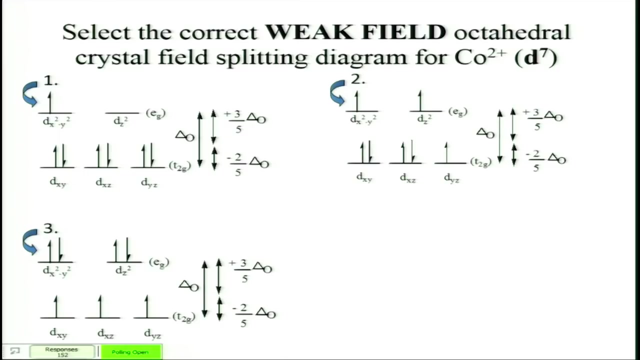 because all the electrons ended down in the lower energy orbitals. So now it's time to try some of the things on your own. See if you got the rules down And let's try some clicker questions. Clicker question one: OK, 10 more seconds. 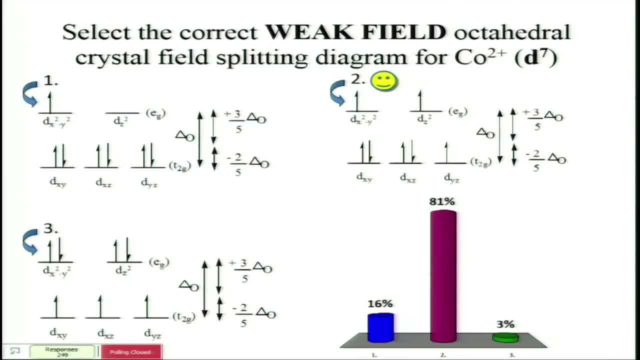 Yeah, All right. Yes, So the trick here is to remind yourself what weak field meant, And in this case, if it's a weak field, that meant that you place all the electrons singly- there's seven of them- to the fullest extent possible. 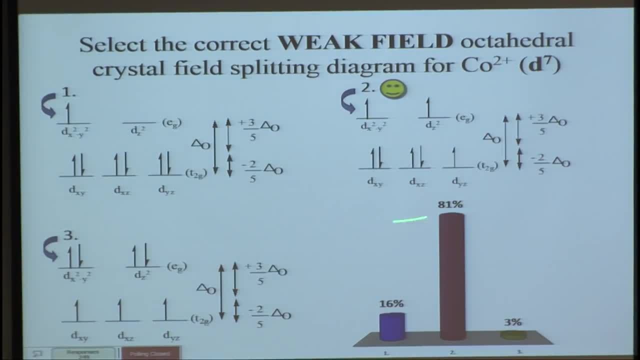 before you pair. You still have to pair, But here you put more. You fill these up before you paired And this is a strong field diagram where you paired all of them possible before you put any of them up here, And to make it harder, I drew them the same. 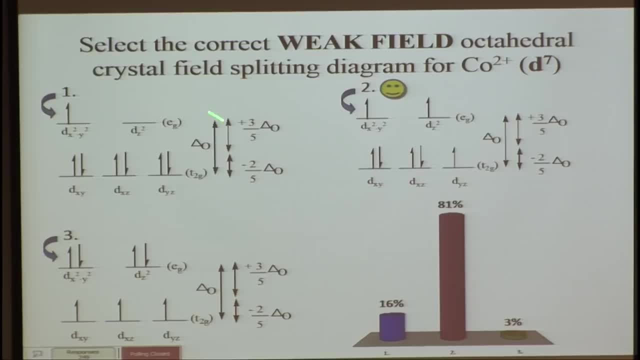 So you have to really pay attention to what weak field meant. But this would be the version of the strong field And this is just wrong. So you wouldn't have more electrons up in the higher energy orbitals for really any reason whatsoever. OK, 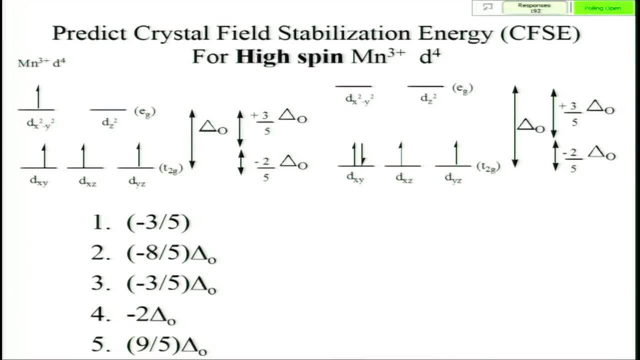 So let's try the next one. All right, Let's just take 10 more seconds And we'll mention high spin And we'll do this problem. Yeah, People did very well with that. OK, So I forgot to mention that. 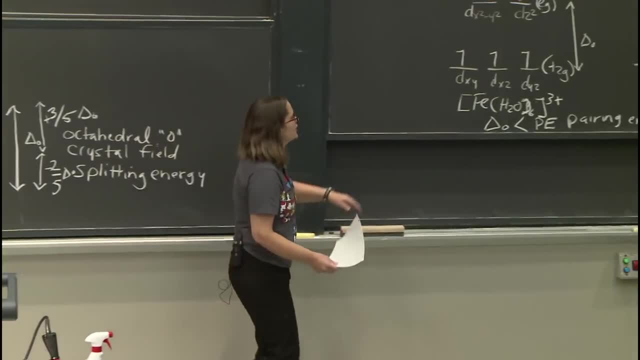 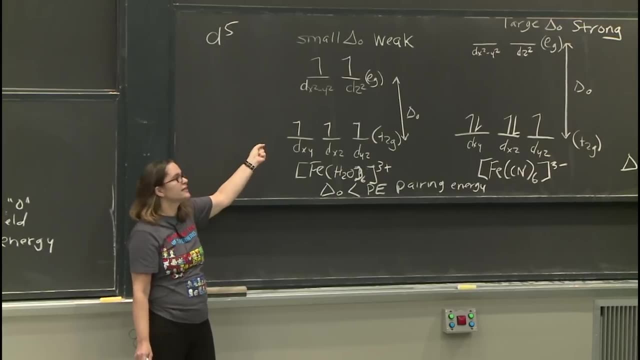 I ran out of room to draw So I decided that was enough. So it's in your notes, though, for here And when you have a very strong field, very small weak field and you end up putting all the electrons in singly. 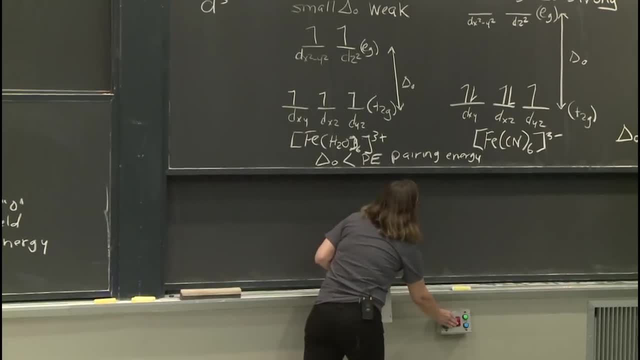 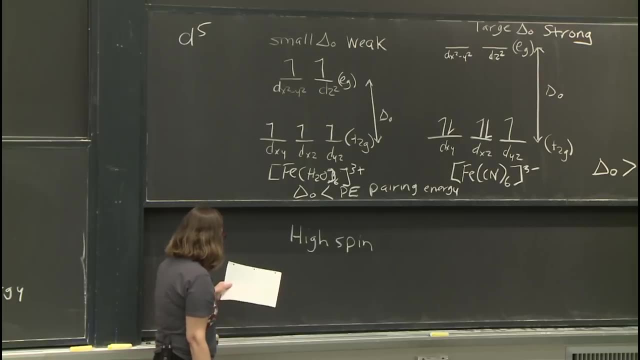 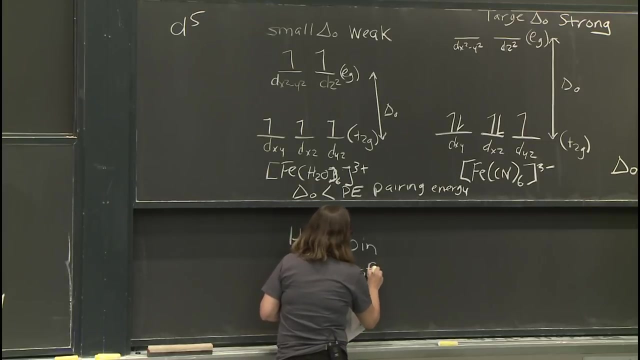 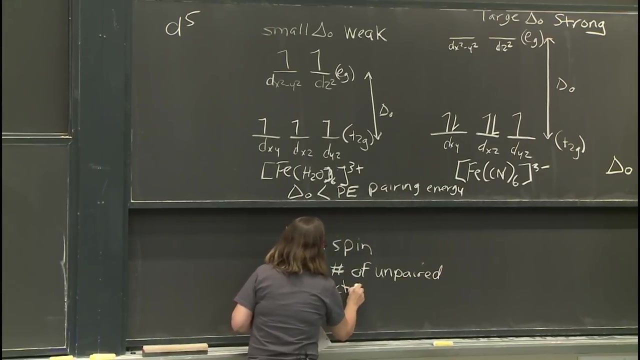 that is also known- and I'll move this up a little bit- as a high spin, And so you have a lot of unpaired electrons in this case. So that is the maximum number of unpaired electrons And it's easy to remember because you have these spins. 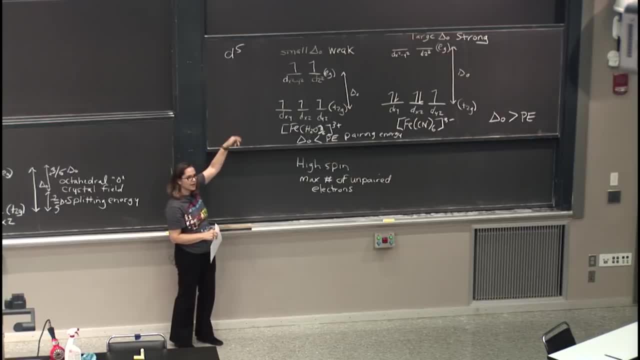 There's a lot of spins, There are a lot of single spins And they're also high up. And this is a low spin case, when you have a strong field, because you like to pair first before putting them singly. So this is going to give you the minimum number. 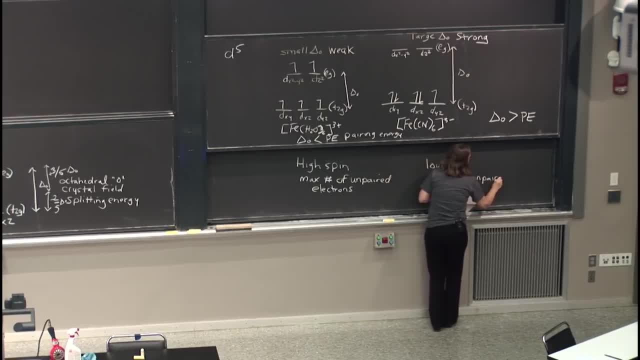 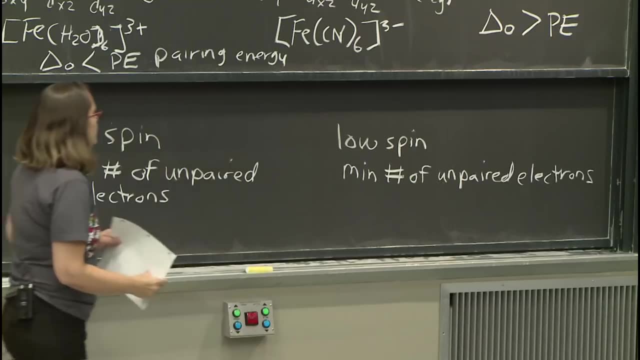 of unpaired electrons. So high spin, weak field. low spin often comes from a strong field, So it's about whether you have maximum number of unpaired electrons, which you do with a weak field. high spin, minimum number- All right. 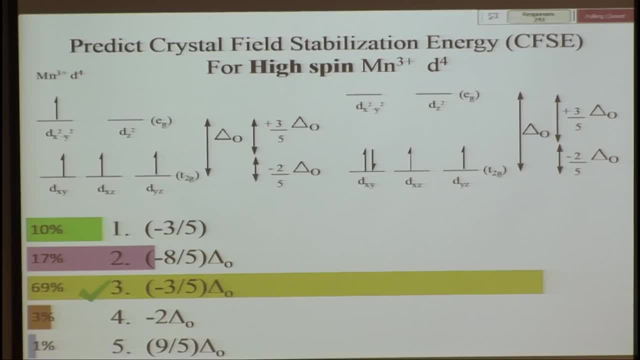 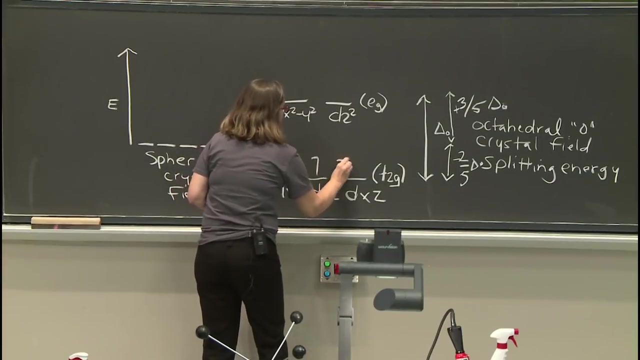 So let's look at this one then. So it's a high field one, So that means that you're going to have the maximum number of unpaired electrons. So this would be, So this would be our diagram here, And I can put that over here. 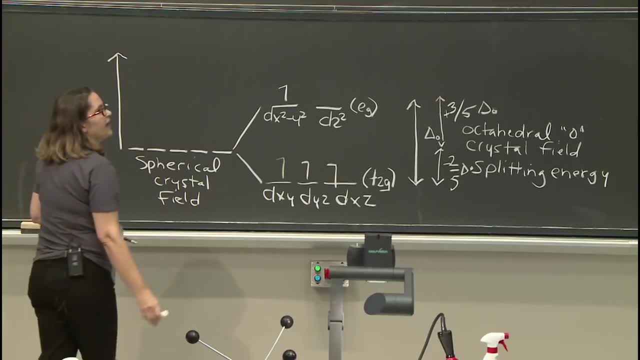 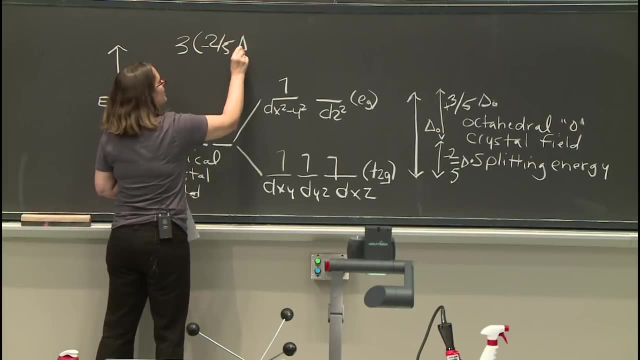 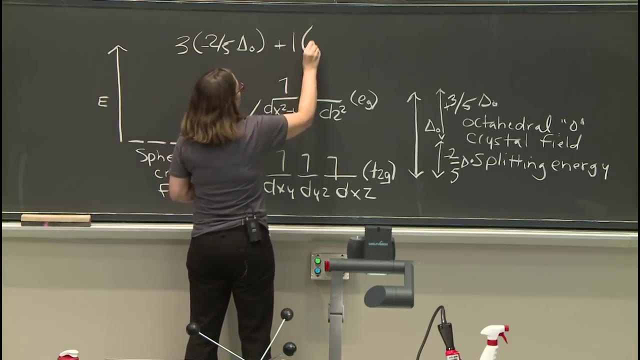 And so then you have to figure out how to write that, And so you would have three ones down in energy, minus 2 fifths times the octahedral crystal field splitting energy, And you would have one electron up by 3 fifths times the octahedral crystal. 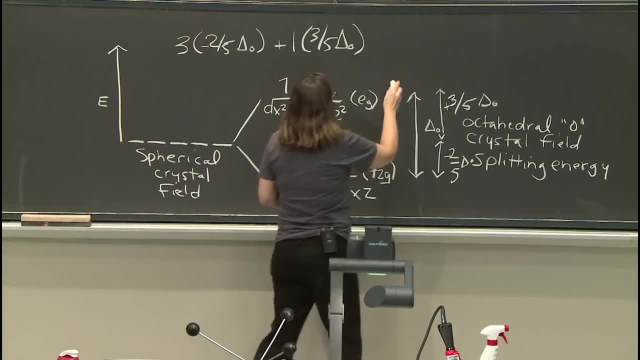 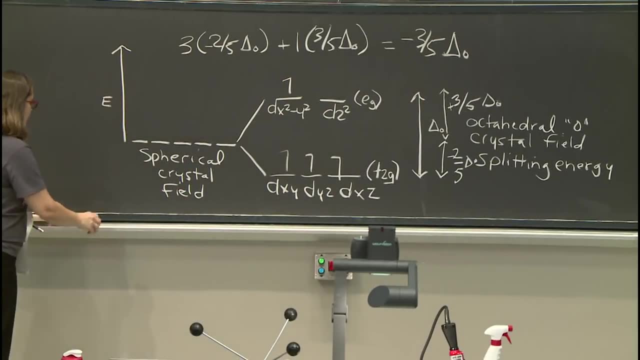 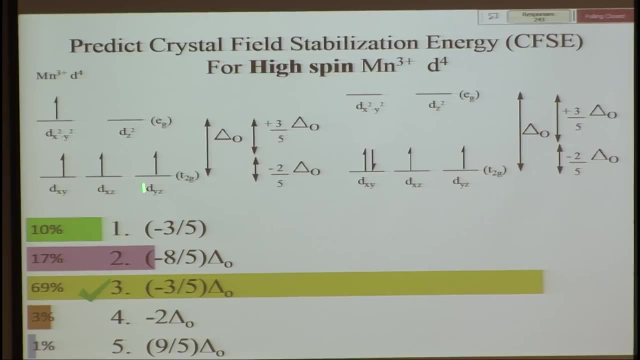 field splitting energy. So minus 6 plus 3 is minus 3, fifths times the octahedral crystal field splitting energy. So this problem required you to know what high spin was, then correctly identify the weak field diagram and then figure out the crystal field stabilization energy. 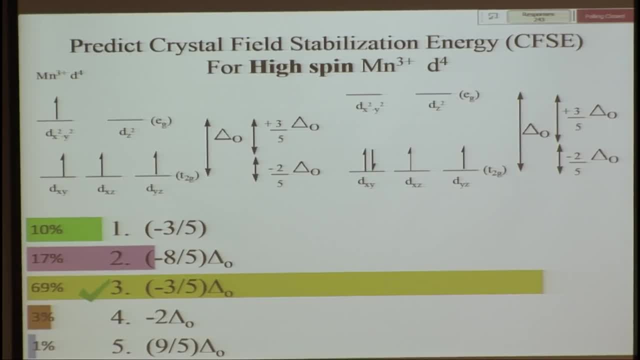 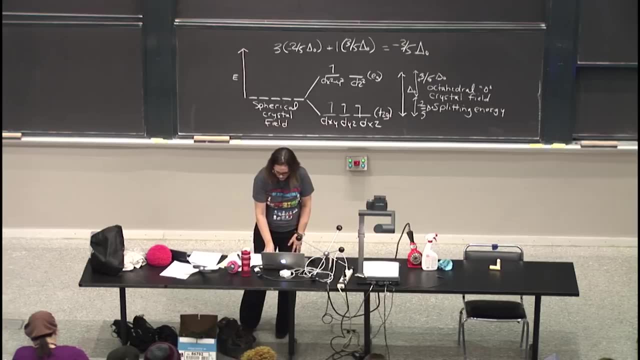 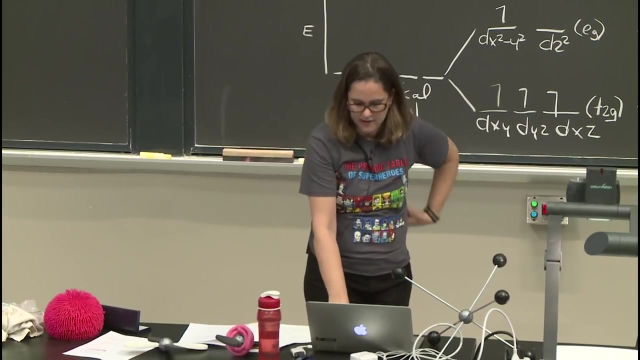 So that was actually quite good, And maybe you'll remember the high spin, low spin definitions as well. So let's just do one more thing And then we'll, because we've just been talking about high spin. So back to our compounds. 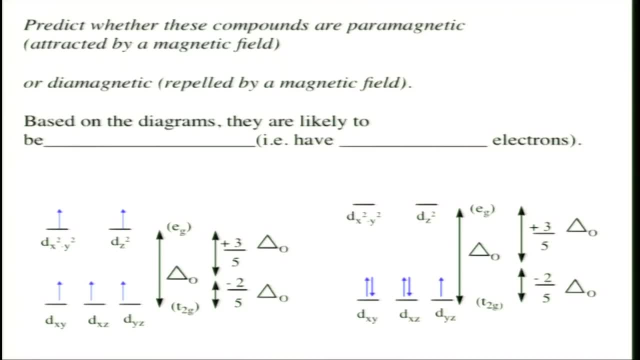 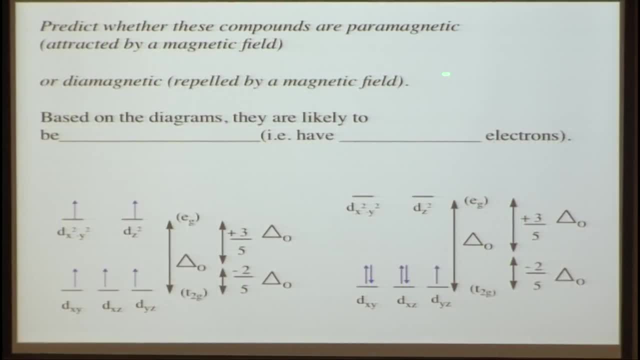 We're going to talk about magnetism And then we're going to come back next time and talk about color, And we have some cool demos for color which we'll do next time. But before we leave from this, our iron compounds. 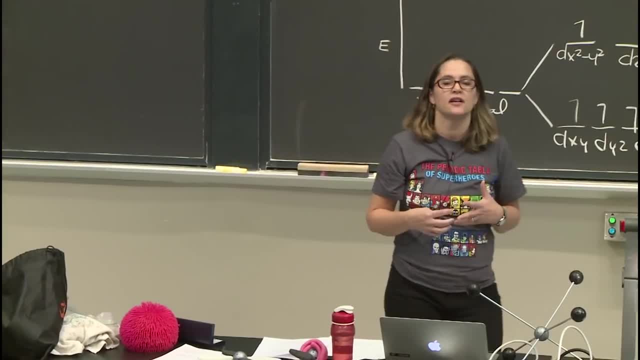 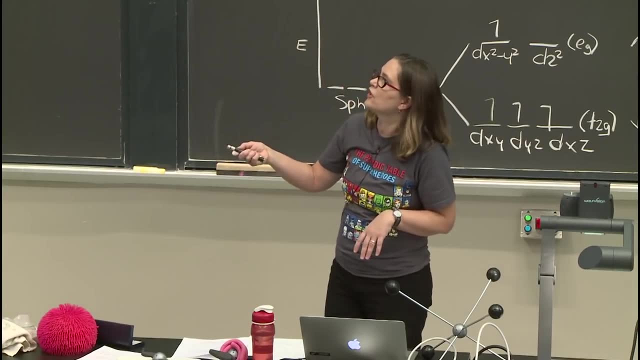 we want to think about whether they're paramagnetic, which is attracted by a magnetic field, or diamagnetic, repelled by a magnetic field, And we've already talked about this in this class So based, and here are our iron diagrams again. 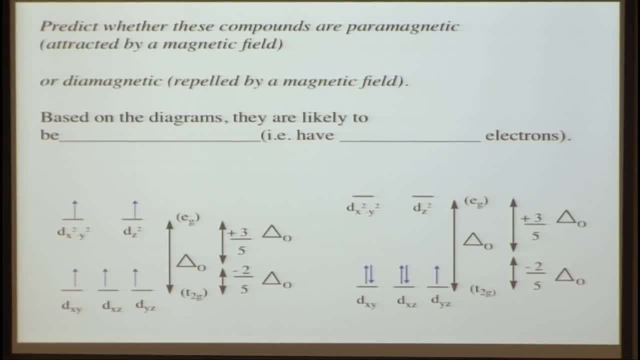 Based on these diagrams, would you expect these to be paramagnetic or diamagnetic? Paramagnetic, And that was because it has what kind of electrons? Unpaired, Unpaired, right. So here you just have to remember your definition of paramagnetic. It has unpaired electrons. Now, normally things with a weak field and are high spin are going to be more likely to be paramagnetic, have unpaired electrons, Things that have a very strong field, and so you pair first before you fill up. 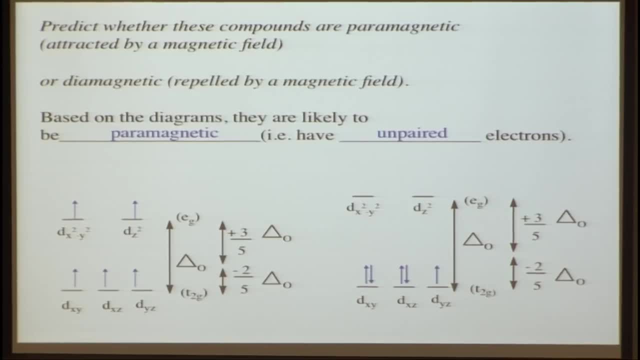 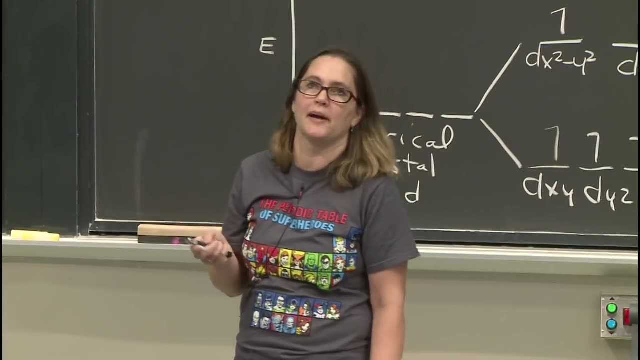 minimum number. low spin minimum number of unpaired electrons are more likely to be diamagnetic, But in this case we didn't have enough electrons, so they're still both paramagnetic, All right. so we'll stop there And we'll come back and talk about the colors. 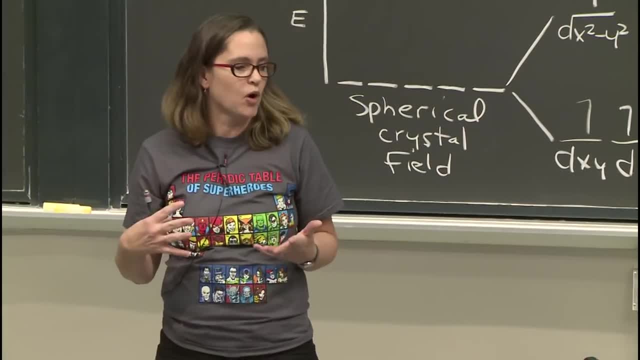 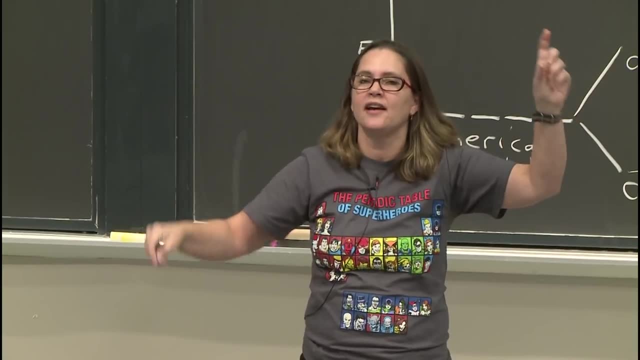 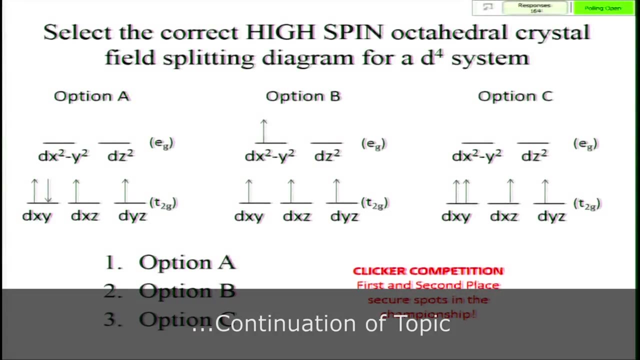 of those iron compounds and more colors and cool demos on Friday. Don't miss Friday. Remember Friday. double clicker competition: The team that comes in second is automatically in the playoffs. We're at 166,, but it stopped OK. 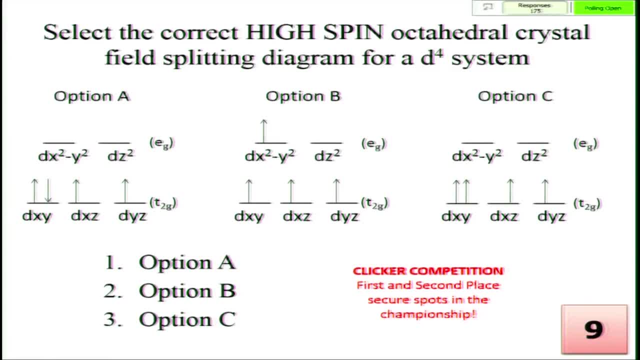 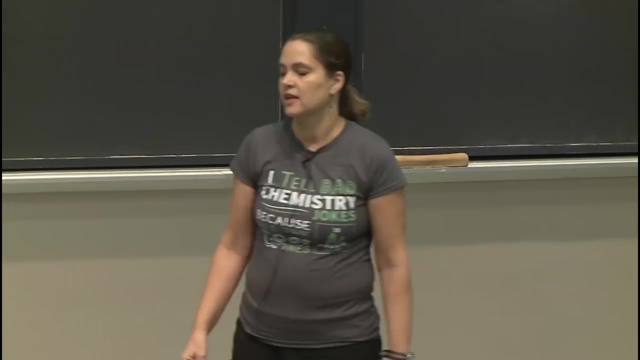 Let's just take 10 more seconds on the clicker question, All right. OK, let's quiet down. I'd like to see the 85%. That's good. Of course it doesn't distinguish all that much for the clicker competition today. 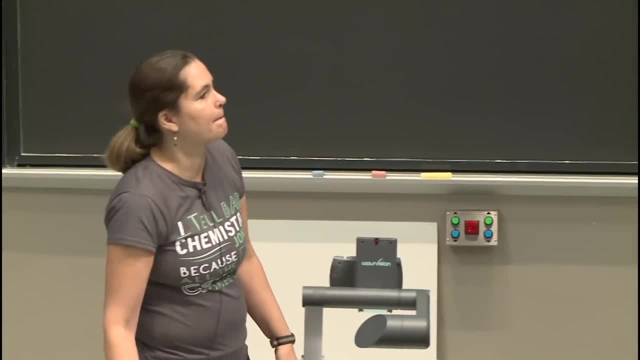 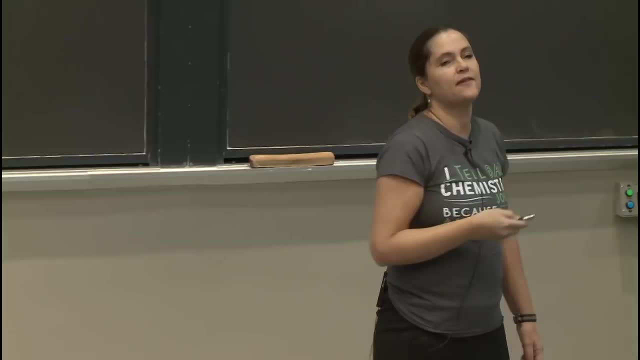 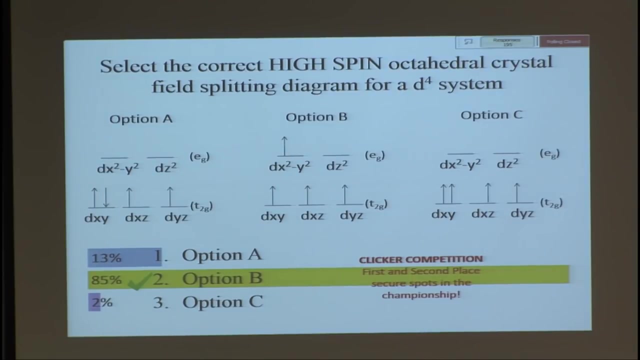 So if we can quiet down a little bit, People can just yell out. What would this have been the correct answer to? What should the question have said for that to be the correct answer? Low spin, right? So low spin is the minimum number of unpaired electrons. 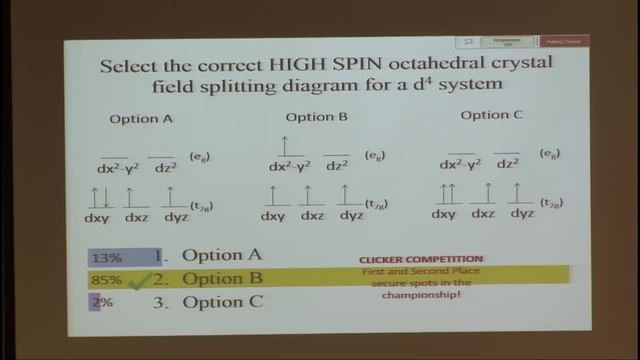 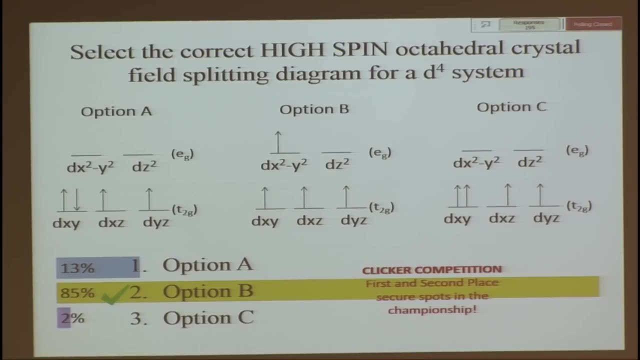 And so this is the low spin. High spin is the maximum number of unpaired electrons. So this is the correct diagram And C is wrong. It's not correct for either high or low spin, because we have two electrons here that would have the same four quantum numbers. 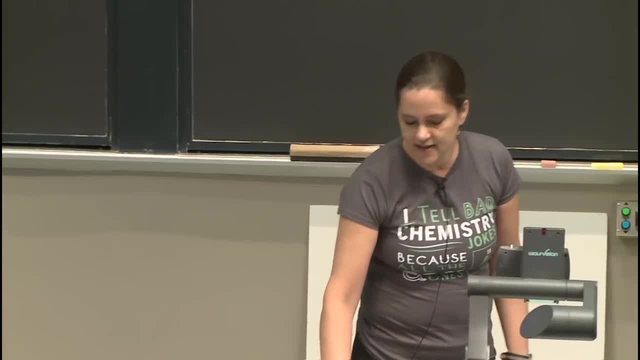 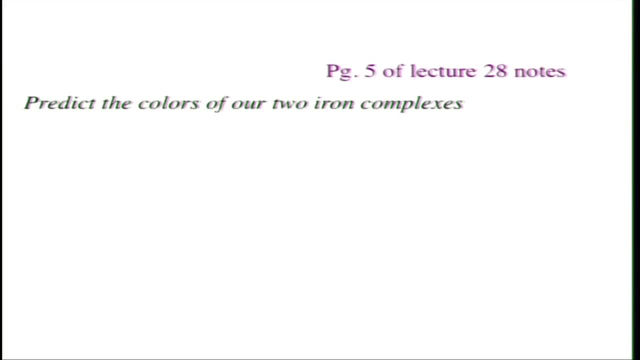 which is not allowed, OK. So let's continue on with the lecture. And we are talking about colors. So we're talking about the colors of the two iron compounds that we had described before, And so let's continue. And when we talk about colors, 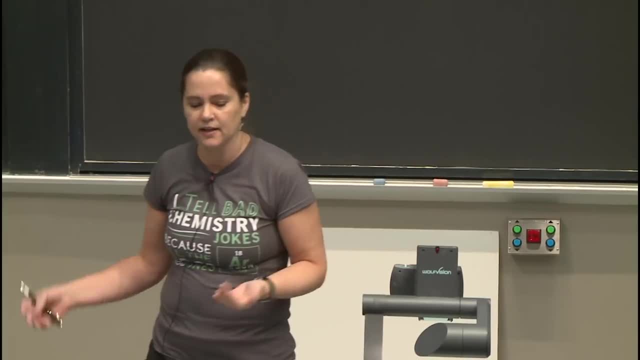 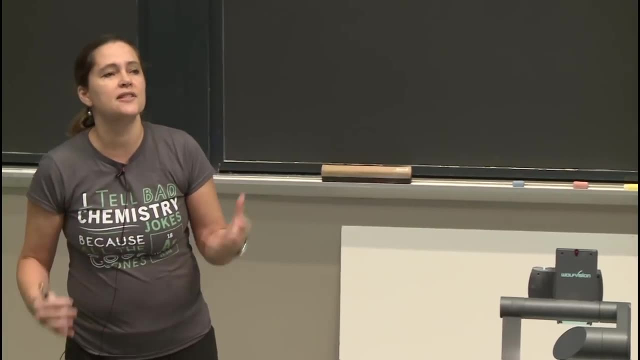 we need to do a little review and think about what's happening when a substance gives off a color, And so when a substance, whether a substance is going to absorb a photon or not, to excite an electron to a higher energy level, that then when it falls back. 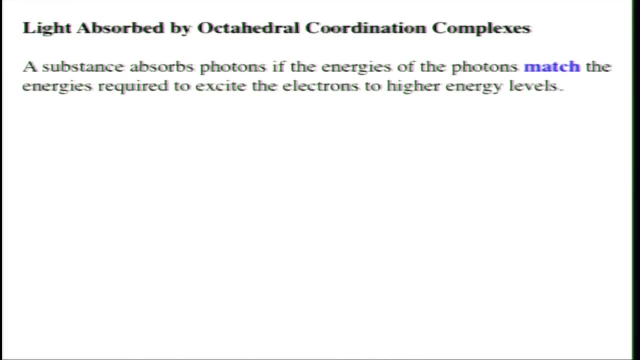 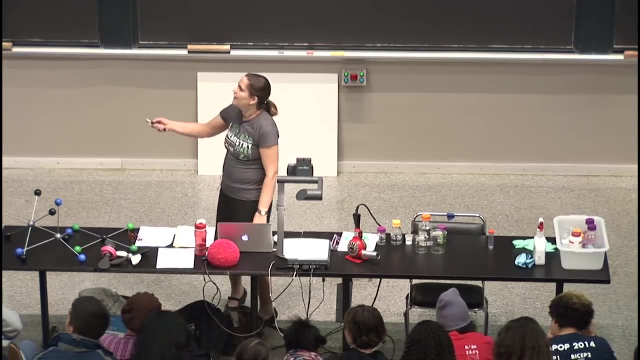 will emit a beautiful light. We can talk about whether a substance is going to absorb a photon or not, And it will if the energy of that photon is equal to the difference in that energy level. So we talked about this before exam one, exam two: somewhere around there. 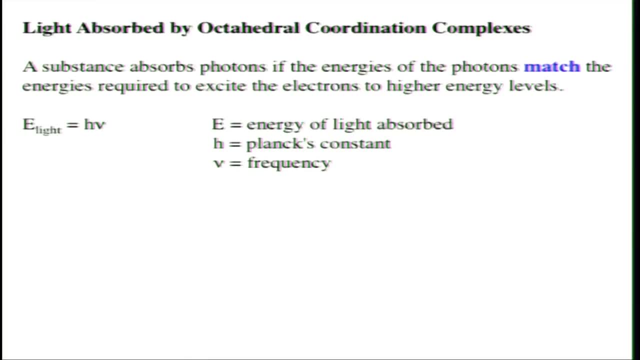 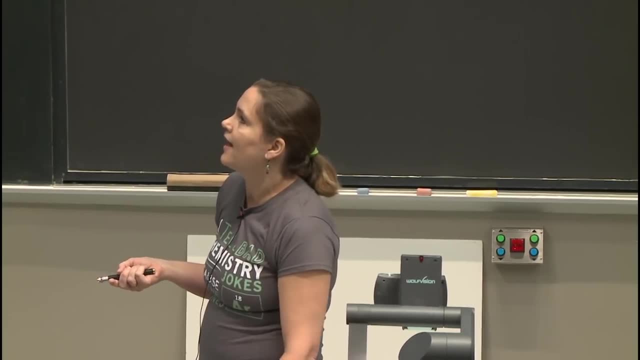 And so we saw this equation a lot, that the energy equals Planck's constant times, the frequency of the light. And now we can take that same gorgeous equation and add a little thing to it, So we can add that that energy is going to be equal to: 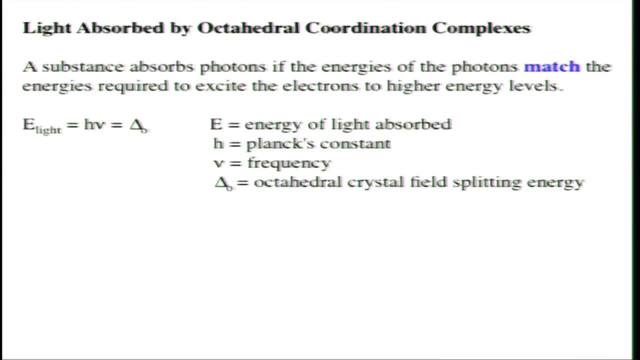 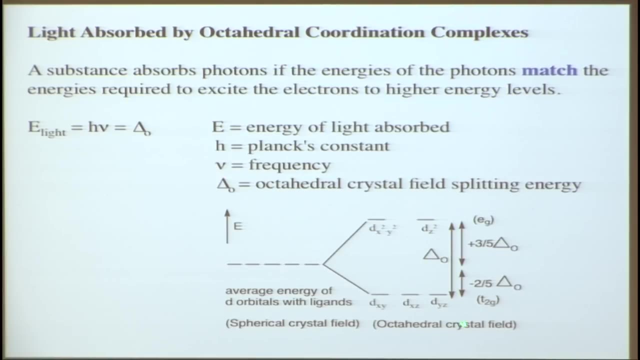 the octahedral crystal field, splitting energy, And so a substance, one of these transition metal complexes, will absorb a photon of light if the energy of that photon is equal to this splitting difference, And if it is, it can promote an electron. 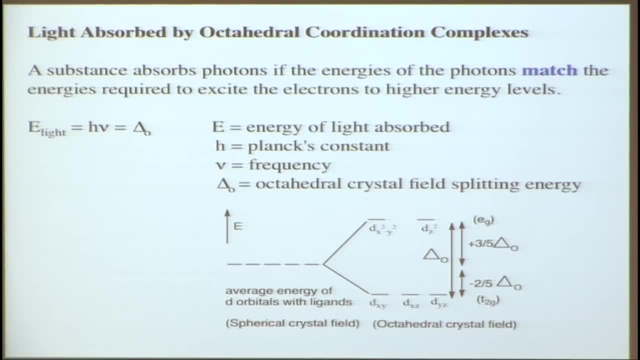 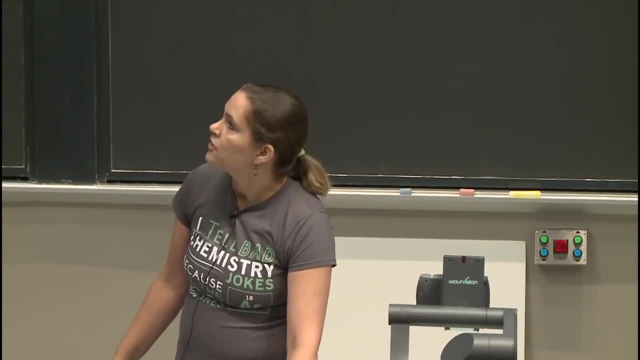 between a lower and a higher state. So this is all the same kind of thing that we talked about before, but now we're just applying it to transition metals. So let's think about what's happening with our iron complex. And if we say 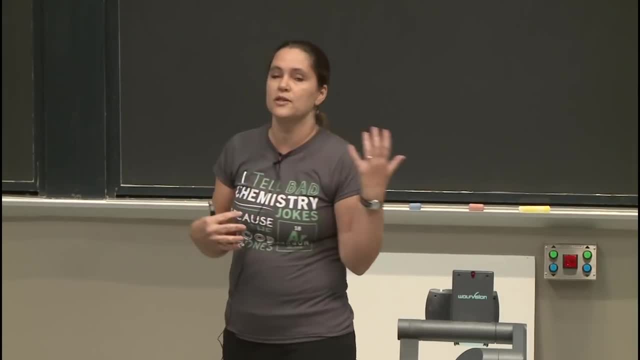 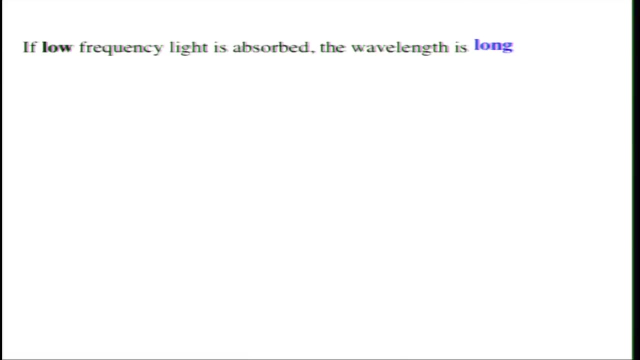 had a low frequency of light that was absorbed. what would be true about the wavelength? Would it be long or short? It would be long. And how do we know this? We know this from the fact that, if you're talking about light, 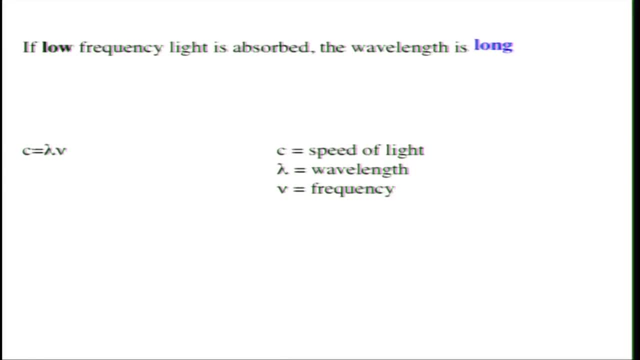 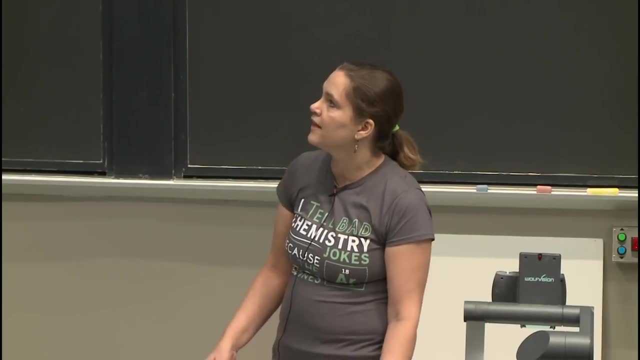 the speed of light equals the wavelength times the frequency. So if you have a low frequency then you're going to have a long wavelength. So our long wavelengths then are, in this end over here, sort of our yellow, orange, red. 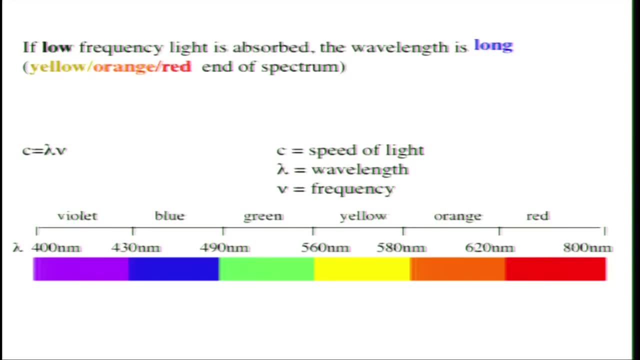 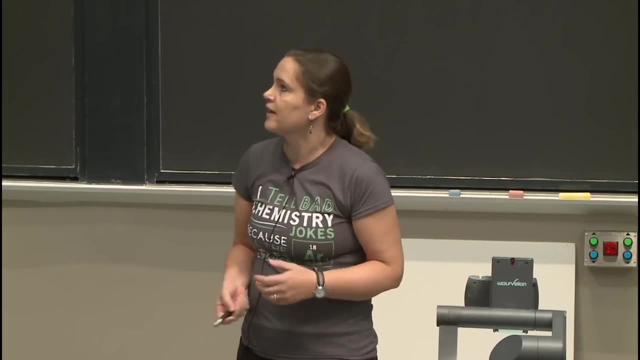 with red being our longest wavelength. So then, if we have a high frequency of light absorbed, then the wavelength would be short, so it would be short wavelength absorbed. And so, again, our short wavelengths are down here, with our shortest being the violet wavelength. 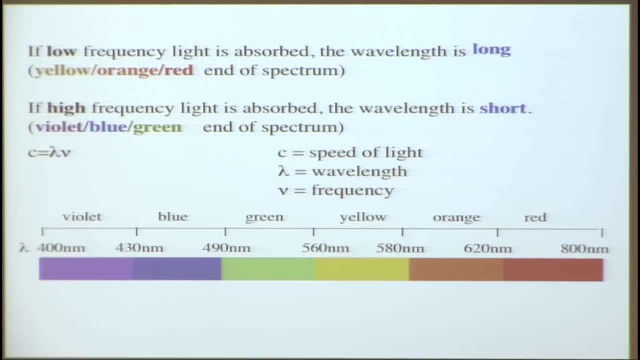 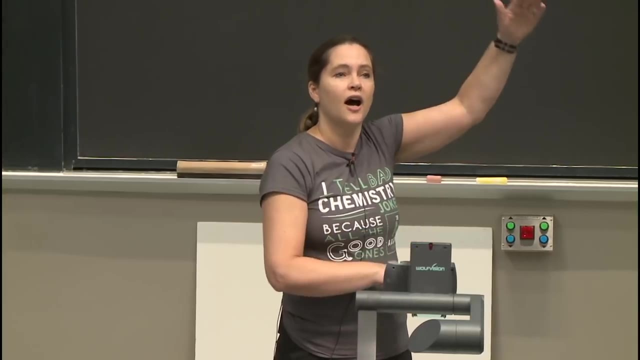 All right, and now the color that you actually see is the one that is complementary to the color, that is, of the absorbed light. So we're going to think about how big those energy differences are, whether that translates to high frequency, low frequency, long wavelength. 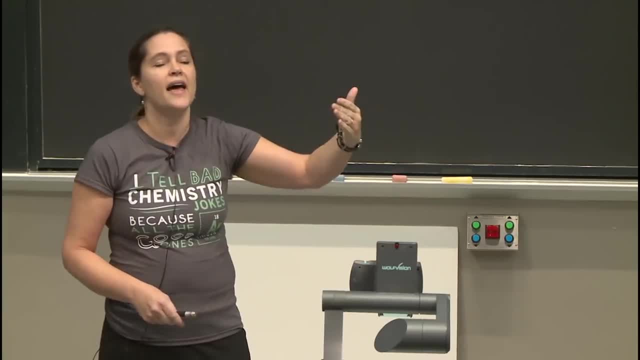 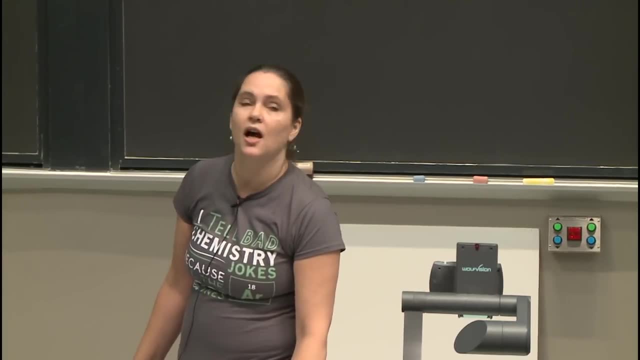 short wavelength for the absorbed light, and then the complementary of the absorbed light is the light that we see, the transmitted light. All right, so let's think about the iron complexes that we talked about, And we had a high spin or a higher spin. 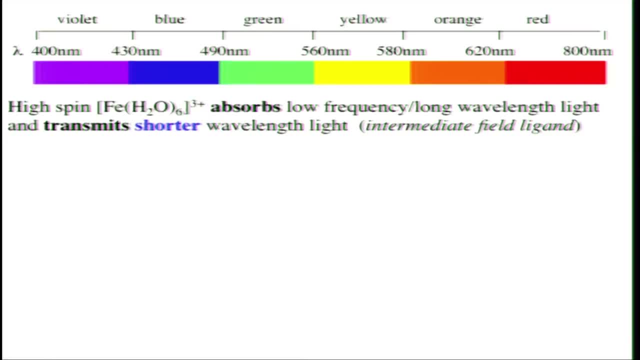 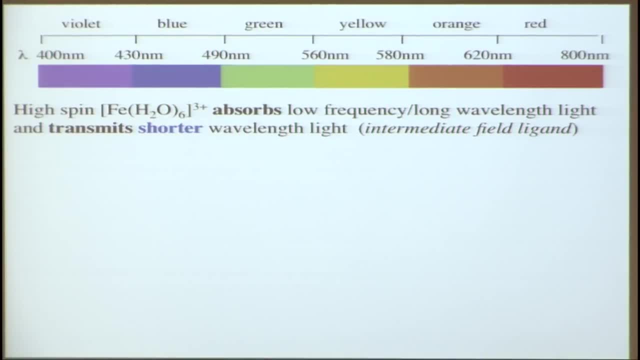 iron-water complex. Water is actually kind of an intermediate field ligand and it absorbs low frequency or a longer wavelength of light and so it's going to transmit on the shorter end of things. Again, water is sort of an intermediate field. 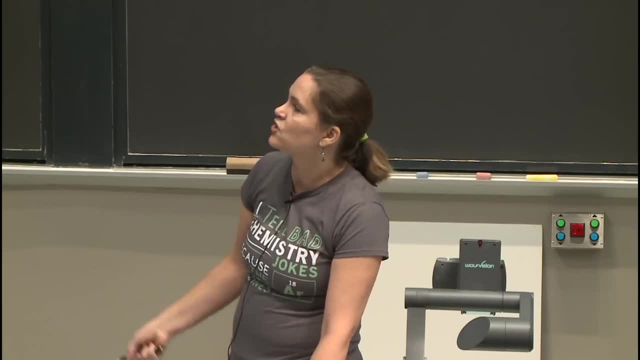 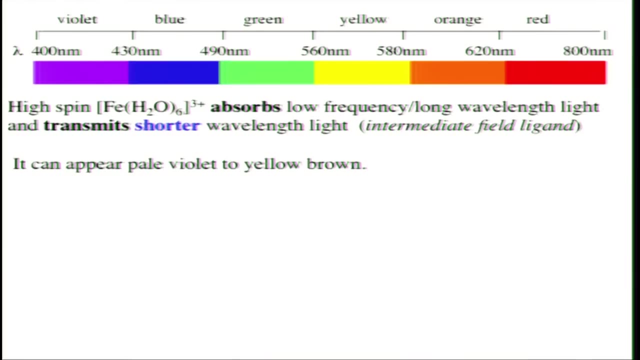 but in this case it was. it's less strong than our other one which was cyanide, which is very strong, And actually these iron-water complexes can appear actually a variety of colors. If they're solid, they're more of this pale violet. 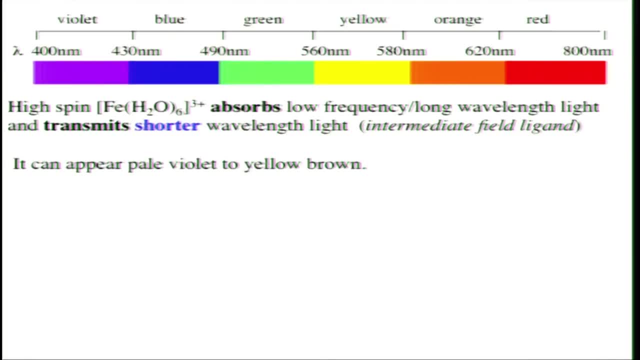 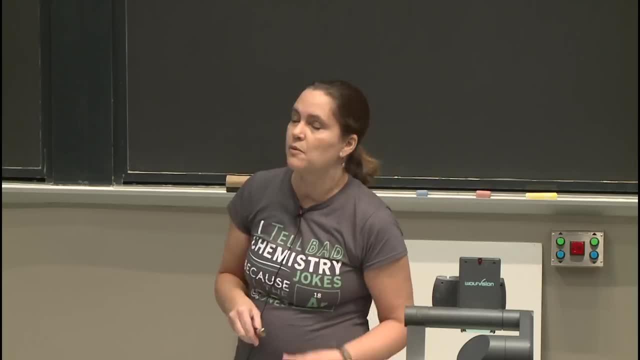 so definitely a very short color wavelength that we're seeing, But in solution and depending on the pH they can be sort of yellowish, brownish color. But the strong field ligand- remember our other compound- had cyanide on it. 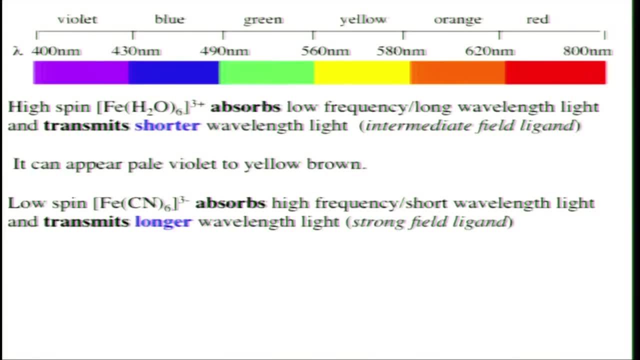 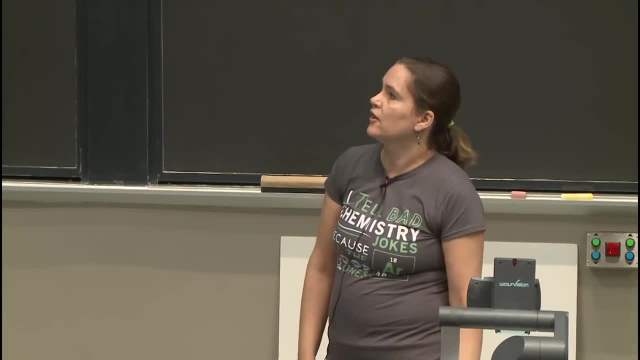 that's a very strong field ligand and so that's going to absorb then a high frequency. It's a strong field, so you have a big energy difference. So you have a big energy, high frequency and therefore short wavelength, so it'll transmit on the longer end of things. 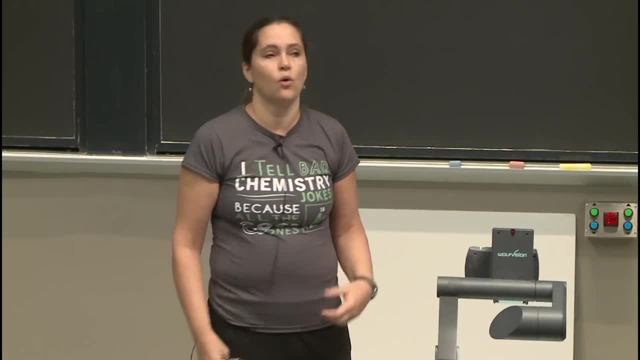 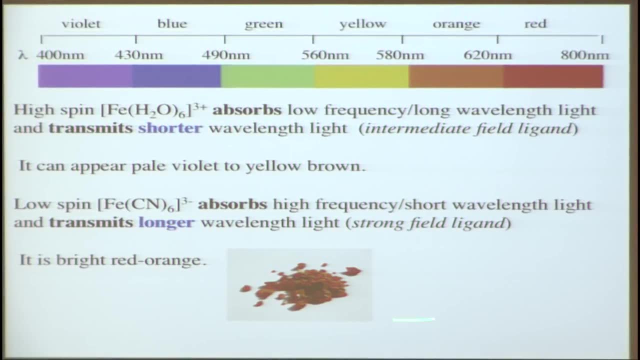 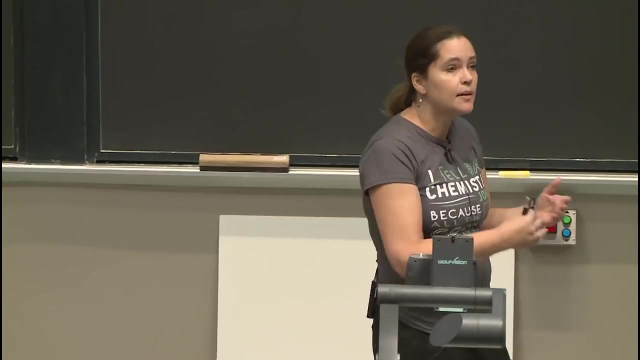 And this is actually a bright orange-red color. so you have a very long wavelength that you're observing here this beautiful red-orange. It's a really brilliant color. Now, interestingly, I mentioned, in terms of applications, that some transition metal complexes. 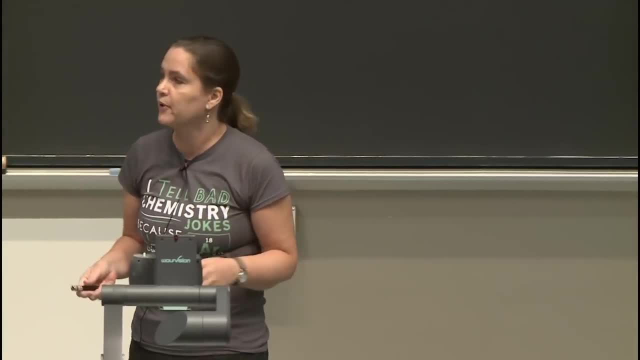 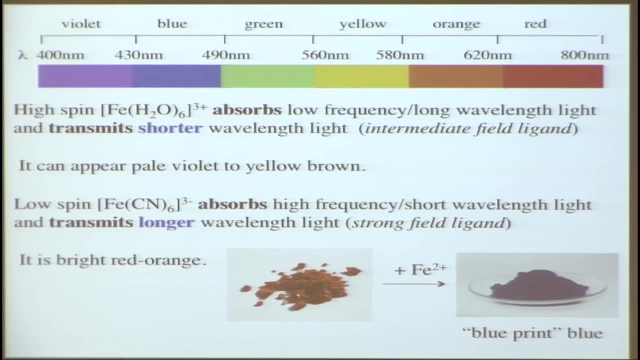 were used to color things and I mentioned the blue in blueprint. And if you take this compound and actually add iron in a different oxidation state to it to form this complex that has iron plus three and iron plus two with cyanide, you actually get the blueprint blue. 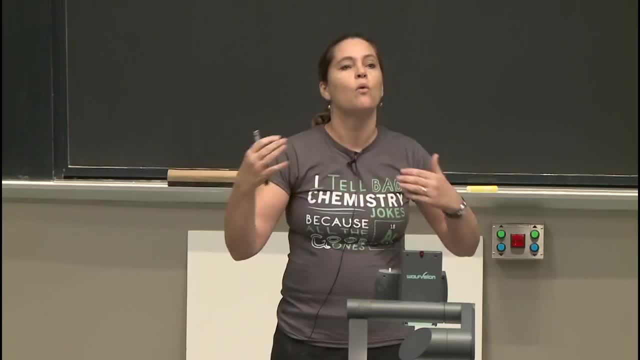 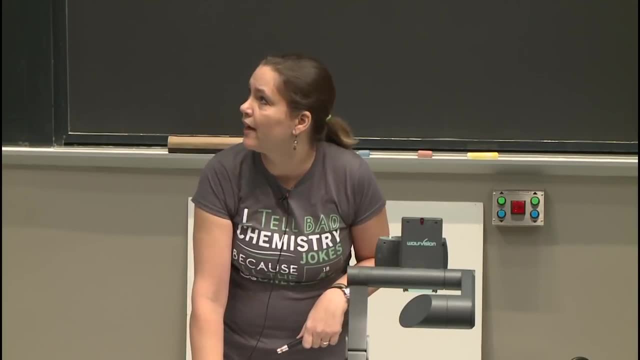 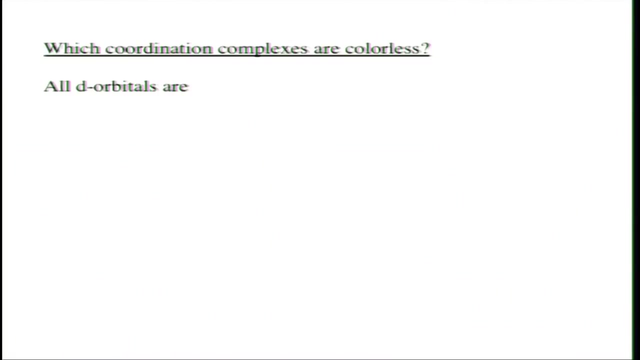 So the colors can be just dramatically different depending on what gets added to the system. All right, so now let's think about- it's a little sad, but things without color. So what coordination complexes would be colorless? What would be true about the d-orbitals? 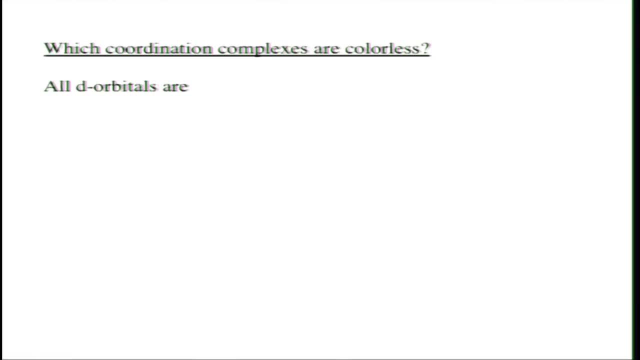 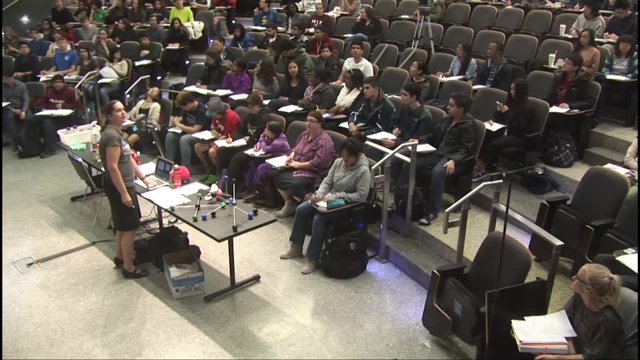 if you had a colorless thing? Yeah, what would be true? Yeah, they could all be degenerate. so there's no splitting at all, which usually doesn't happen if there are any ligands around. That's our hypothetical spherical crystal field. 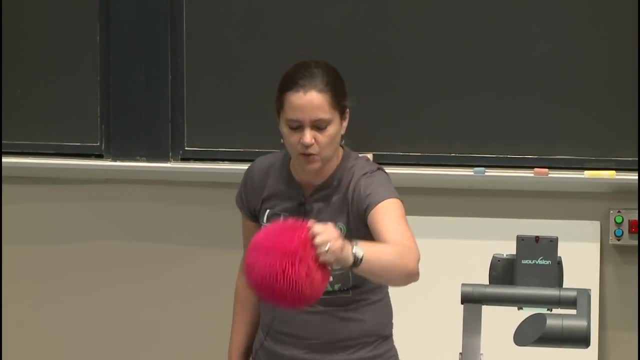 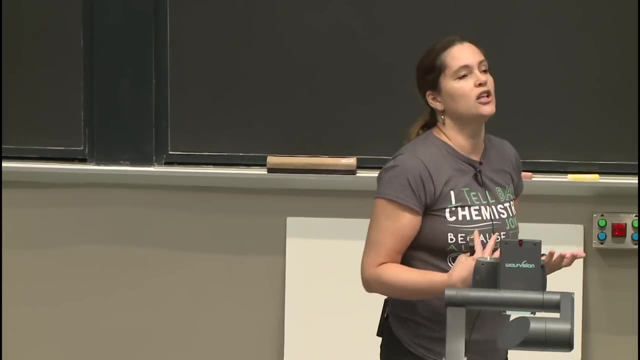 which I brought with me again because I just love carrying this through the infinite corridor and have people look at me. But if you do have ligands around, it'll happen if all of your d-orbitals are filled or if the energy levels are basically out of the visible range. 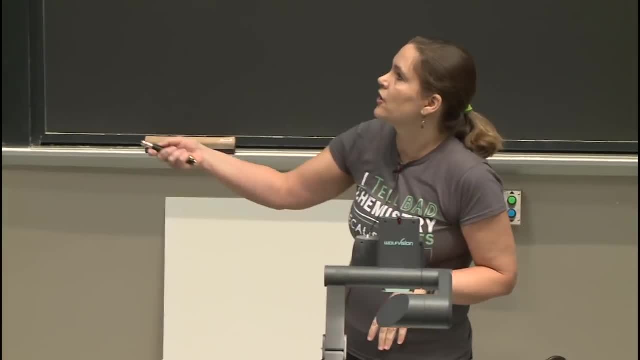 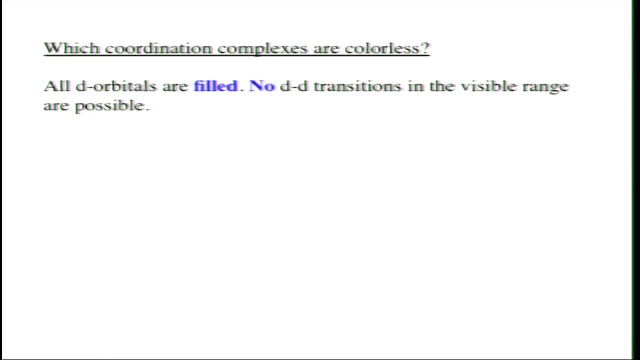 so the transitions are not in the visible range at all. So if they're all filled, so there's no way that you can move an electron, or if you can, but it's outside the visible region, All right. so now let's think about some examples. 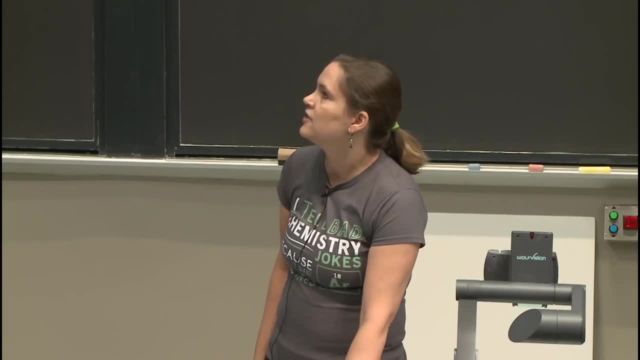 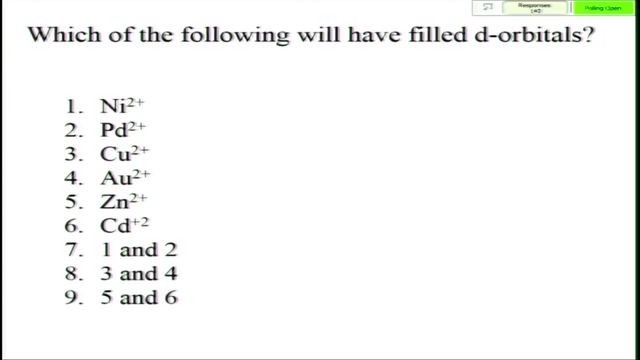 of what transition metals would fit into this, and I'll bring up my periodic table and we'll also bring up a clicker question. All right, let's just take 10 more seconds on this, All right, so we can take a look at this. 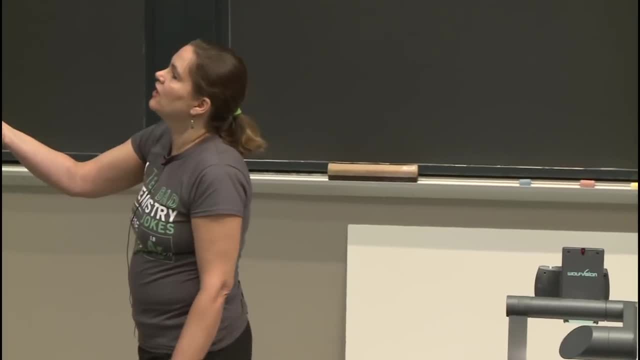 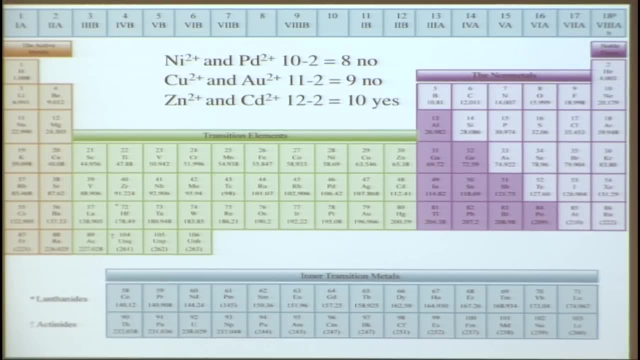 And with our periodic table, we have nickel and palladium Group: 10 minus 2 is 8.. Copper plus 2, gold plus 2, 11 minus 2 is 9.. Zinc plus 2, cadmium plus 2, 12 minus 2 is 10.. And so 10 would be the correct number for our filled d-orbitals. They can hold 10 electrons, So if we then go and fill this in, examples would include zinc plus 2, and cadmium plus 2 with our d-10 system. 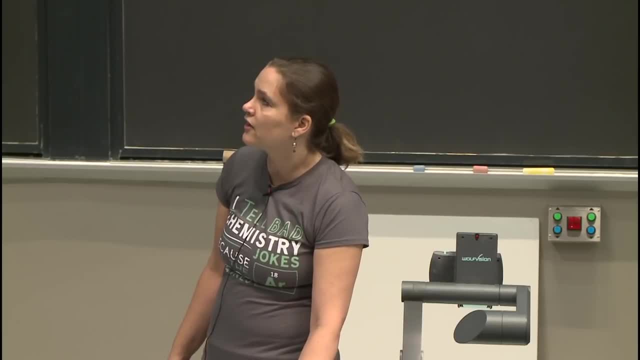 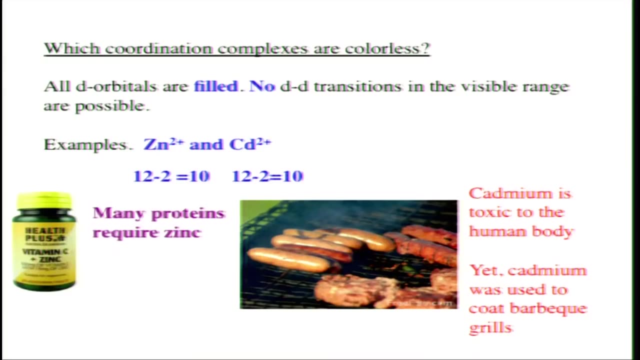 And in fact, zinc plus 2 is a very common oxidation state for zinc. Many proteins require zinc, Many of you have zinc in vitamin tablets, Some people take extra zinc to make sure you have enough zinc plus 2 in your body And a lot of times people who are studying proteins. 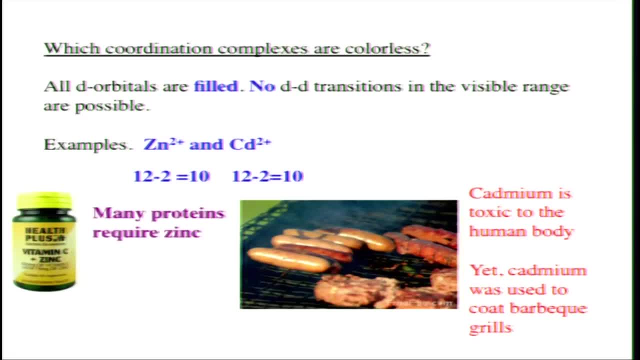 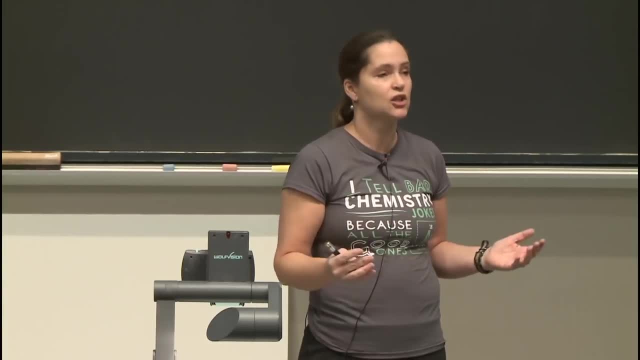 do not realize it's a zinc-containing protein because they isolate the protein and it's clear, So they don't think it has a transition metal in it. But zinc is hiding in that protein because it's colorless so you don't know it's there. 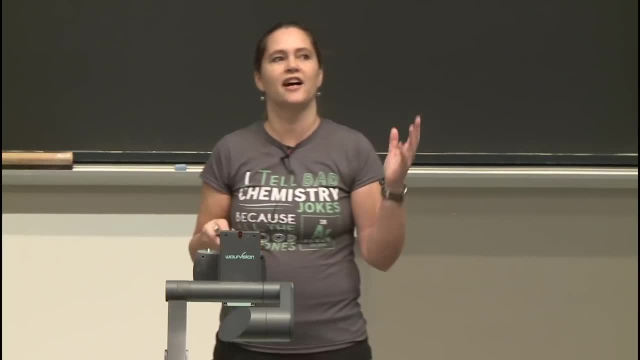 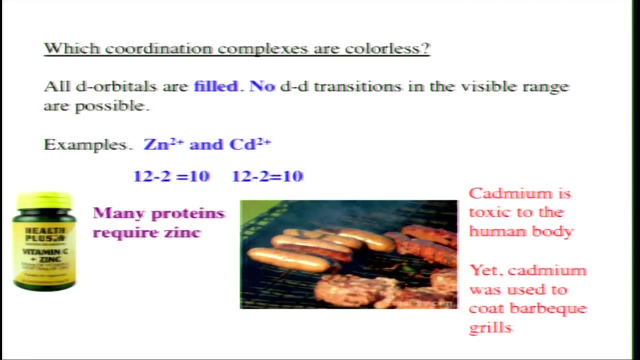 If you purify a protein with color, with other metals, it's really obvious that the metal is there. But zinc can be sneaky. Cadmium can also be sneaky. Cadmium, for the most part, is a poison to us. 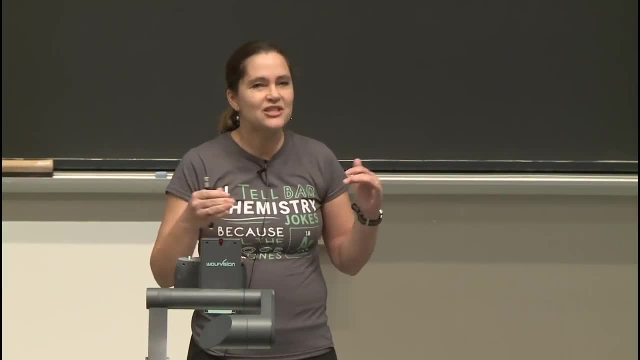 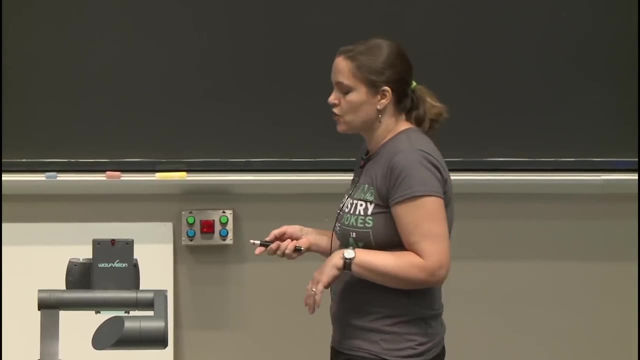 And they used to use it to coat barbecue grills, which is not. You don't want to put a poisonous substance on a barbecue grill and then heat it up. That's a really bad idea. So if you go to a barbecue and you think 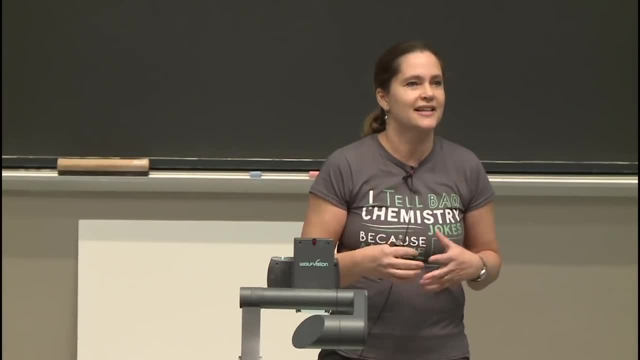 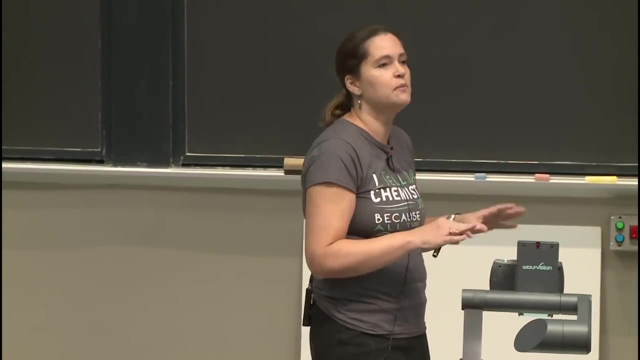 wow, that grill looks like. you know it's like 70 or 80 years old or something like that. it looks ancient. maybe you don't want to eat from that barbecue grill. They don't do this anymore, but old barbecue grills had cadmium on it. 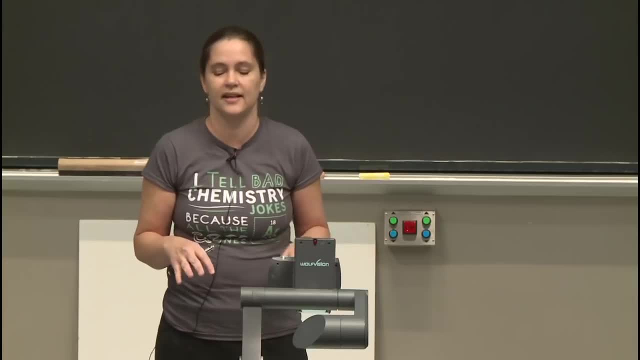 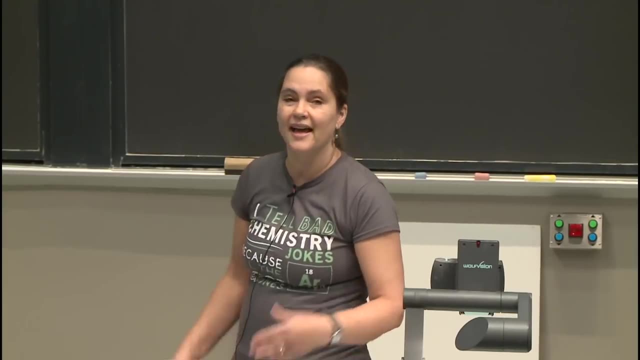 And I know someone who actually had cadmium poisoning and it was a really pretty terrible thing because it's hard to diagnose that, But they finally got the right diagnosis, All right. so again, colorless things. you don't know that they're there. 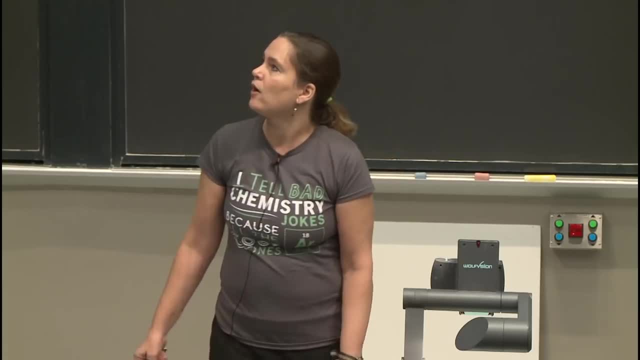 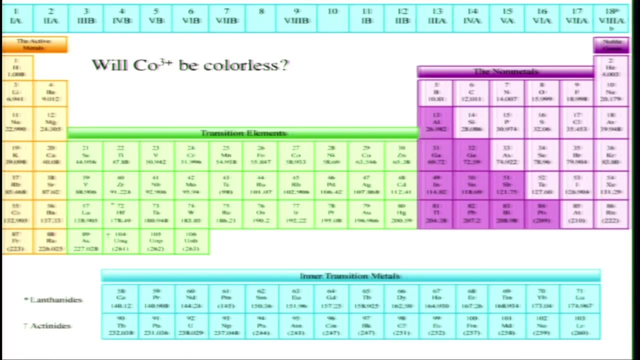 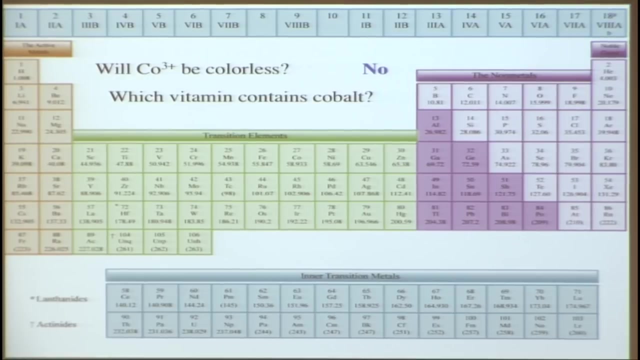 But they sometimes are All right. so what about cobalt plus three? You can just yell this out: Would this be a colorless compound? No, So we have in our group. nine minus three would be six, so it's not. 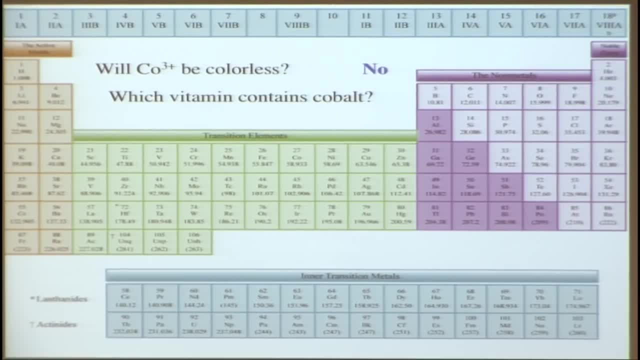 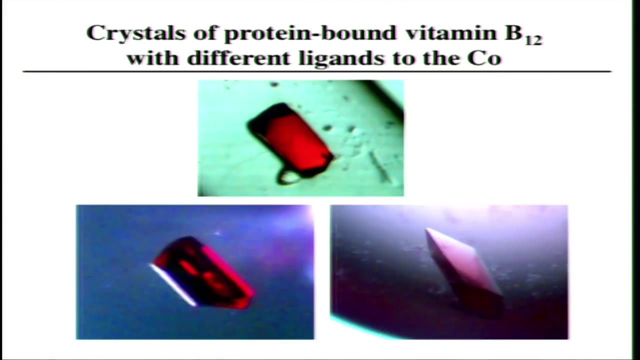 Which vitamin contains cobalt? And you probably all know, because we've been talking about it: vitamin B12. And I just thought I would share with you the colors of vitamin B12. And so this is crystals that contain vitamin B12, and these are their actual colors of the crystals. 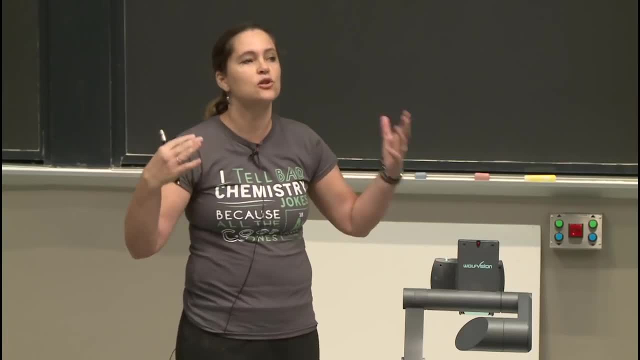 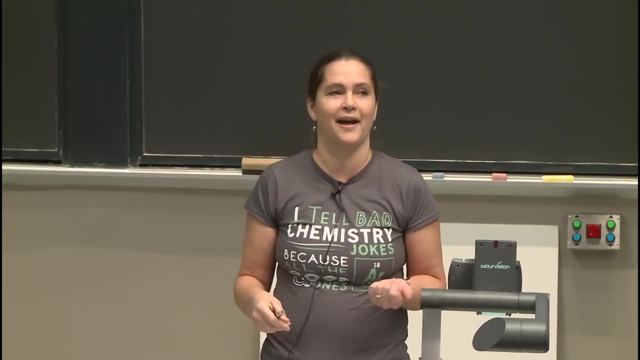 So it's really fun to work with vitamin B12. It's absolutely brilliant. except that it's also light sensitive, so you have to work in the dark under red light. So everything then is red because you're under red light. But if you bring them out and you expose them to light, 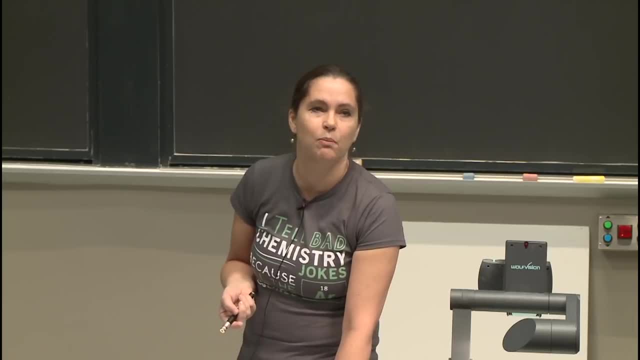 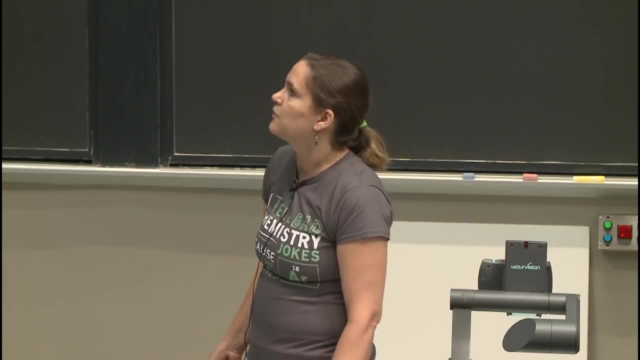 they're really, really pretty All right. so we're going to continue on this cobalt theme, because cobalt is one of the most spectacular transition metals when it comes to color, And I'm going to get you ready for a little demo. 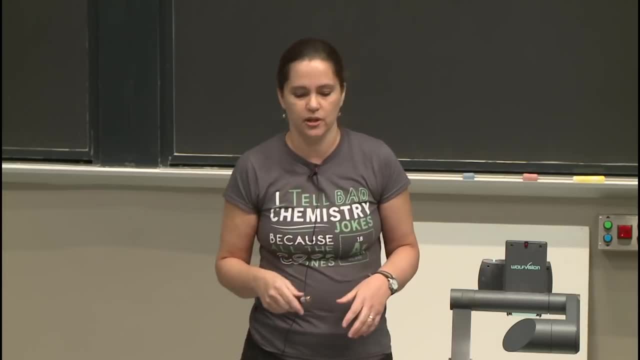 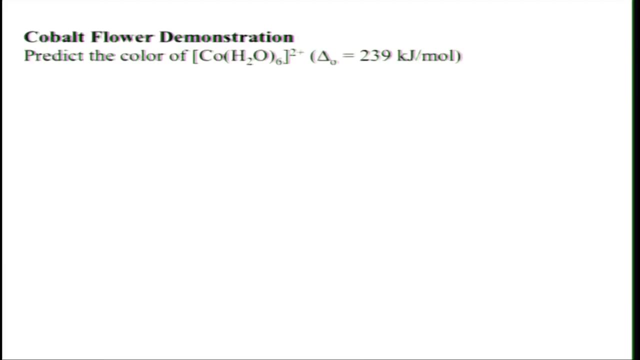 and you're going to help me first figure out what colors you should observe in this demo. All right, so we're going to have a cobalt compound that has six waters with it and you're given the octahedral crystal field splitting energy. 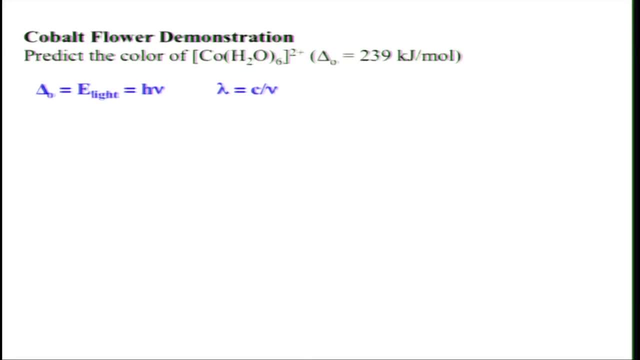 So now we want to predict the color. We want to predict the color. We're asking about what sort of wavelength is going to be absorbed, so we can think about the wavelength that will be transmitted. So we need to think about our equations. 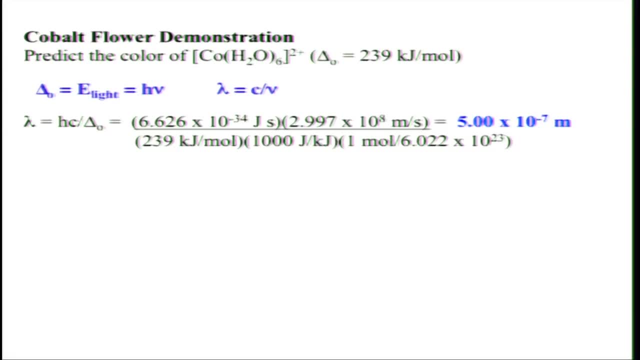 and we can combine these just like we did in many problems in the earlier part of the course. And so wavelength equals Planck's constant times the speed of light. Now, instead of just divided by any energy, we're dividing by the energy that's the octahedral crystal field, splitting energy. 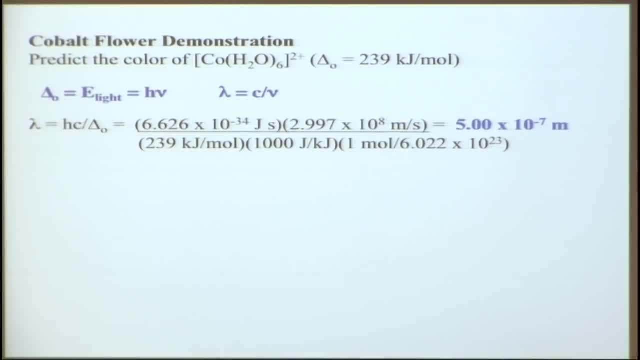 And so we can put in our Planck's constant and our speed of light and we can put in the octahedral crystal field splitting energy that we were given. but we want units in meters and so we need our joules to cancel out. 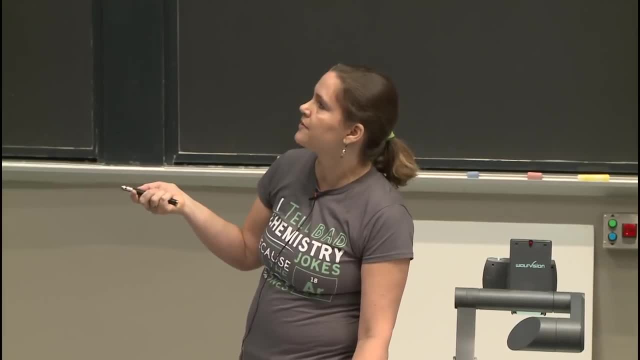 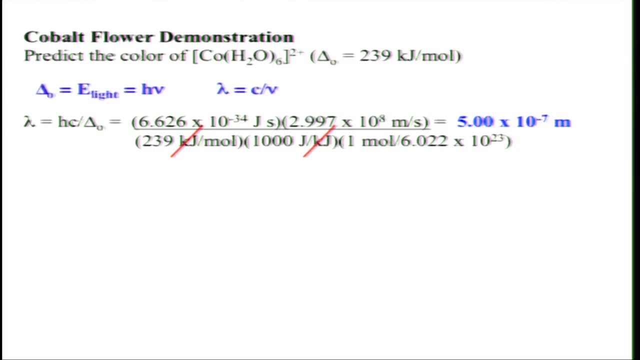 And in the bottom we're given the splitting energy in kilojoules. so we need to do some conversions. So first we need to get rid of this kilojoule, so we're going to convert it to joules, Then we can get rid of our joules. 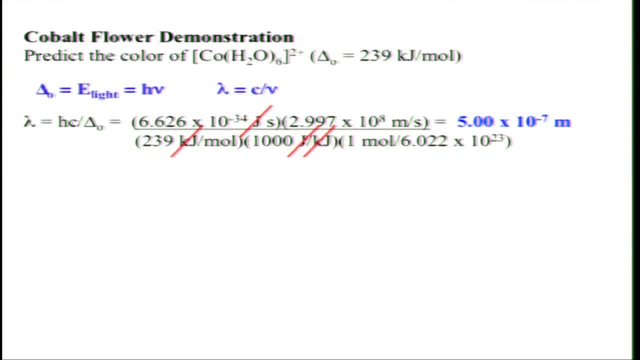 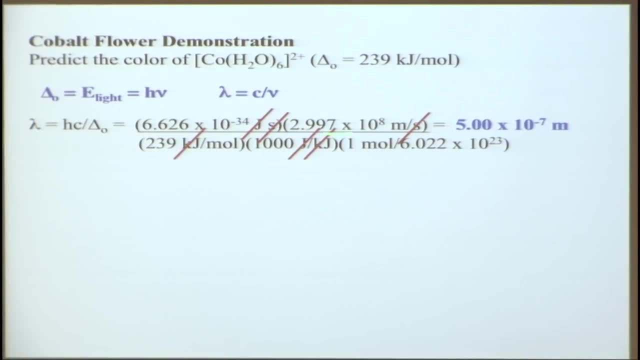 We also have seconds. We don't want seconds in our wavelength, but that is going to cancel out here and here. so we're good. But now our answer. we have meters at the top, but we have moles on the bottom. 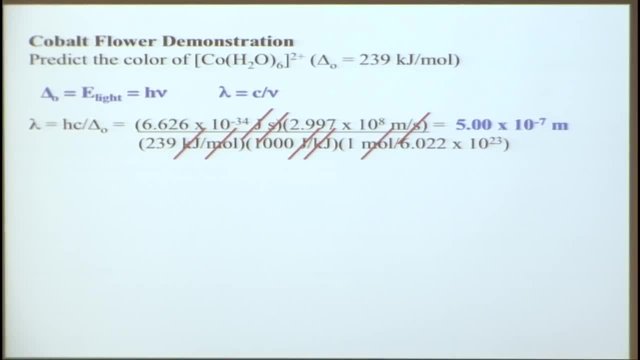 so we need to use Avogadro's number to cancel out our moles, And if you don't do that, you're going to get a really weird number for your wavelength. It's not going to make sense. It's going to be off by something like a factor. 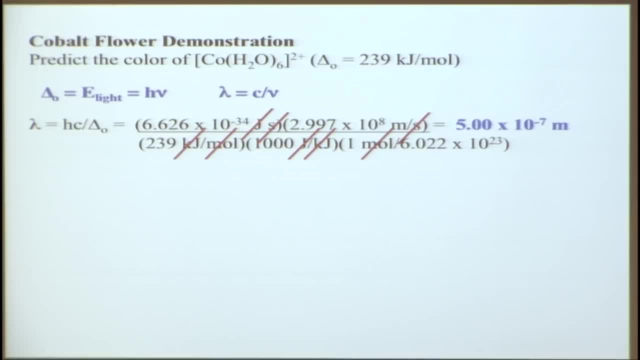 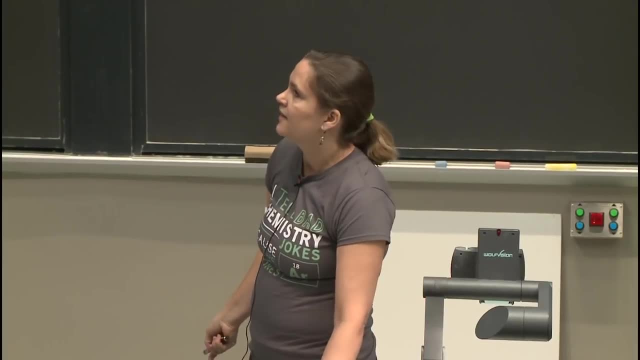 of 10 to the 23.. That should remind you. you want to use Avogadro's number here to get rid of your per mole. All right, so now we have a wavelength, And yes, on your equation sheet, we will give you this. 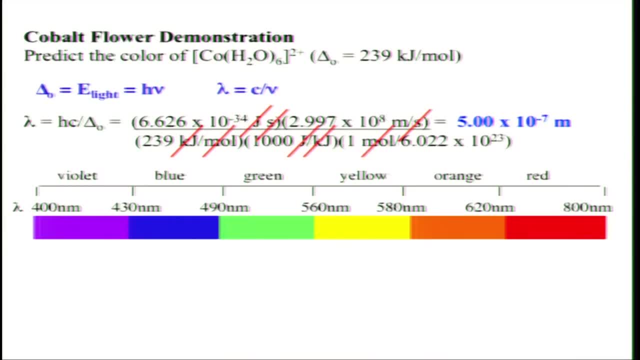 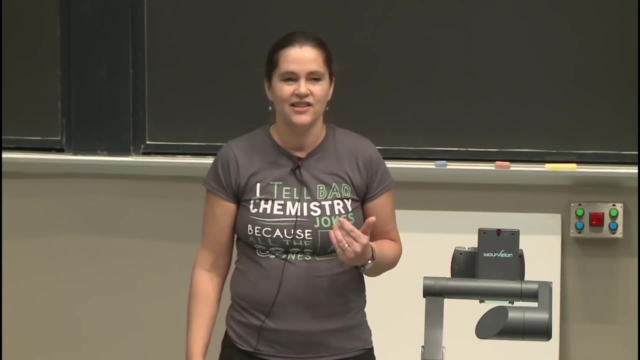 We will give you the color spectrums. You don't have to memorize this. So about 500 nanometers is in our green region over here. So the color that should be absorbed, given this octahedral crystal field splitting energy, is green. 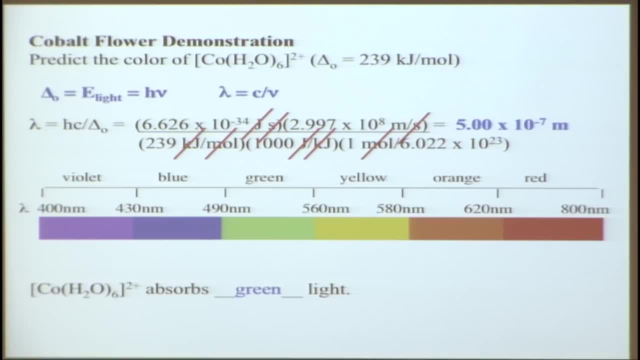 So now for green. what is the complementary color of green? Yep, so it's going to be reddish. We have our little drawing over here, So the predicted color would be red. So let me just now tell you about this demo. 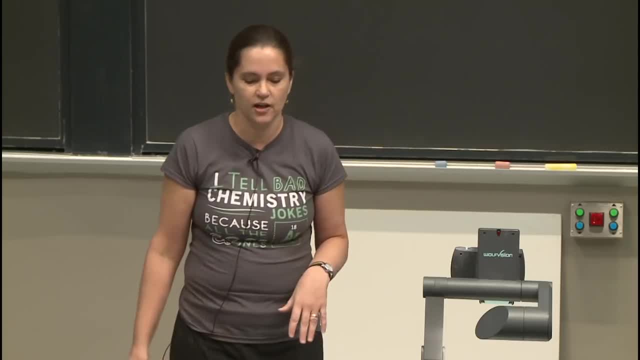 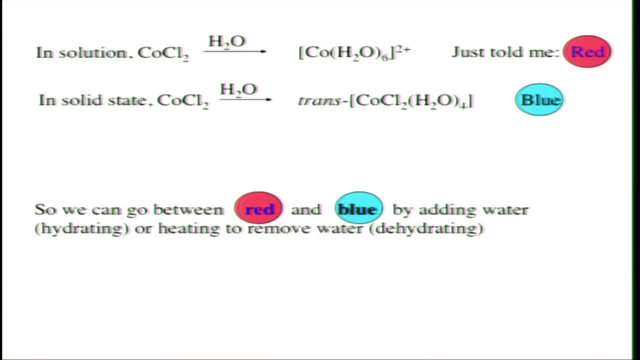 And we're actually going to see some red color, but we're also going to see another color, which is blue. So, in this demo, if you start with some copper chloride and add a lot of water, a lot, a lot of water, 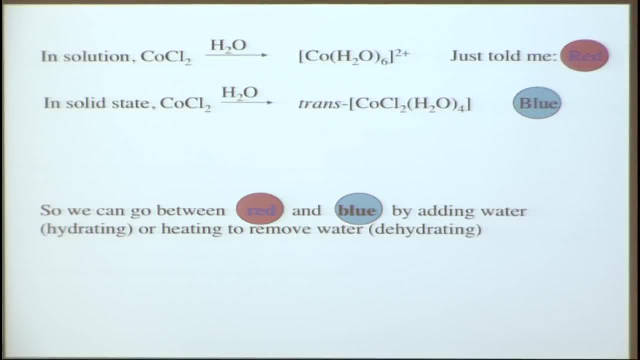 hydrate it really well, you'll get this octahedral system that you just told me was red, But if you don't add a lot of water, just a little bit of water, you'll only display some of the chlorides And then you're going to have a blue system. 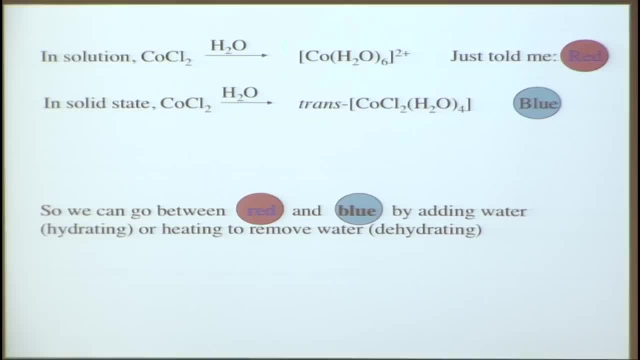 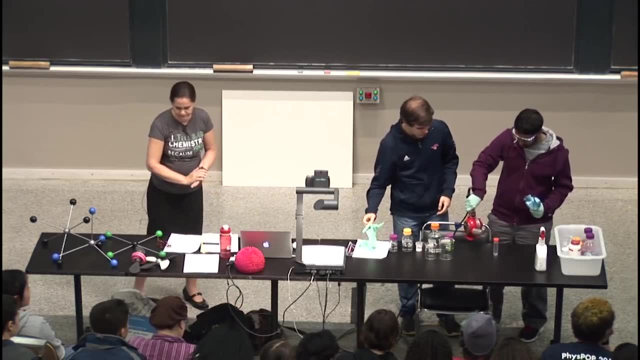 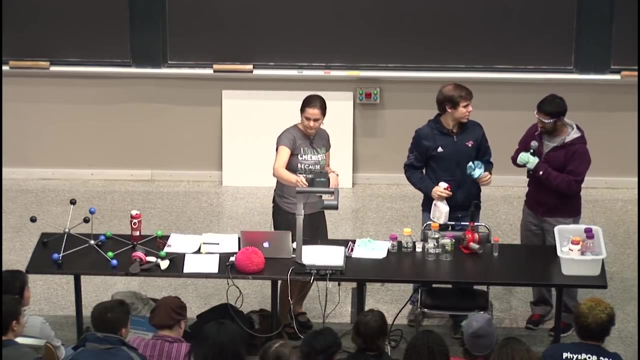 So if you have a lot of water, red and you're hydrated, red, if you're more dehydrated, you get blue. So we're going to now try this out and see if it works. Is it on? Yeah, it's on, great. 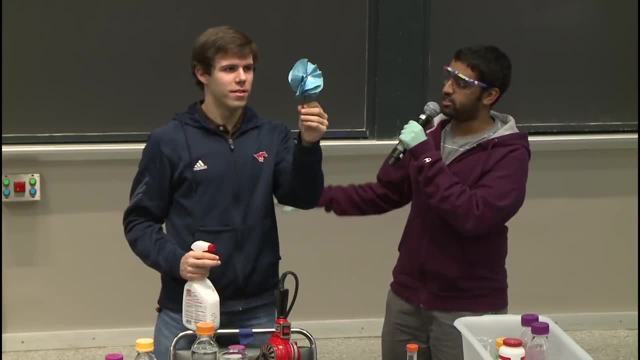 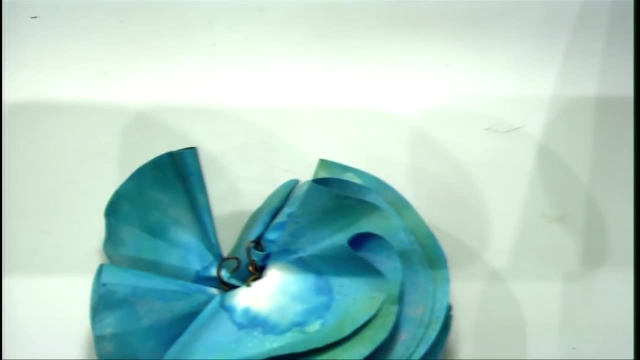 Okay, so that's the cobalt flower And, as Kathy said it's, Oh, we're going to put it under there. As Kathy said it's, It's got some cobalt and it's got water ligands and it's also got chlorine. 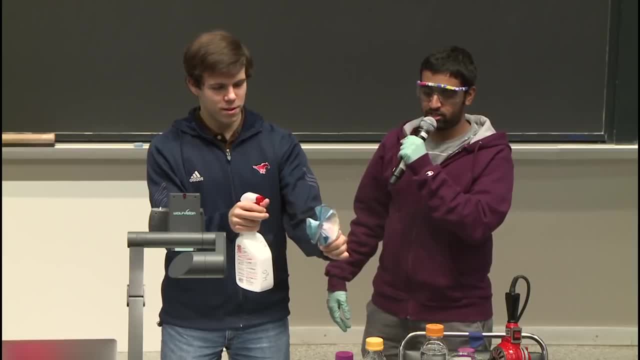 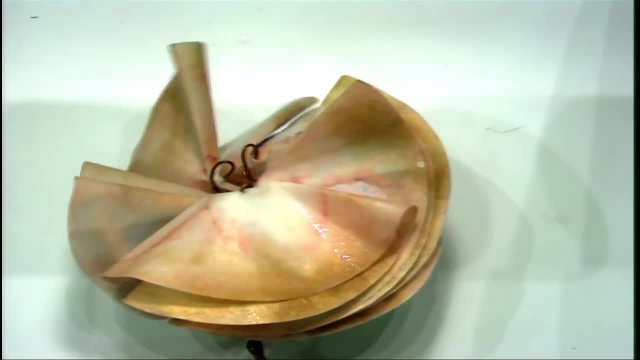 And Eric's going to sprinkle it with water now. So we're going to hydrate it. Hydrate it as you do when you have to water a flower, And it's turned, I guess, a pinkish-reddish color, right. 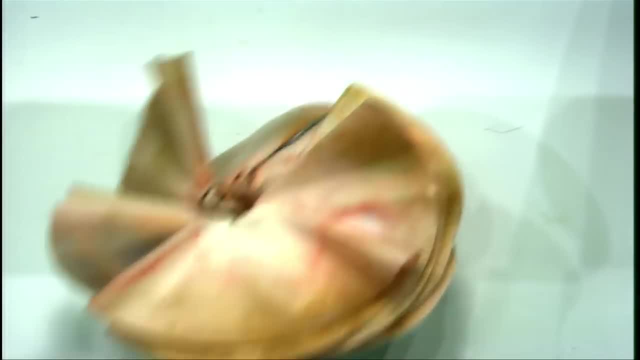 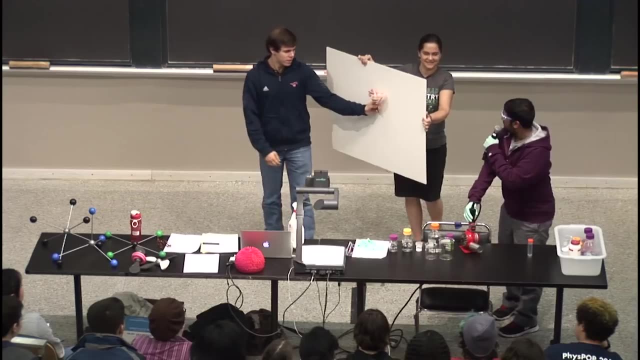 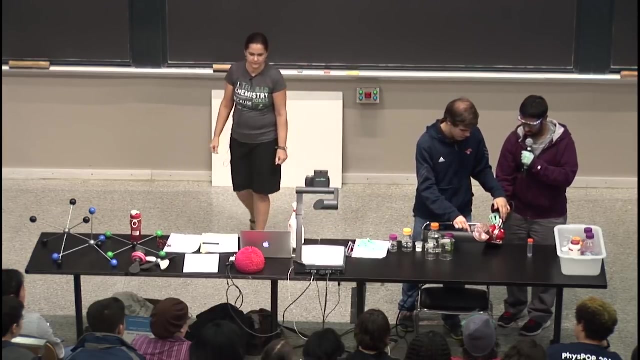 Can they see that up there? Yeah, It looks better with that. Hold it against this too, I think, Right. So to show you that it was. This is, in fact, the water that led to this color change. We're going to try to dry out the flower. 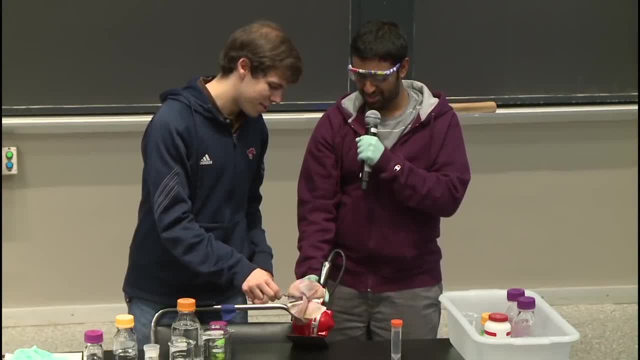 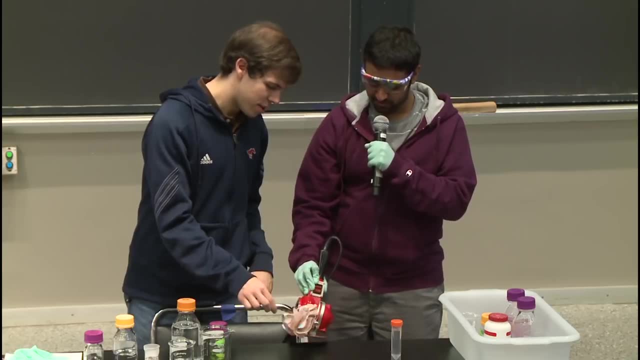 Is it working? Am I on hot? Yes, I am. I know it's really slow, I'd just rather it go faster. And Oh Yeah, Why don't you hold it under the document camera? I think you can kind of see it happening. 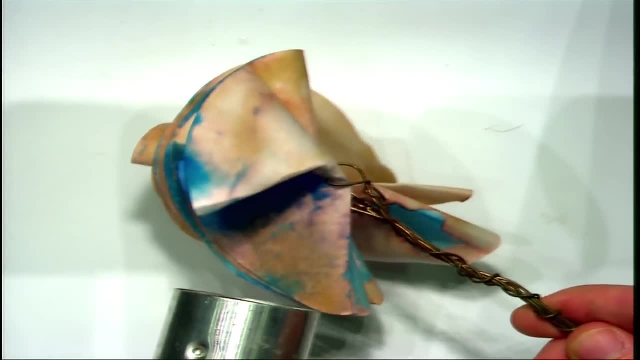 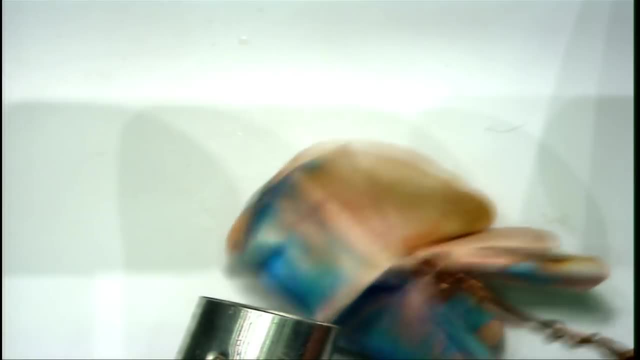 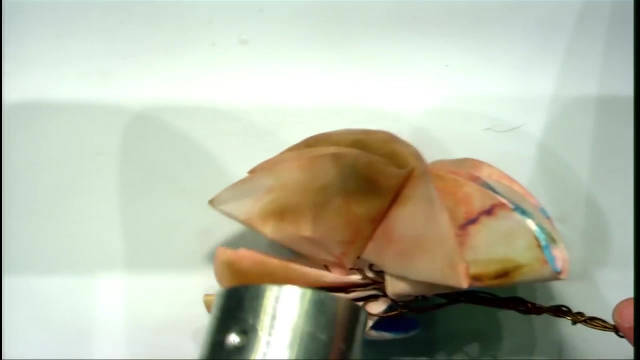 So as There we go, That's working. As Eric continues to warm this thing up, the water is evaporating and, as that happens, it starts forming that hydrous chloride complex instead of a pure hydrous complex, and it's.